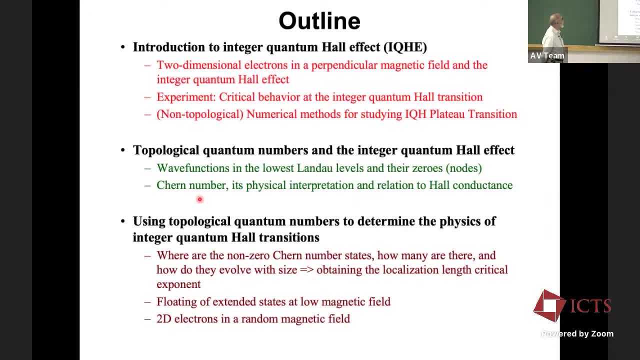 Introductory part. So I will basically talk about three things there, Just general two-dimensional electrons in a perpendicular magnetic field and the integer quantum hall effect, And then I'll talk about critical behavior at integer quantum hall transitions for non-interacting electrons, As the speaker this morning emphasized. 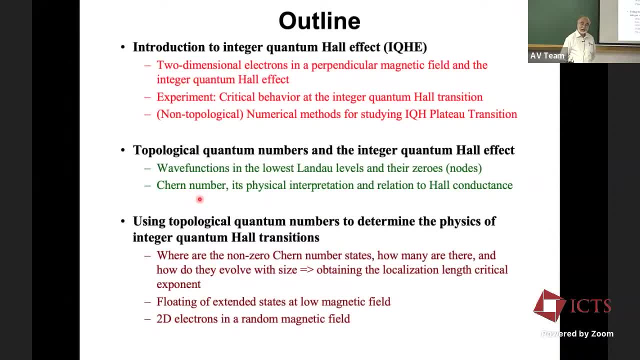 we don't really know whether the non-interacting electron model is appropriate for real electrons at these integer quantum hall transition. That is a question that still needs to be addressed. But this will concentrate only on non-interacting electrons, And then I will talk about numerical methods for studying these plateau transitions between. 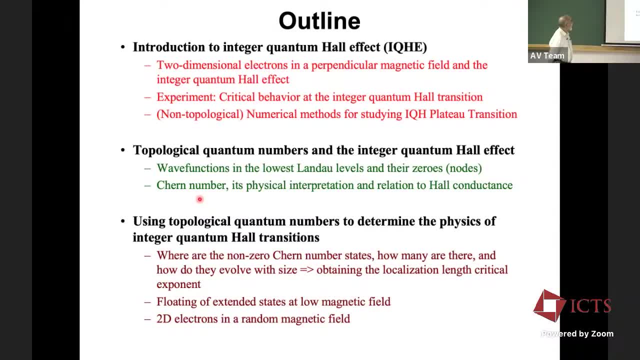 different integer quantum hall states And I call them non-topological methods because they're not topological. This is just conventional methods using strip geometry, which I talked about under Anderson localization, But I will give some more examples of how this is done in the quantum hall regime. 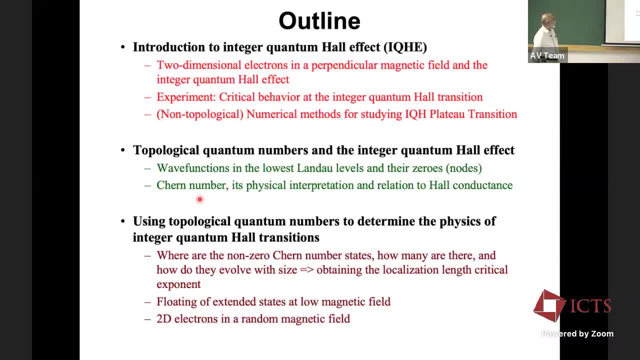 And then I will concentrate quite a bit on understanding topological quantum numbers associated with eigenstates in the quantum hall regime. These are known as Chern numbers, And so I will go through this description of what happens to wave functions when you have electrons in the lowest landau level. 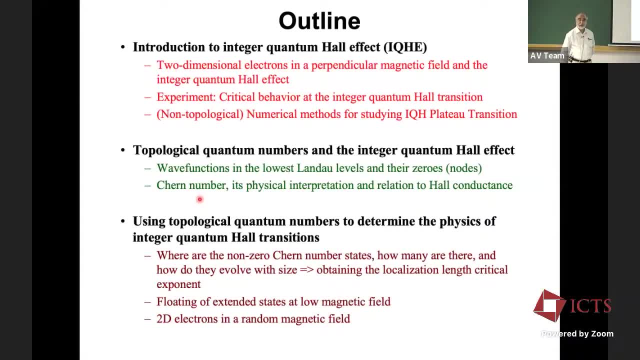 because as soon as you put on a big magnetic field and if it's large enough, all the electrons going to the lowest landau level where the kinetic energy is quenched, and the only energy in the problem, if you're not having the electrons interact, is the disorder potential that is there. 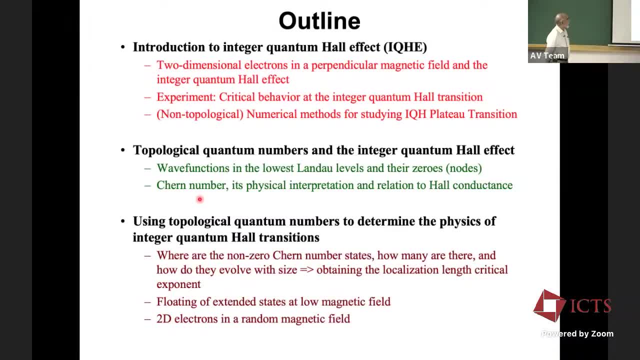 invariably present in any experimental system, And I'll introduce the Chern number, talk about its physical interpretation and its relation to the whole conductance of contribution due to that eigenstate, And then I'll describe a method which is very different from the conventional methods. 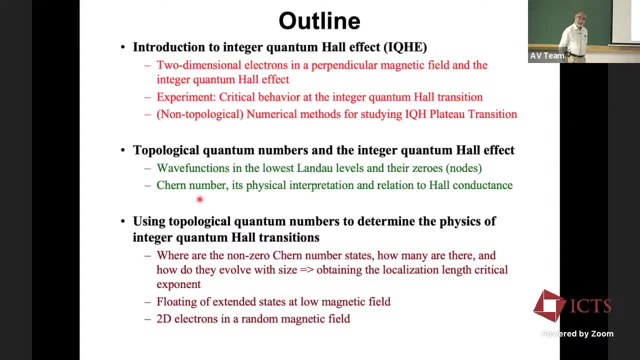 to determine the localization length exponent near an integer quantum Hall-Plateau transition, And this involves looking at non-zero Chern number states, eigenstates. We're talking about one electron physics, so there's an eigenstate for each electron And we look at the properties of those eigenstates. 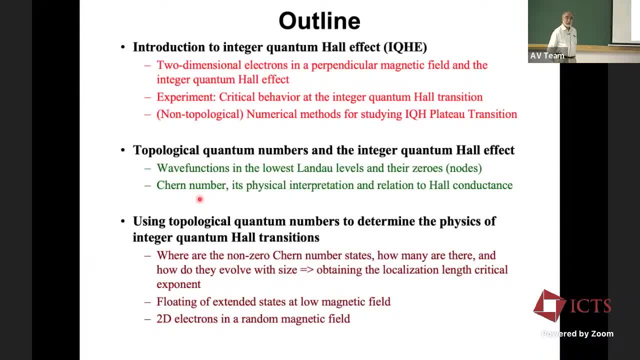 and from those properties and simply their topological character, we are able to actually get the exponent of the localization length. And then we can also look at the quantum Hall-Plateau transitions, And then I'll also show that, the same kind of method. 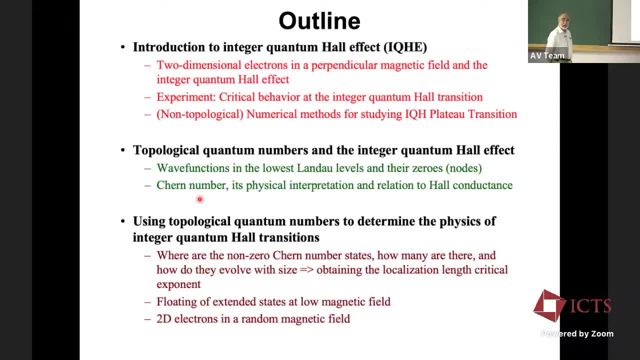 can be used to answer other questions, In particular a question as to what happens when you go to low magnetic fields, because we know that in zero magnetic field, with pure potential scattering in two dimensions, all eigenstates for non-interacting electrons are localized. 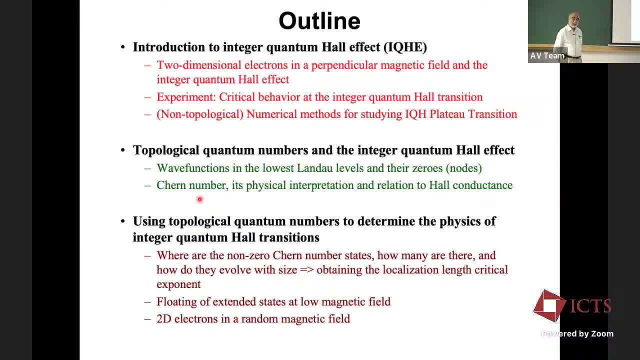 So you don't have any extended states In that system, And how does the quantum Hall picture merge into that? And then, finally, I also do apply it to 2D electrons in a random magnetic field, which is a bit of a- you know more of a- theorists problem. 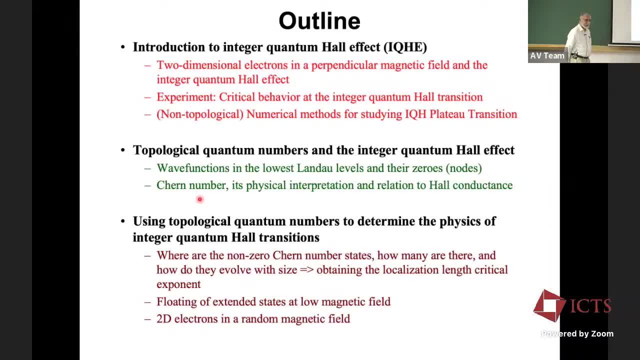 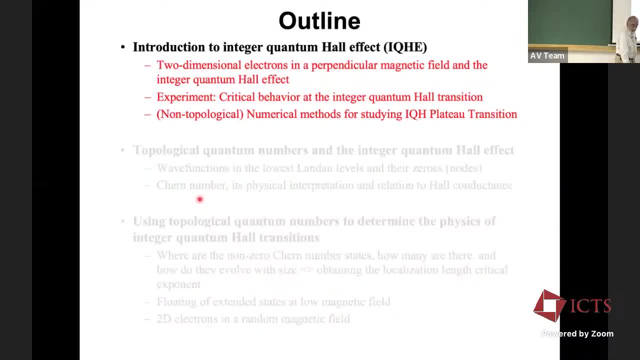 It's not something that the experimentalists can do, but it's also worthwhile looking at that case. So that is the basic plan for today's lecture. So we'll start with the first one, which is basically introduction to the integer quantum Hall effect. 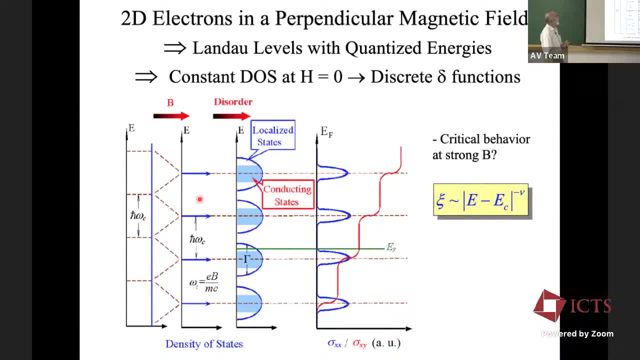 So when you have two dimensional electrons in a perpendicular magnetic field, the constant density of states that you have, which is shown here, here's energy, there's the density of states and it's constant At zero magnetic field As soon as you put on a magnetic field. 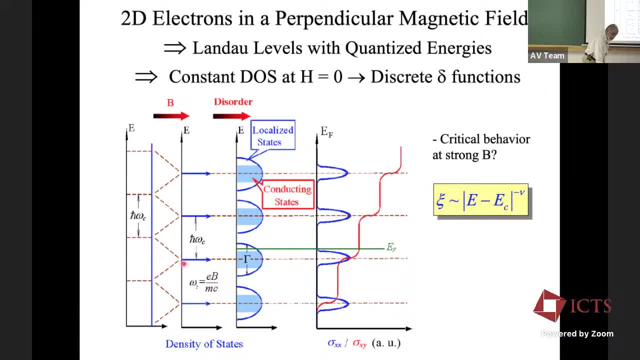 this constant density of states splits into Landau levels, which are fixed energies that are separated by an energy H bar. omega C and omega C is proportional to the magnetic field. Omega C is EB over MC. I will be using both the word symbol B. 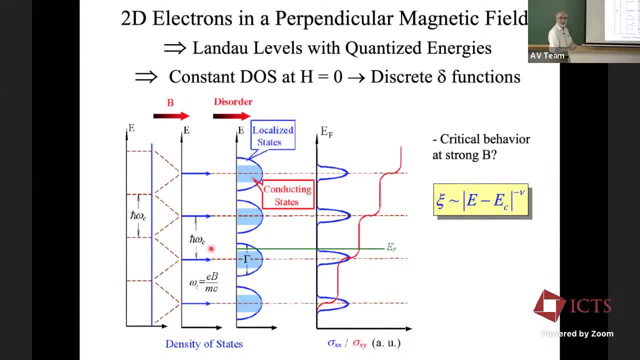 and the symbol H for magnetic field, And there's no difference between what those two things if you're talking about, you know, magnetic field. There's no non-magnetic materials with no, no difference between B there. There's no induced magnetization, if you will. 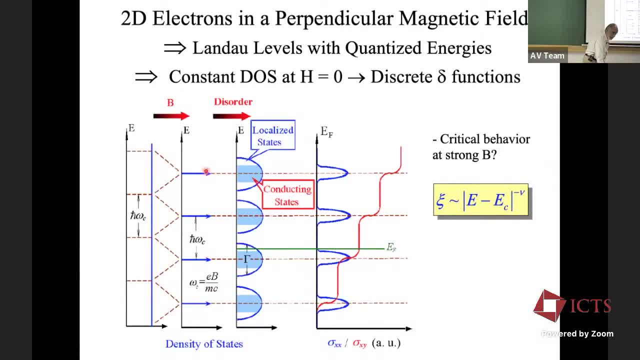 Now these are in a clean system. you get these Landau levels which are separated by H bar omega C, and you can make H bar omega C as large as you want by increasing the magnetic field. It also turns out that the number of states 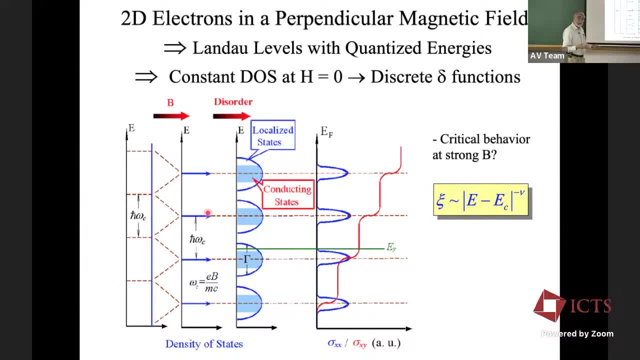 in each Landau level is not only proportional to area, it's also proportional to the magnetic field. So you can get more and more electrons in the Landau levels as you increase the magnetic field. So as you increase the magnetic field you can actually in a experimental system 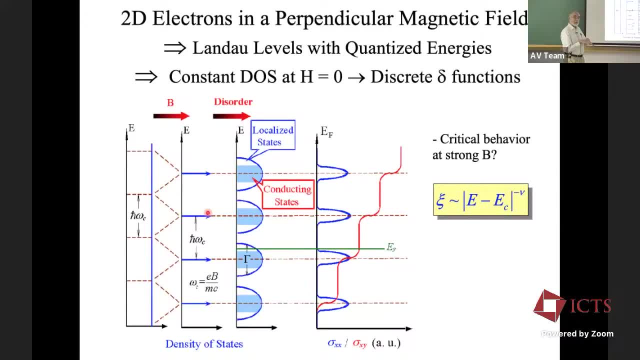 with a constant number of electrons. the electrons first have a continuum of energies, then they occupy a lot of Landau levels, then the number of Landau levels shrinks as the magnetic field goes up And finally you can at high enough fields. 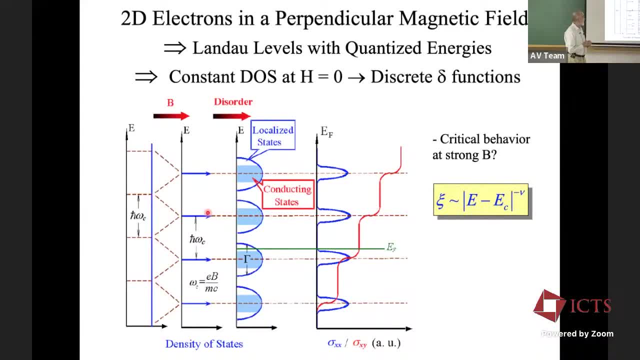 all the electrons could be in the lowest Landau level, And what we will show is that that, in fact, if you, if there is disorder present- and we will represent most disorder by a white noise- potential of a certain width- width is taken to be much smaller than the Landau. 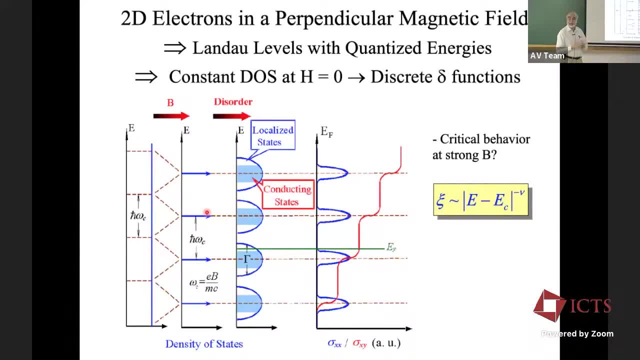 the cyclotron energy, H bar omega C. So we don't mix Landau level, we just stay within one Landau level And, in particular, what's gonna happen is we are gonna study only the lowest Landau level, this one. 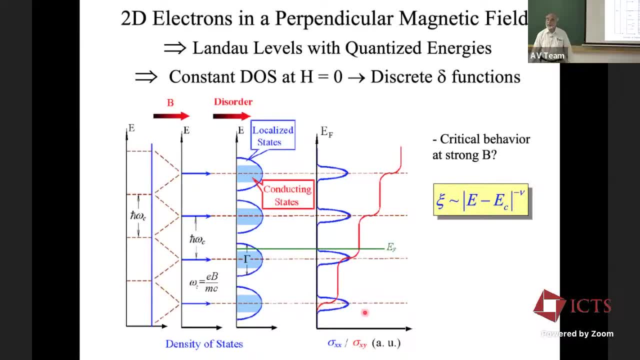 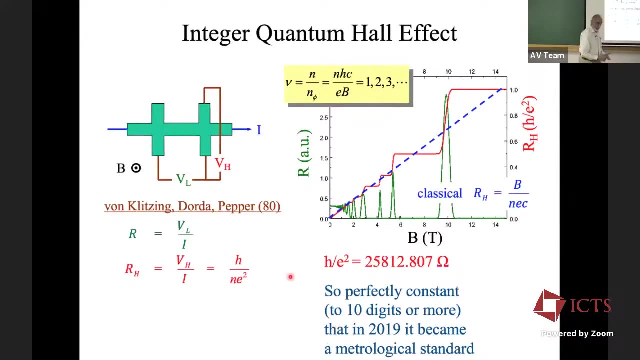 Assume that the field is so large that all the electrons are in that Landau level, which has been disorder broadened in some way Now, as one sees in experiment when you take such a sample. and so here is the same plot that was shown this morning. 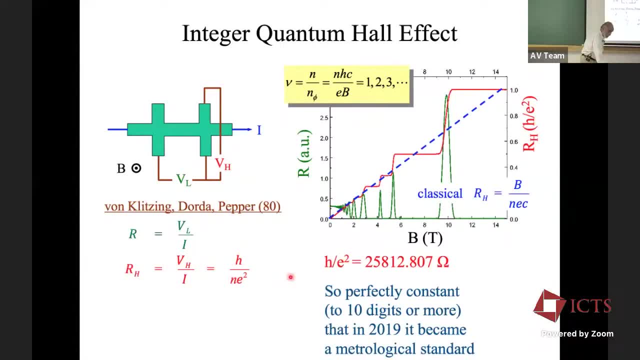 in this morning's lecture is: you take a typical Hall-Barr sample. you pass current in one direction, put a and you can measure the potential transfers. you can measure the potential longitudinally and the magnetic field is out of the plane. 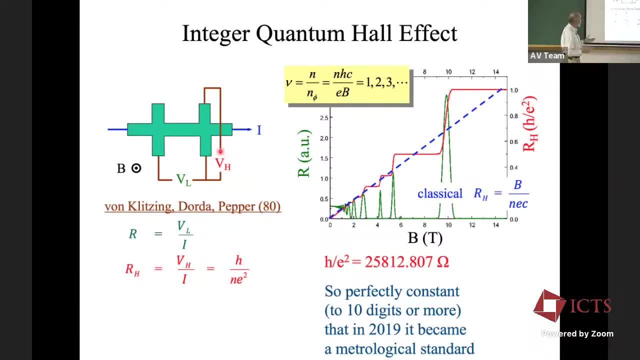 So it's in the third direction. And when you do that, if you look at the Hall resistance, which is just defined as Hall voltage divided by current, and you look at the longitudinal resistance, which is the longitudinal voltage divided by the current, 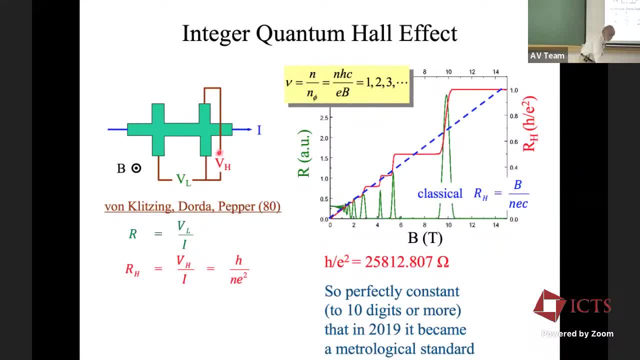 you get these green and red curves that are shown here. The red one shows these big plateaus that those are the quantized integer Hall effect, which is H over N, E squared. The values are, and these values are incredibly accurate With reasonably good samples. 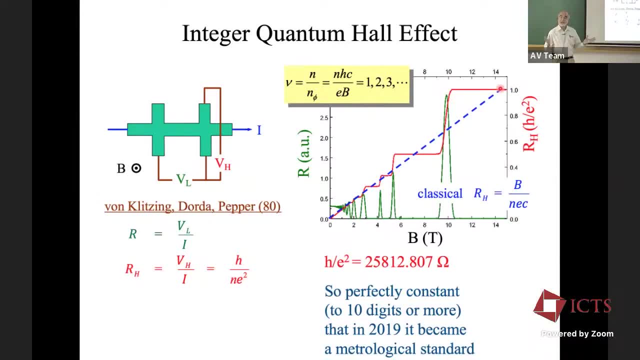 you can get this to be correct to 10 digits or so At low temperatures. And so, in fact, this particular number, the conductance or unit of resistance H over E squared, which is some 25,800 ohms, is so perfectly constant that, three years ago, 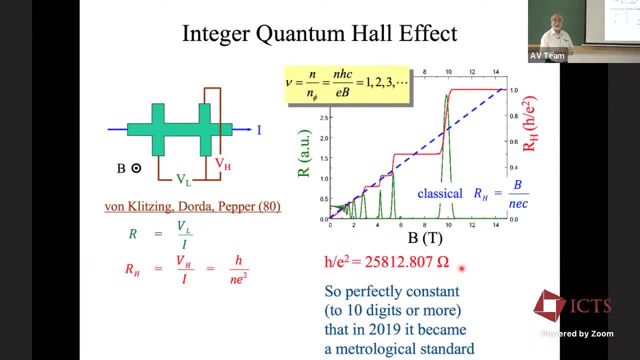 it became a metrological standard. We don't need the meter in France or the kilogram in France anymore. Everything is defined in terms of the quantum Hall effect plus some atomic measurements, And so we have length, weight, everything defined in these terms. 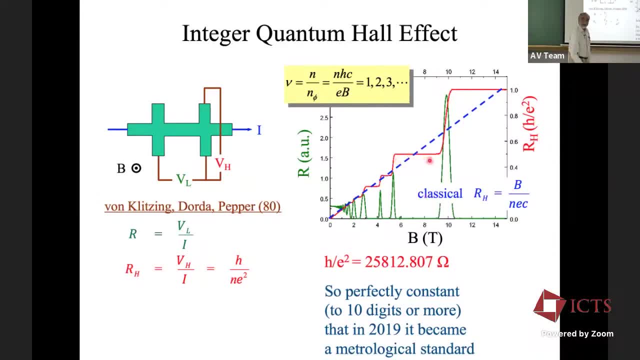 So this is how constant this one is. It is, that's what I want to emphasize. Now these plateaus happen at H over N, E, squared for the Hall resistance, And between plateaus, the resistance, the Hall resistance changes And technically the belief is that at zero temperature. 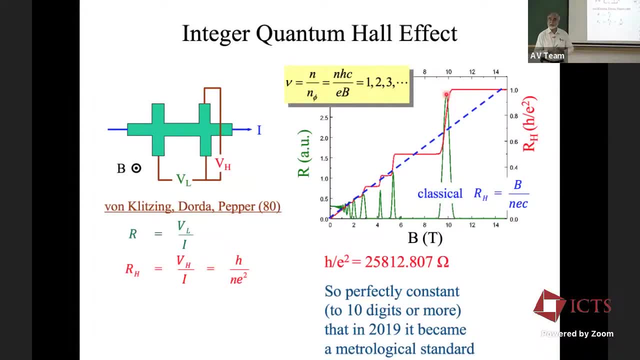 it actually just there's a precipitous step at one energy or one magnetic field, But at finite temperature. you find that this step is actually broadened by a certain amount And that broadening actually measures the nature of the electronic states that are there in this system. 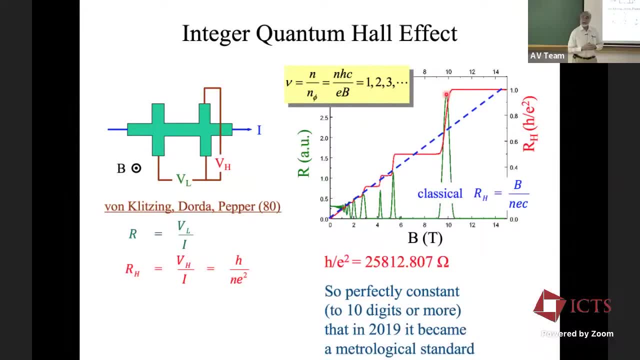 Another point that is very important, very important to realize, is that disorder is really important in this, in this thing. If you'd have no disorder whatsoever, it should imagine a pristine two-dimensional electron gas- you will find that you should get a Hall resistance. 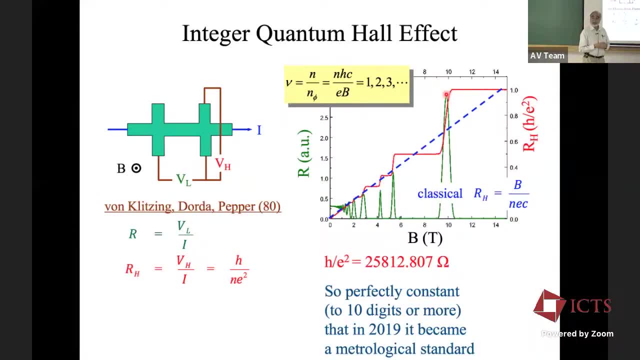 which is just linear in the magnetic field, And so getting those steps, one needs to have disorder, And these samples are actually reasonably disordered by today's standard, And something like several tens of thousand in centimeters squared per volt second mobility, Whereas now we have millions. 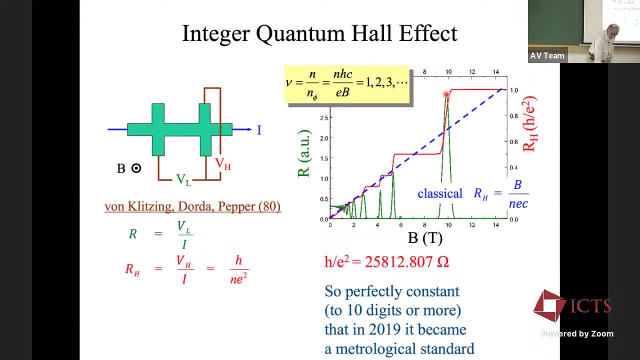 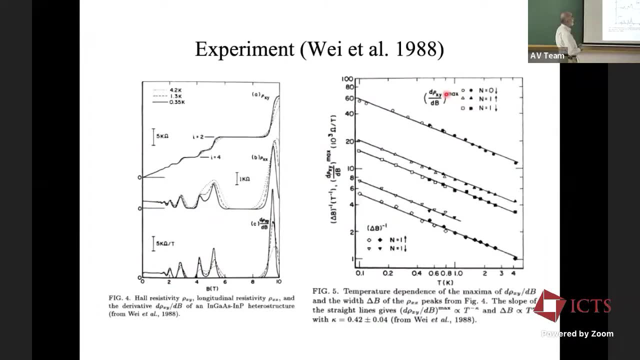 40 million available with very pure samples. So what actually you see is: here are two data points showing how the longitudinal resistivity at the step. So if you notice the longitudinal resistivity at the step, that's the longitudinal resistivity at the step. 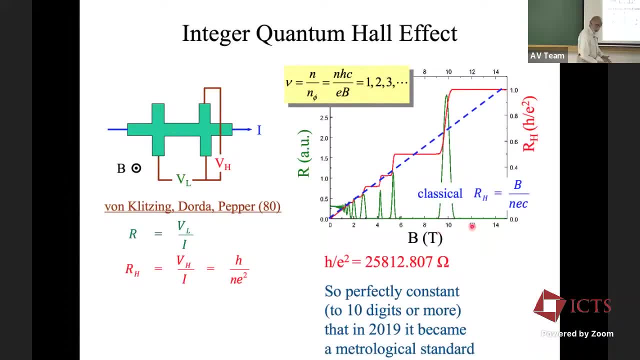 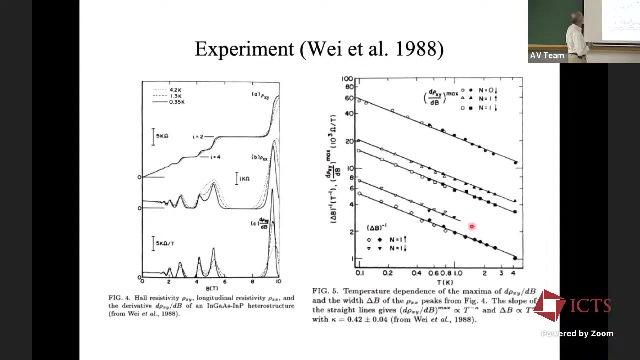 That's the green curve. here is really a peak. It's longitudinal resistivity zero elsewhere, And then it's it peaks up at that And you can look at how the peak changes with temperature And that's what you see. here is what you find the data. 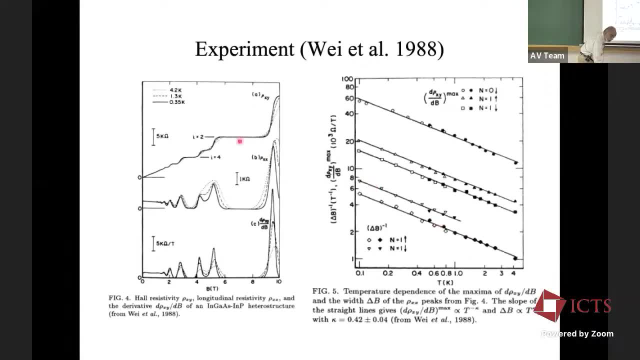 from three different temperatures on the left side: 4.2 Kelvin, 1.3 Kelvin- 0.35 Kelvin is some early data- And 988, and you see that the peak sharpen up as you lower the temperature And they're consistent with the peak going to zero width. 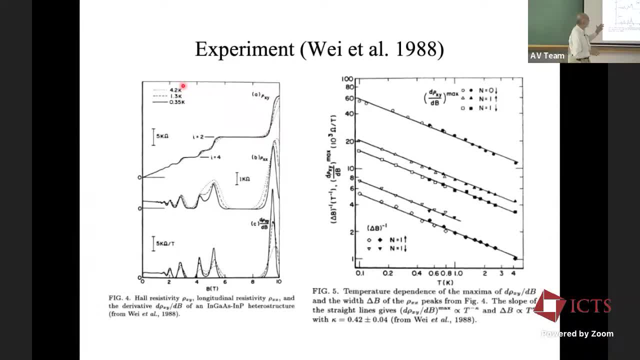 in the zero temperature limit. You can actually plot this peak weight as a function of temperature. In fact, this is the opposite. This is the slope that is being plotted at the midpoint, plotted as a function of temperature on a log-log plot. 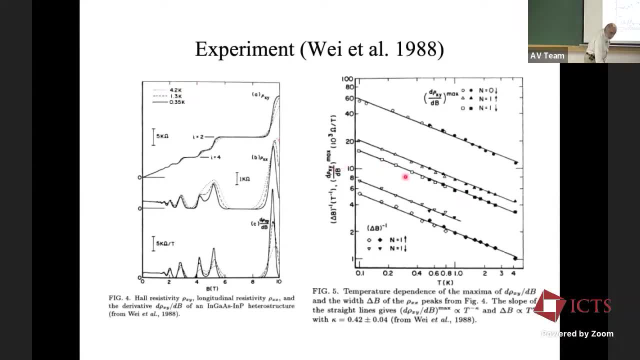 And what you find is that these log-log plots are fitted by a functional form T to the minus Kappa, And similarly, the width of the peak is also is fitted with the form of Delta. B goes as T to the plus Kappa, And the Kappa that is obtained from these experiments is 0.42,. 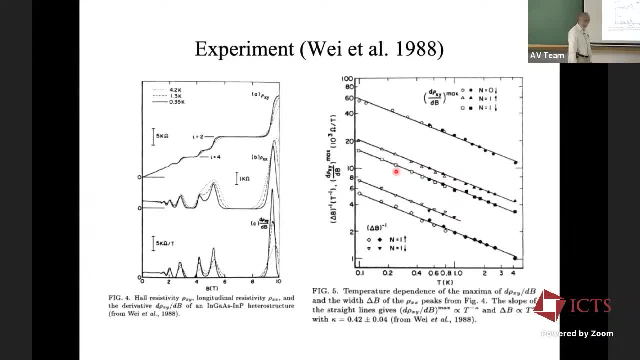 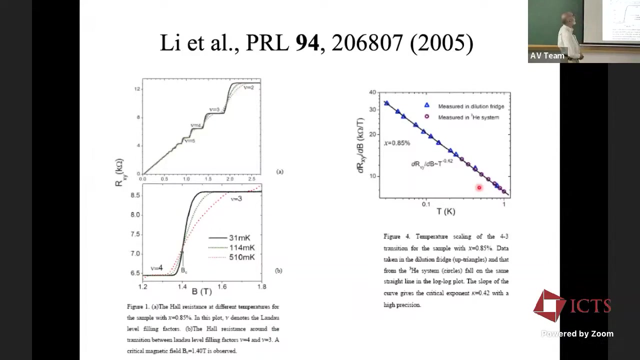 with an error, An error bar of about 10%. So these are again early measurements. So we'll see how this Kappa is related to the nature of eigenstates in this system. Here is somewhat more recent data from 2005.. 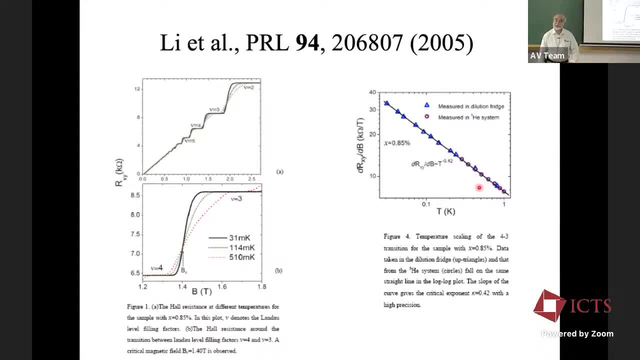 It's again from the same group. All both of these are from Dan Sui's group And at Princeton. And again you see that how the plateau transition here, in this case the plateau transition is from from the third Landau level to the fourth Landau level. 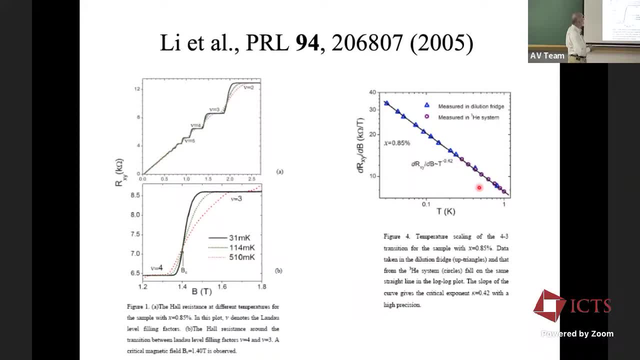 And you find that the step from one to the other is become sharper as you lower the temperature. And again the same story. you go ahead and do that And you find that this slope, as a function of temperature, is a power law, with a power law exponent of 0.42. 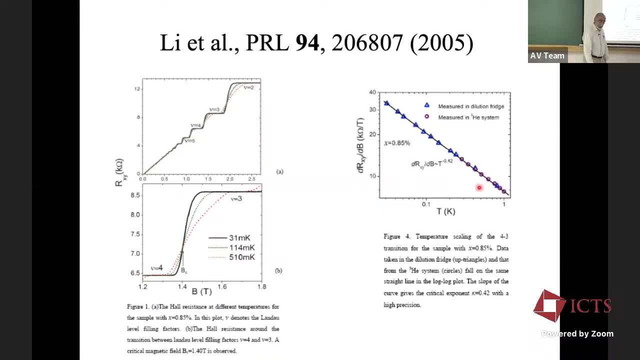 as in the previous data. I should point out that this only holds for certain kinds of samples. There are other samples which don't quite fit this picture and that issue is still not quite resolved as to why that is happening. But the reason why this was done was because Dan Sui felt that one should try and do short-range. 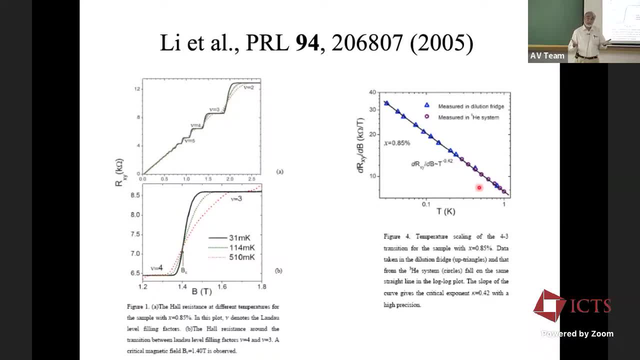 disorder, not have a, because if you're going to do disorder because of remote impurities which are giving a potential, then that that's a long-range kind of variation of the potential and maybe that long-range nature might be might mess up the experimental data. So in 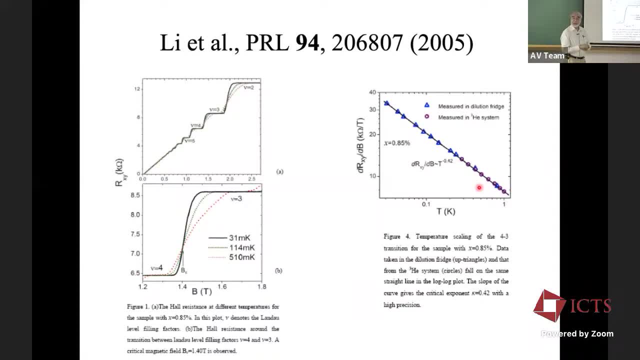 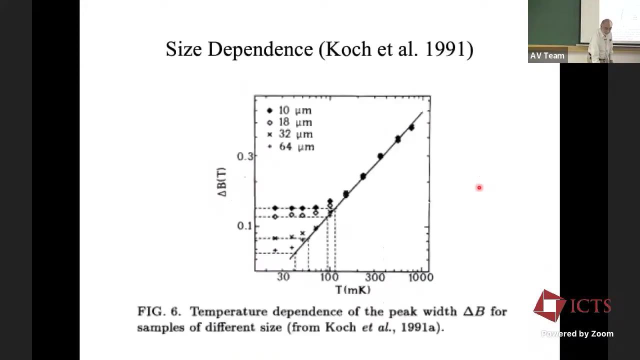 this case, he actually used alloy disorder in the sample to try and get very short-range potential, and this- x equals 0.85%- is basically the alloy concentration in the gallium arsenide system. Another thing that you can do is you can actually look at the temperature dependence of the 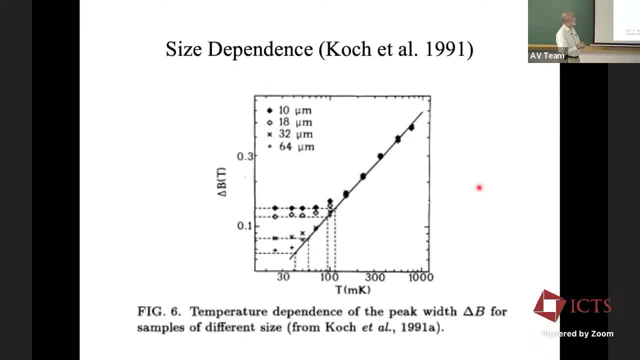 peak width for different sizes, And this is from a German group of Focke et al, and again you see the peak width as a function of temperature on a log. log plot seems to go up as a power law. But one other thing that you notice is that, depending 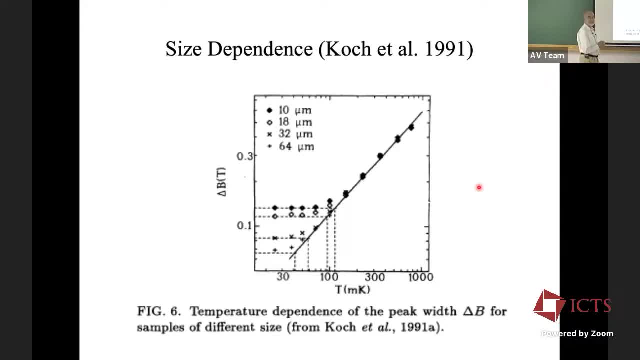 on this size of the sample. these are small samples, from 10 microns to 64 microns. You see that the 64 micron sample gives the data down to lower temperatures and whereas the- you know- 10 micron sample saturates at something like 100 or 120 milli kelvin. It's coming down and then it 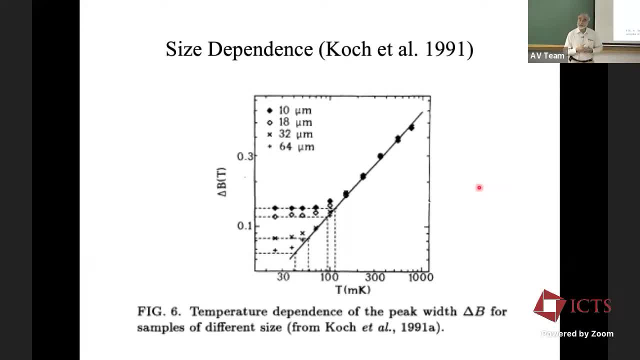 saturates, And the understanding is that when it saturates you're not really looking at the localization length of the electronic wave function because it has reached the size of your sample And so you can actually look at directly from the saturation. you can also 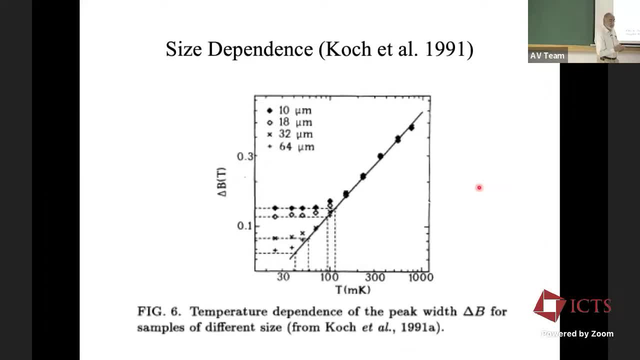 determine what is happening. There's a third way of doing it, which is you can put on an electric field and see saturation because of finite electric field effects, and that is yet another way. So there are actually- it turns out that there are the. 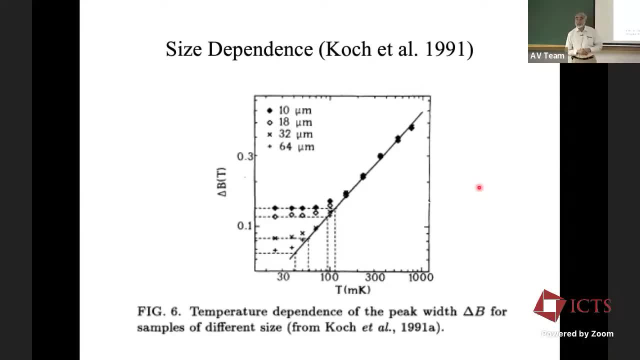 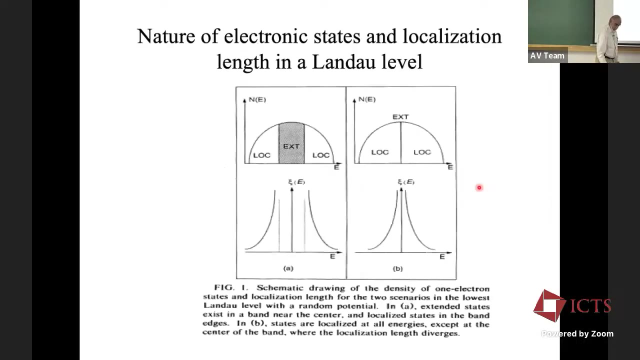 natural quantity that the experiment measures is a combination of the localization length exponent and the dynamical exponent z. it's the product, But you can extract the two by doing these various different experiments. and that's how experiments get the localization length exponent is by combining several experiments and separately extracting z, nu and then z. 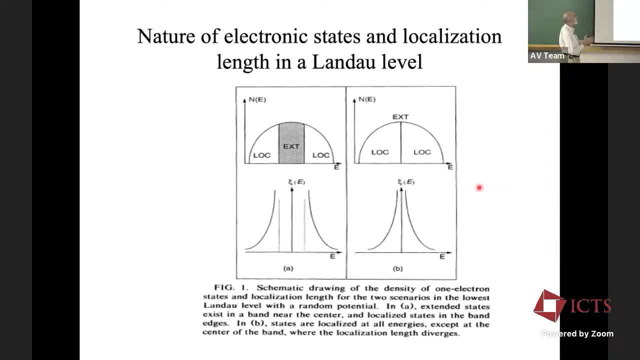 as a result of that. So schematically, this is the picture that one has in for non-interacting electrons- is that the density of states is some. I mean, I've drawn a semicircle, but they're just stylized. I think There's no reason for the density of 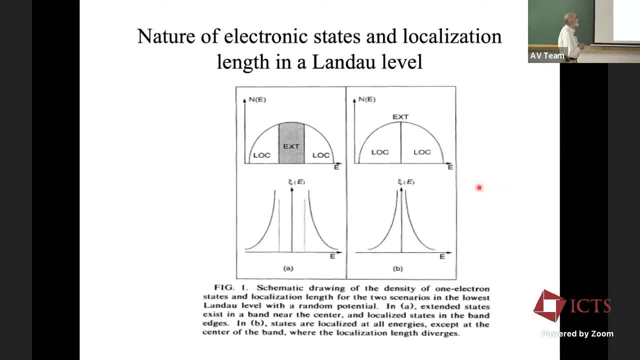 states to be semicircle. it just was easy to draw that And the idea was at that time the feeling was the so-called extended states, at any given temperature, were those states that had a localization length of z, length scale that was larger than any, you know, inelastic and scale in the problem, and so 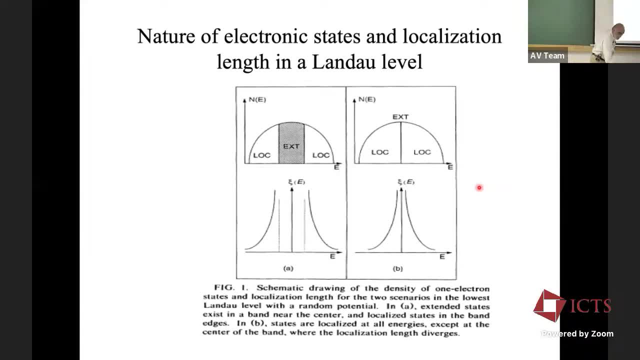 the true zero temperature result is exactly this. but one can ask the question, and that was certainly in the early days. the question was asked: is there really an extended band inside the Landau level? we know now much better that that is not something that one would expect, because if 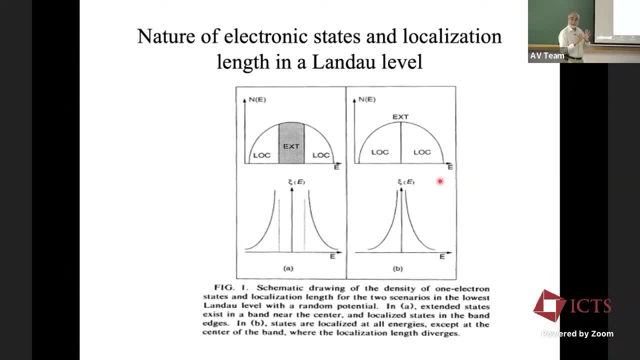 that were the case, then the step would stop becoming a step. it would because of extended states in the middle of the band. so the true picture is the one that is drawn on the right, that there is only a one critical energy at which the localization length will diverge in. 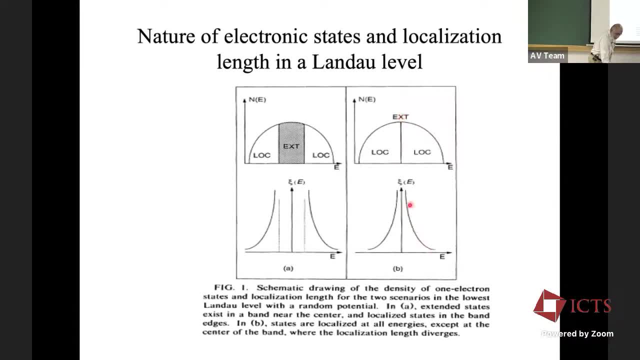 and and the divergence of the localization length is shown here. it for a symmetric potential disorder, equally positive or negative, which is usually not an experiment but more. and you can do it in numerics, you can do it in theory, because that's something that's easier to handle. okay, all right. now, that does not. 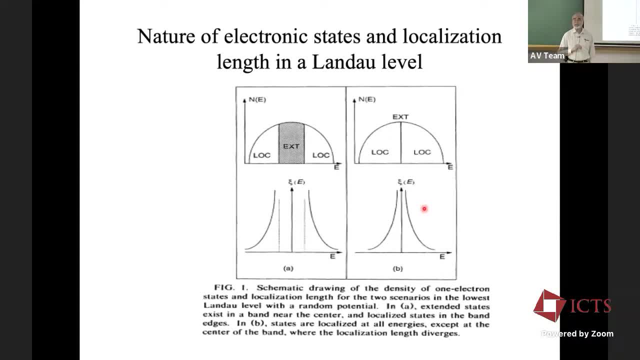 mean, and this was something that was misunderstood for many, many years. in the early days, they thought that it meant that there was a single state at the center of the band that was delocalized. everything else was localized. that is not true and we i'll show you explicitly through numerical 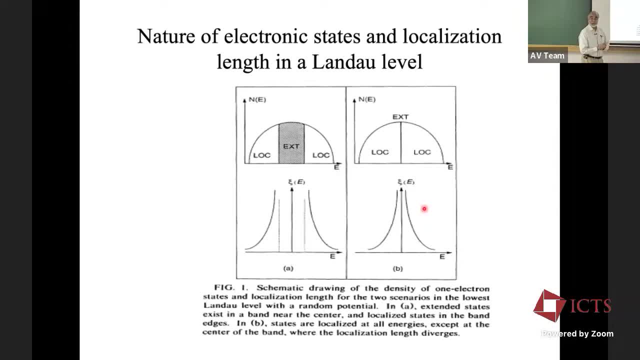 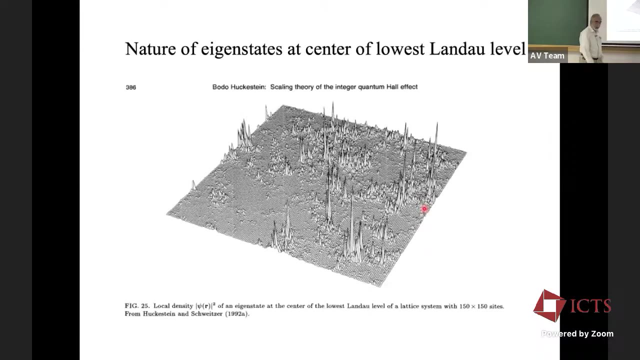 calculations, that that kind of a picture is wrong. it is actually a lot of states, but they go in the thermodynamic limit. they are at this, at the energy e equal to zero. okay, so if you want to actually look at uh eigen states, you can take it this, you can model this system, you can. 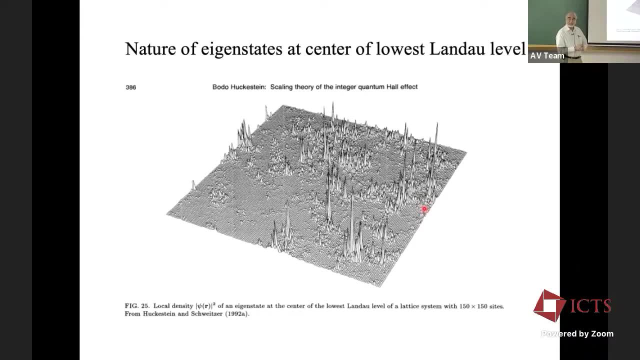 add a random white noise potential and, uh, diagonalize and get the eigen states. so here is actually work done by border hookerstein and ludwig schweitzer in 1992 showing what is the local density that is the wave function. since it's a complex wave function, this is a complex emission. 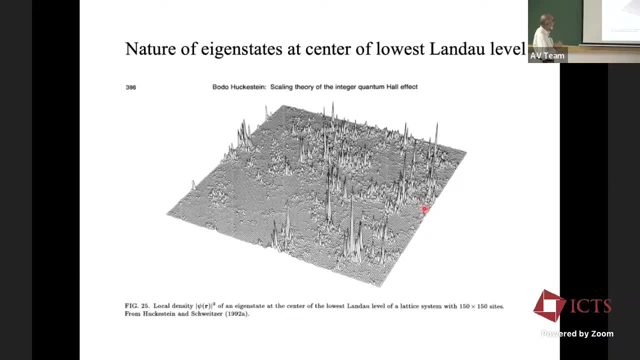 eigen value problem and if you look at the density of agradation electron in corresponding to that eigen function, that is psi r squared and that's what it looks like. it's very, very complicated. it is what's known as multifractal state. it has peaks and then there 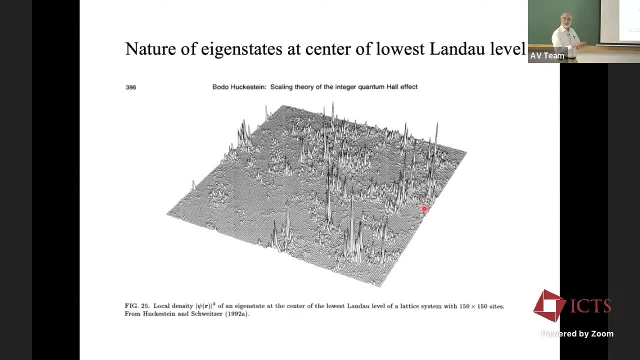 are peaks within. you know, you get rid of the top peaks and then you'll find smaller peaks and then you find smaller peaks, even smaller, etc, etc. and if you really wanted to analyze, you wanted to describe this wave function. it has to be done in terms of multifractals and that's a whole. 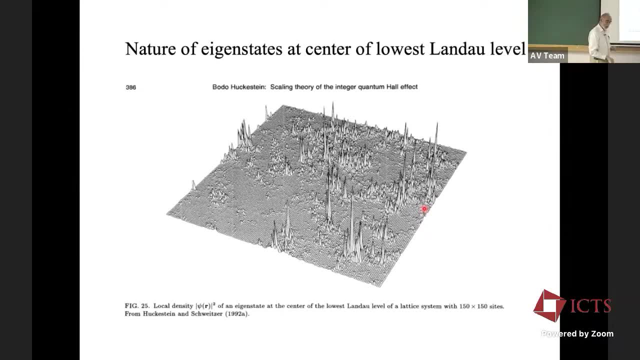 sort of subject in itself. i won't go into that. i just wanted to show you what this wave function looks like. it's not a very simple plane wave like wave function at all. it's very complicated and the precise nature does depend on the disorder- precise disorder that you have. but 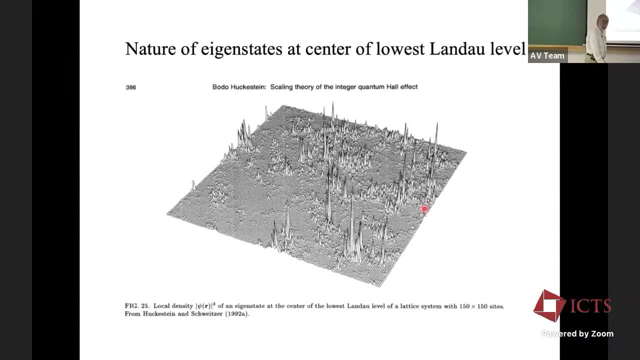 statistical properties are the same. on that, the disorder mean the, the, the, no, no, no, i don't mean that. i mean that the precise geometry of this depends on the disorder. that's all. so that the disorder is not at the scale of that, yeah, etc. all the same, right, exactly, if you, that's what i said, if you take any statistical property based. 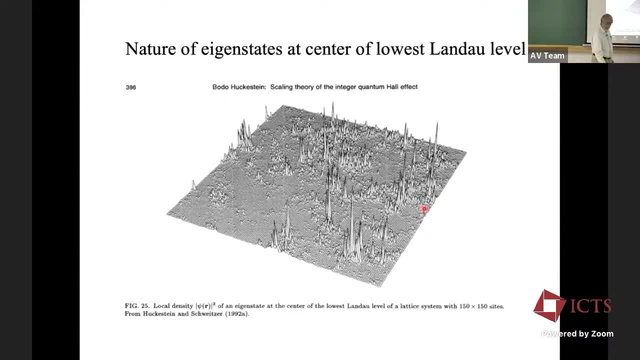 using this wave function, you'll get the same answer, but there's a lot of things you actually don't have to do to make that less simple. so what are the phenomena and what do you mean by nature of the disorder? what do you mean by nature of the disorder? 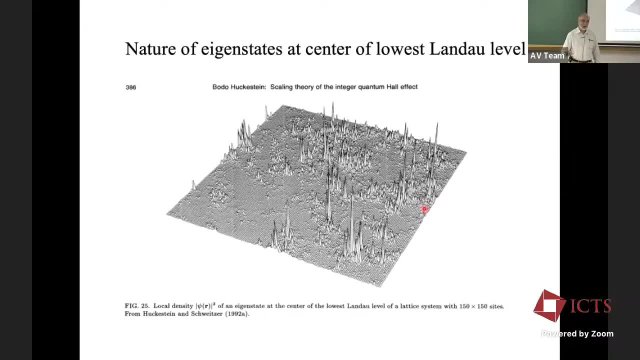 sure, if you do, if you make it correlated with the power law correlation and you know the small enough power law exponent, there will be changes of course. so the all of this is assumes that the disorder it has finite correlation length or most of the most of the numerics, is actually done that as well. so that's how it changes the Wonder Law. 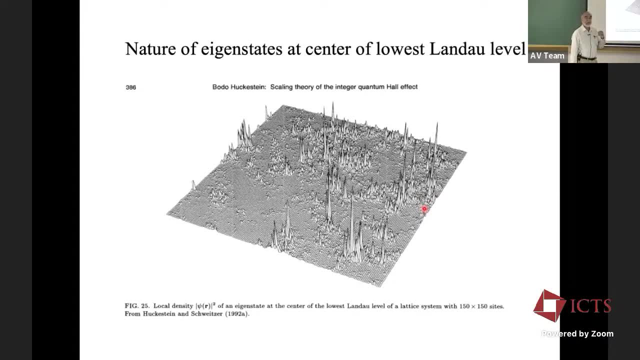 with zero correlation white noise. Now, for those of you who might be interested in doing pursuing this, you should. there are some words of warning. White noise potential works perfectly in the lowest Landau level. It turns out in the upper Landau levels. it is not a good random, this thing. 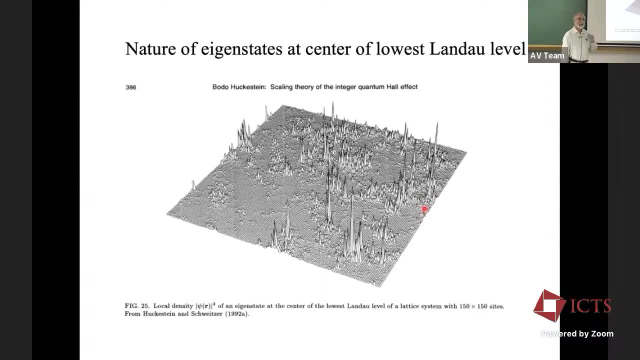 You want to put something that has a finite extent, not zero extent, and I can discuss that with anyone who's interested, but that's a technical point- that it turns out that Landau level it's only the lowest Landau level where you can model with the white noise potential and 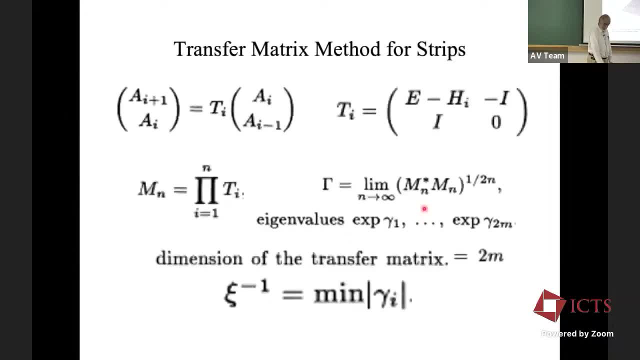 and everything is well behaved. So how do you actually extract the localization length? And this? I'm going back to a slide that I had shown when I was talking about Anderson localization, because the same method is used there, which is Sorry. one more question. So in this numerical definition, so if I think about the number of 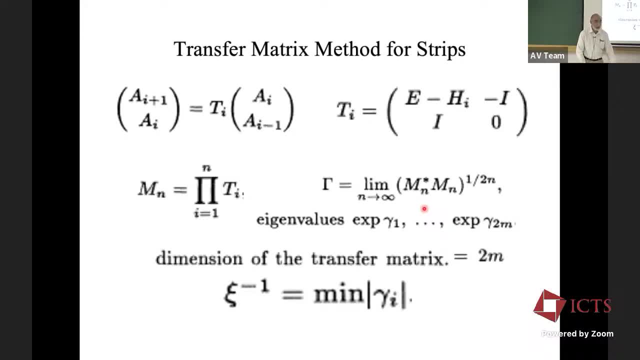 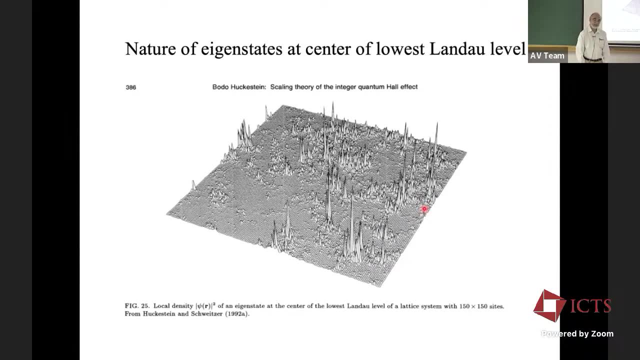 zero energy states at the center. extended that's not one, but then it's like a vanishing fraction of it. So does the exact number of of 100 energy states depend on the disorder Or a given system Like, say, 150 plus 150 states? 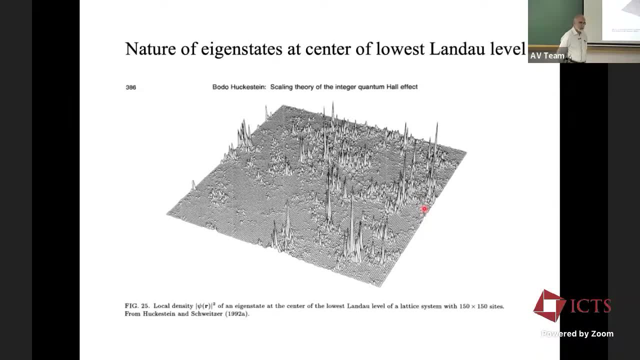 Sure, of course I did that. of course, if you have a finite sized system, how many states are clustered around the zero energy can precisely where they're clustered is also, it may vary a little bit. So now, if I take the system at the number, 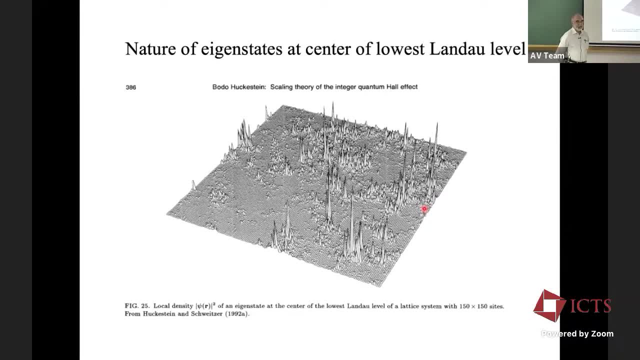 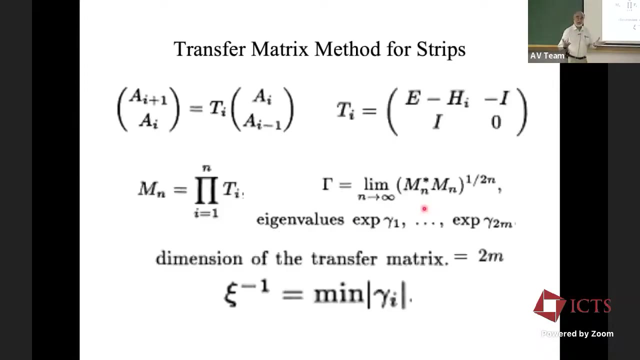 yeah, the number. then the number is is it's fixed in the sense that it goes to a certain average number. I'll show you that data. in fact, I'll show you that data. okay, so one of the most used methods for finding out localization length for any. 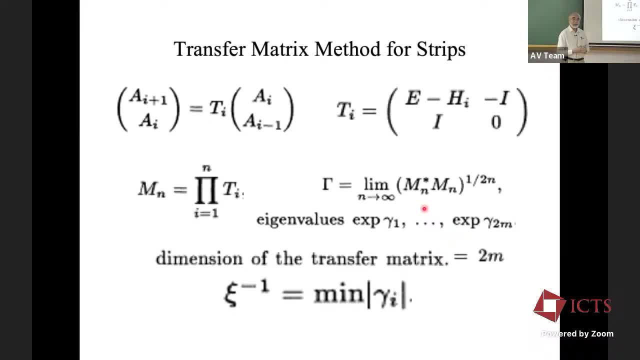 whether it's a three-dimensional system or a two-dimensional system is to start with the two dimensions. so in this case it's a two-dimensional system. so you start with a square and then you extend this length. so there is one length scale on out here, which let me see if I have the second slide in there or not. no, I 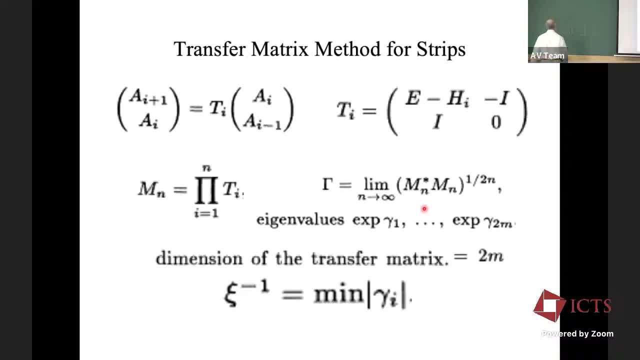 don't have the second slide, all right, then I I'm free to use what I want. so let me assume this is a two-dimensional system and then I extend this length. this has M I against effectively M wide, and this length, L, is going to go to. 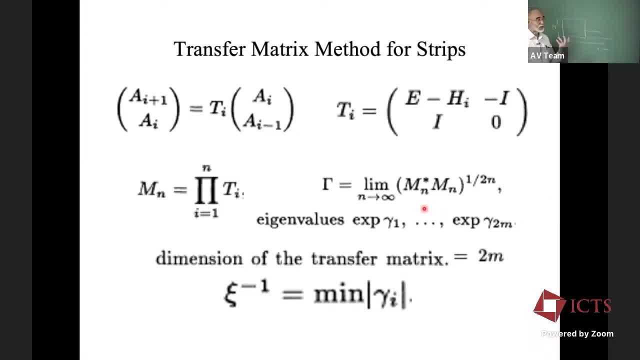 infinity. and what you do is you try and find out the localization length for this finite width one-dimensional strip. it in the end becomes one-dimensional because only one direction is going to infinity. the other direction is finite. okay, and so the way you do that is you, you write down the wave function on here and at the 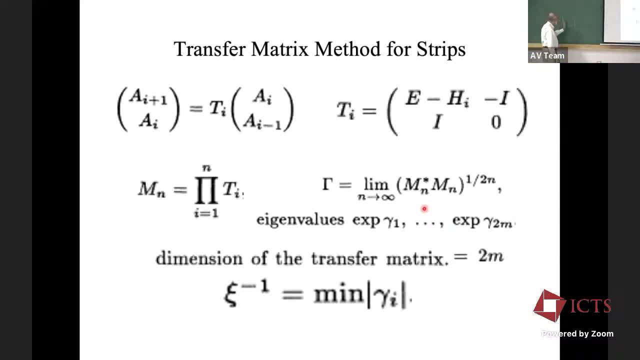 next site, site, and then you use the transfer matrix, which is basically that if you know the Hamiltonian of the system, you know what, and you're looking, deciding what the energy is that you're trying to model, then you give. the transfer matrix is just given by this. 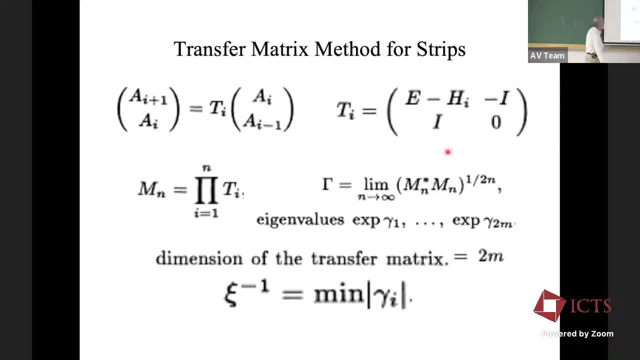 this combination right here and you can, starting with these two, you can then get the next two, etc. etc. and you can keep on going. and then what you do is you look at the transfer matrix product of all these TI's and, of course, what's going to? 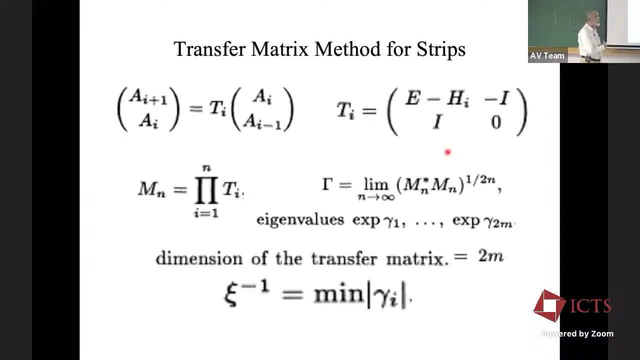 happen is that some eigenvalues are big and some are small, so you start getting more and more of one eigenvalue compared to the other. but you have to. you have to, In that case, look at this, this average, that is basically the product matrix multiplied by its complex conjugate to the power one over two, n, where n is the number of transfer matrices that you have multiplied. and look at the limit- n, going to infinity- of the eigenvalues of that matrix: gamma. 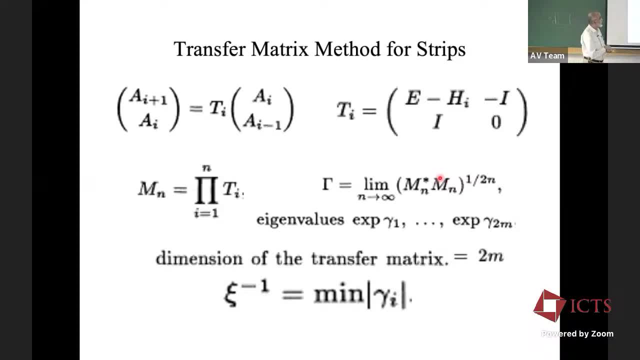 And the eigenvalues are exponential, are represented as exponentials of what are called Lyapunov exponents, gamma one to gamma two, m in this case, and the inverse correlation length is the minimum of these Lyapunov exponents. So you do this procedure, you go ahead and find out the minimum eigenvalue, gamma one over two n. 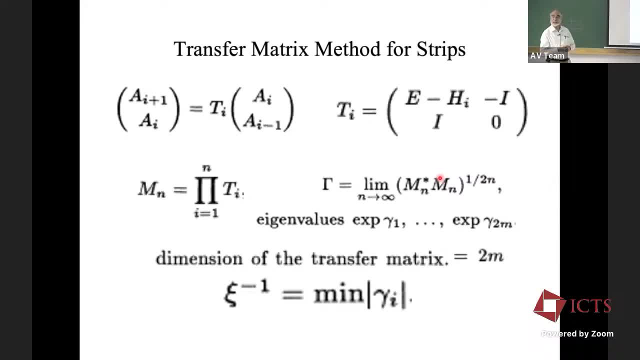 And the inverse of that is the localization length. It tells you what is the longest length scale in the problem. Everything is decaying, but the longest length scale of the decay is the one that's the localization length. Now this is well defined because there's a mathematical theorem that in one dimension, with any disorder, you always have eigenstates with finite localization. 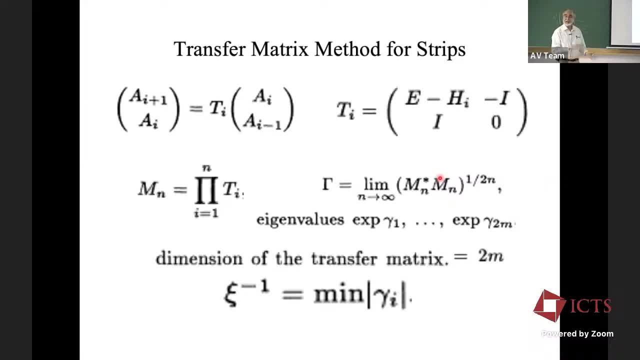 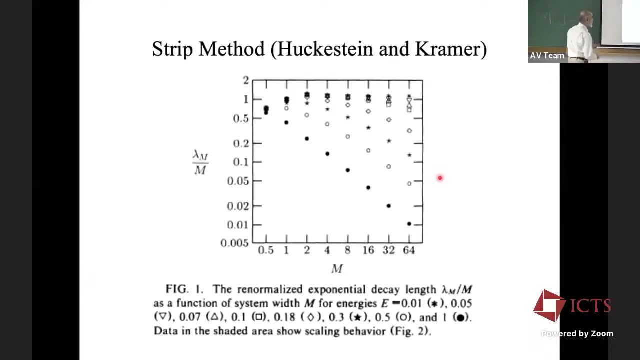 So there is no problem, You're not going to get any zeros or stuff like that. You're going to get some small number, but you're going to get. it's always going to be finite. So basically, of course now the decay length. since you have a parameter m in here, the width of your sample, the decay length will depend on m. 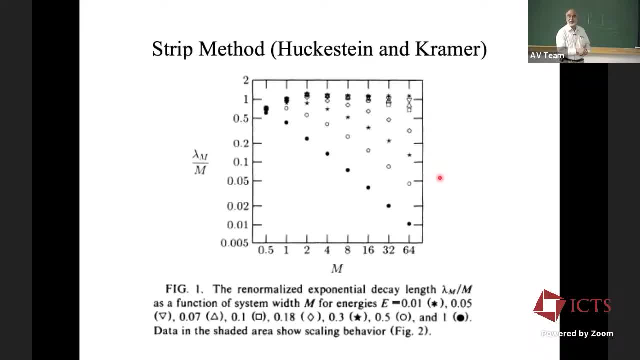 Because it's an m by infinity problem, not a one by infinity. So it's a one dimensional system, and so the expectation is that lambda m over m will be some universal function of m divided by the actual localization length. So first I'm showing you what the actual data looks like, without any massaging. 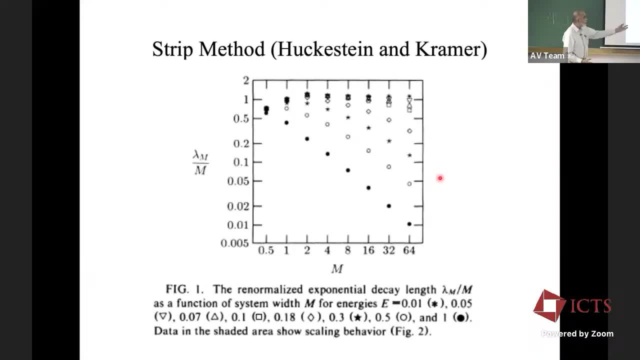 You just look at lambda, m over m and plot it versus m for different m's. I don't know, I don't know how he did 0.5, but that's you know. this is actually a continuum problem. So therefore, I think the m stands for the ratio of the size of the of the system and the magnetic length. 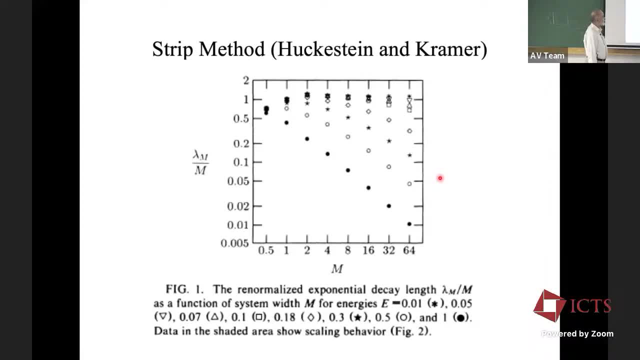 So, going from 0.5 to 64, what you find is you get a series of curves that depend on the energy that you have. OK, so the topmost curve, which is which is that one right there, is coming at energy. 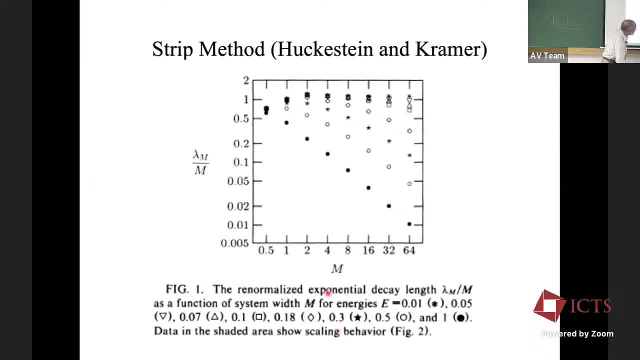 0.01,, that's, that's this one right here. 0.01,, all right, And then at 0.05 is the next curve, then the next curve, then the next curve. Now, if these were all localized, then all these curves should actually go down as m increases for every energy. 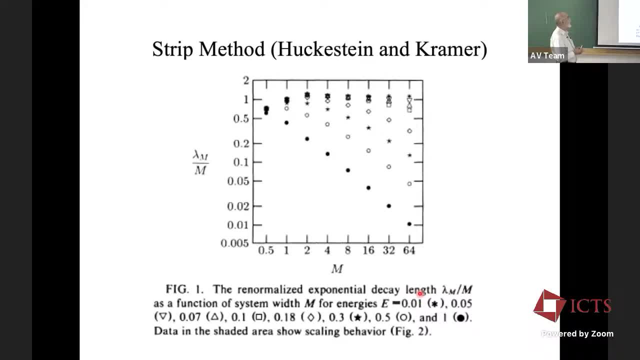 But do you notice that there is a little bit of a non-monotonicity for near the center of the band At least there's non-monotonicity for small m. So you have to throw that data away because basically that's saying that these are very strongly finite size, limited data. 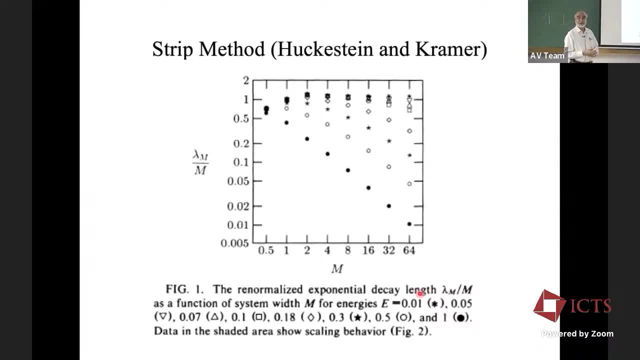 And so we are not going to expect long distance physics to come out of that. But what you can do is you can take the data for larger m for energies. You know you don't want to be far away from the center of the band either, because you don't expect the asymptotic behavior of the localization length to be true for all energies. 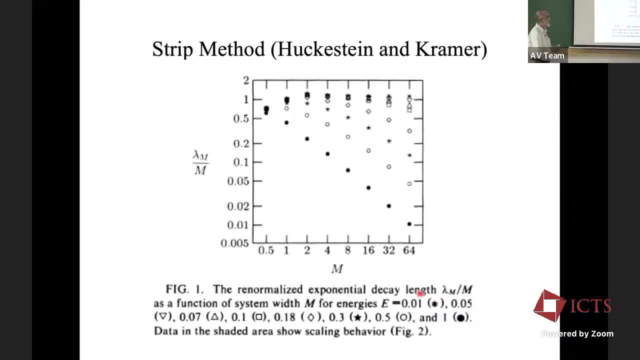 It is only near the center of the band that it is true. So you have to play this delicate balance of keeping the lowest energies where you think the data is reliable. If you could go to a much larger m, then even 0.01 would work. 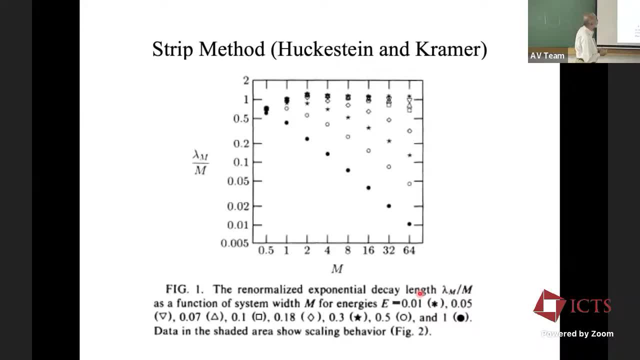 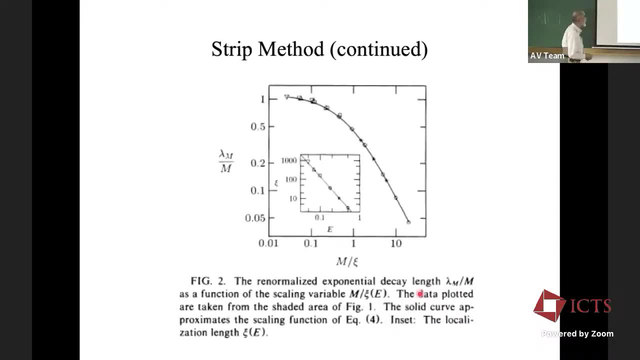 And in this case It probably works beyond about four or eight, but it doesn't do a great job. So let me show you what exactly, in the end, it's done. What you take is you take the data that you have And then you say that, depending on the energy, there is a localization length: psi. 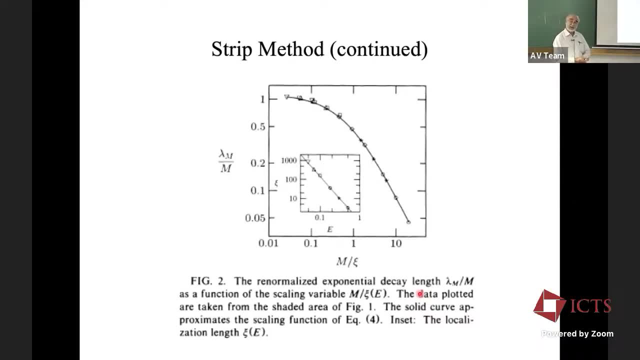 And how I'm going to determine the psi as a function of energy is I'm going to make sure that all of the energy that I have is equal to the energy that I have. All those data lie on a single curve, So for each energy, 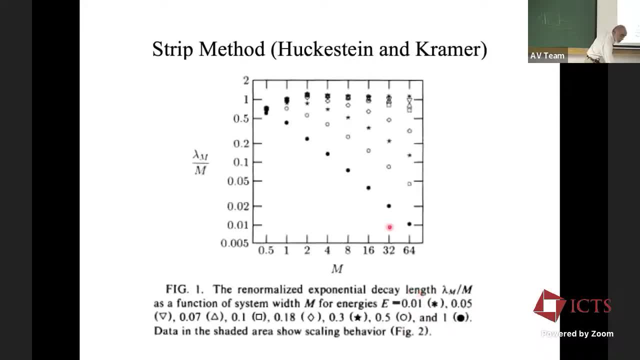 So there are all these different curves that we have This one and this one and that one and that one. I'm going to assume that psi has a certain value such that when I divide it m by psi, All these curves will collapse into one. And you can see immediately that that's not really what I'm going to do. And you can see immediately that that's not really what I'm going to do. And you can see immediately that that's not really what I'm going to do. 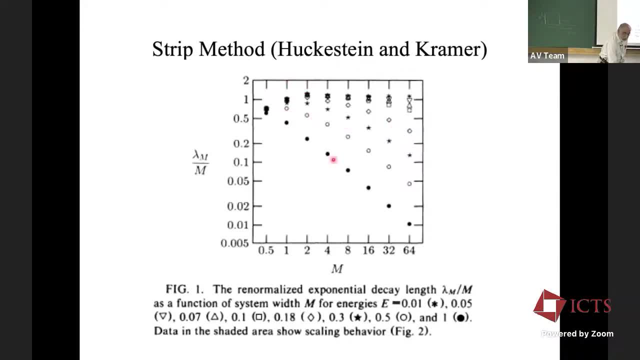 And this is going to happen out here, because this is an upward bending curve And this is a downward bending curve, So no matter how much collapse you do, it's not going to fit. So that tells you where you're limited by finite size. 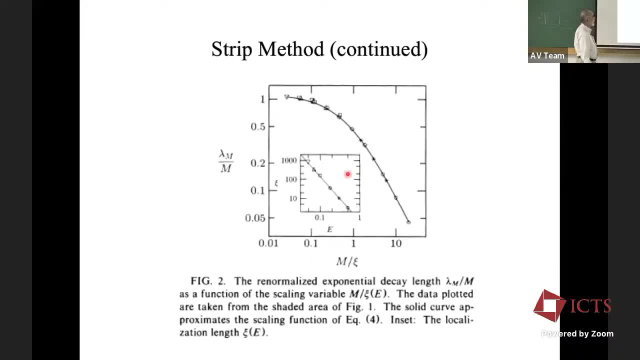 OK, but a lot of the data does seem to fit one single curve. And then, of course, what you do is: then you plot your psi that you determine by forcing all the curves to lie on top of each other. And then, of course, what you do is: then you plot your psi that you determine by forcing all the curves to lie on top of each other. 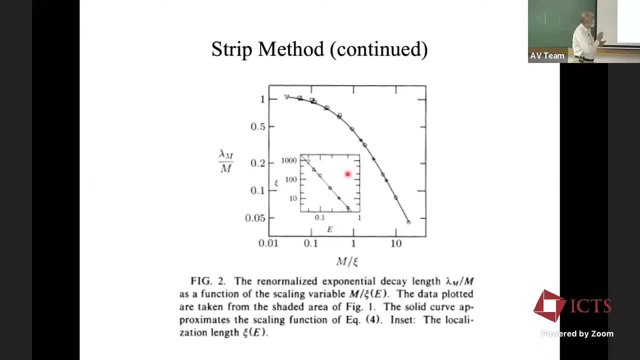 Versus energy on a log, log plot. And that's the inset, right here, with right, this one, And then this slope of this curve tells you what is the how it goes. And this is work done by Hookerstein and Kramer And they found that psi goes like e minus e, c to the minus two point. 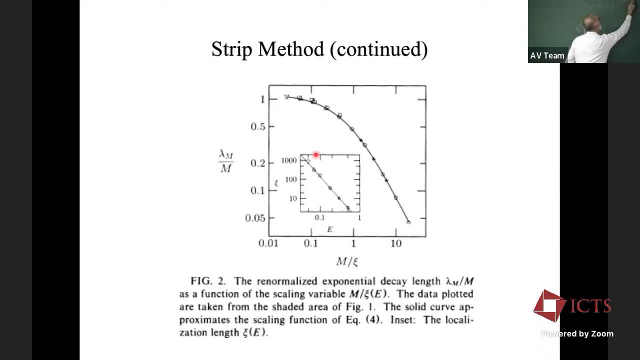 The original work was 2.34 plus minus 0.02,, I believe. So that is how you determine it. Now, those of you who might have attended this morning's lecture, there are many more works that are very similar to Hookerstein and Kramer. 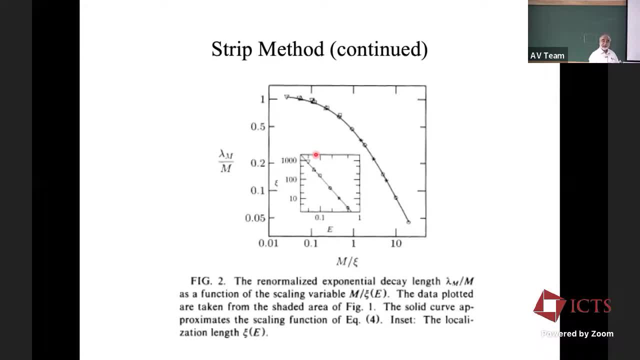 But they go to bigger sizes. They analyze the data a little bit more sophisticated way, They allow for irrelevant variables and then get psi of e And the claim is in the latest set of papers that some I would like to be. I'm not exactly sure what I should write. 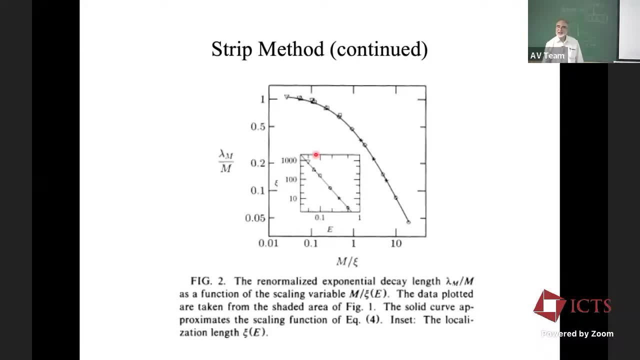 But it's certainly this is. the answers are 2.6, with probably not more than 0.05 away from that. There are lots and lots of different groups that have got that. So This is all numerics. There is no. 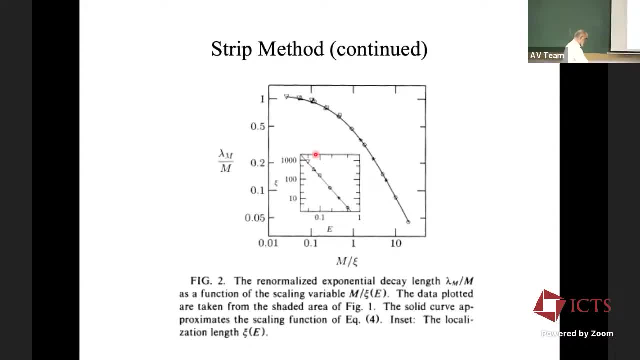 So there is work done by Martin Zornbauer who is actually claiming that this exponent actually is infinity And it's logarithmically dependent on the length size. Of course, numerics will never get that. I think we- I would say most numerics- don't actually agree with that. 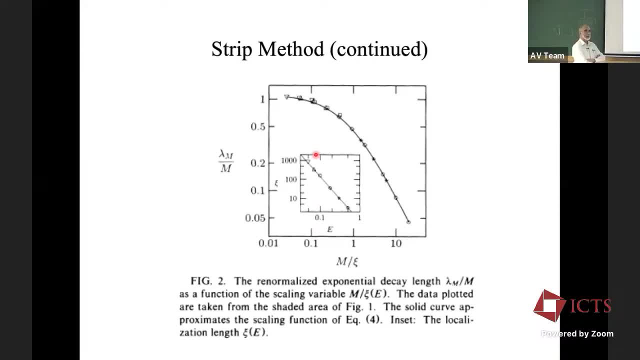 If the coefficient, if there is a logarithmic dependence, the coefficient of the logarithm is very small, And so it's so small that it is not numerically really detectable, And so I'm not really sure that's that, that, that field theory that Zornbauer has. 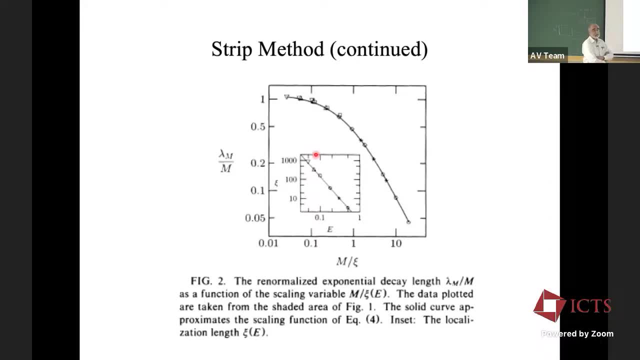 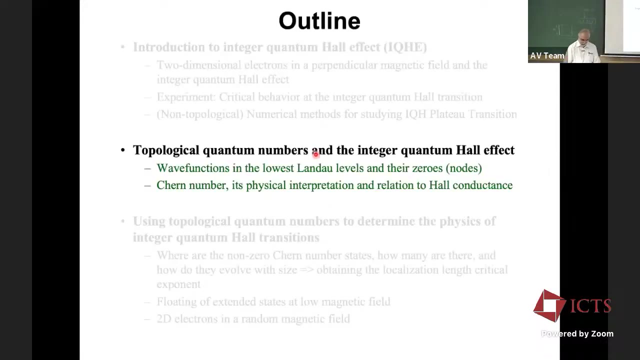 Is the Final word? Yeah, right, Yeah, I'm with. He showed that it's very peculiar in the quantum Hall regime. Yes, So I want to actually tackle the problem slightly differently, because When you take the data like this, 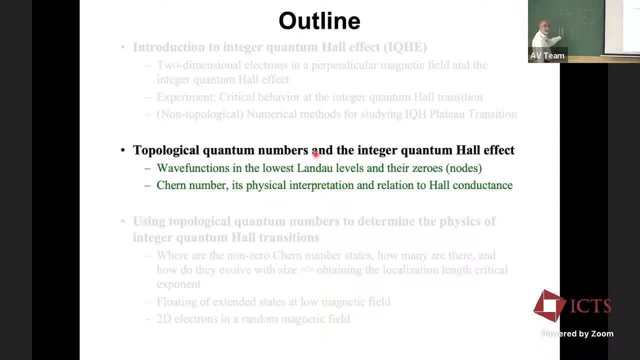 You're actually taking a two dimensional problem and converting it into One dimensional problem, And so there are many fitting parameters that you have first have to extract the localization length for your one dimensional system, then see how it scales with the size of the width of the system and then extrapolate to get the answer. 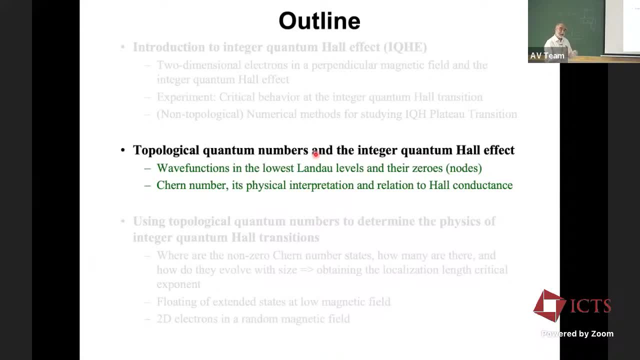 So there's a lot of jugglery that's involved there. In addition, More recent data that said that this number is actually not right, but this number is more right. I'm required, So I not just to go as that, but there are corrections to that which are sub leading. okay. and, of course, if you have more parameters and you have numerical data with some uncertainty, with some error bars, you can fit the data and get different results. 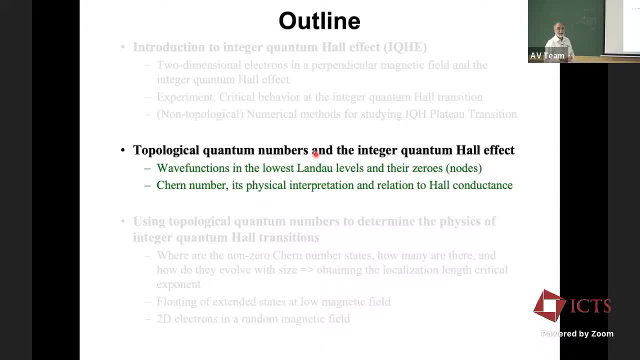 After all, the data has only finite fidelity you can. if you put in lots of parameters, you can get Many things. So that's a that's a real issue that I think needs to be sorted out. so we decided Some years ago that we should really try and understand these eigen functions from a different point of view, and so i'm going to talk about 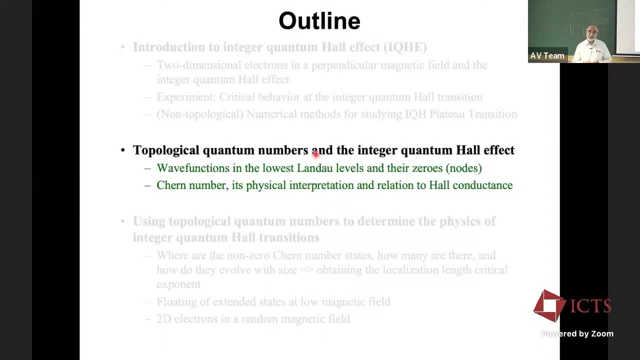 A paper that I wrote with Dan or over some Duncan holding in 1980s, when we first started understanding these wave functions, and then What that? that led us to a way to estimate The localization, then exponent, and i'll describe that- that method. so this is a very different method. it's only going to talk about two dimensional system. so it's l by l, and then we're going to change l. 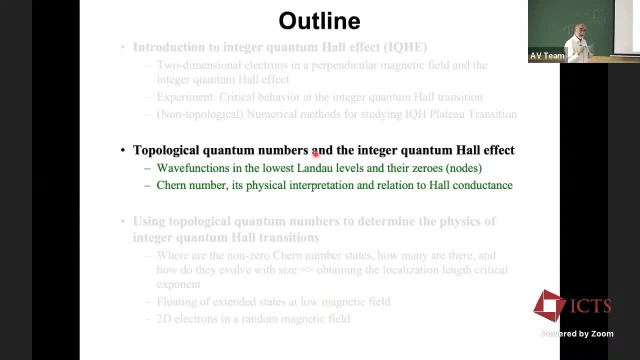 Okay and see how properties change as a side of the size l changes and then try to extrapolate to l equals infinity. but we are not going to change the dimension of the system is going to remain two dimensional And there's some other things that are that are very 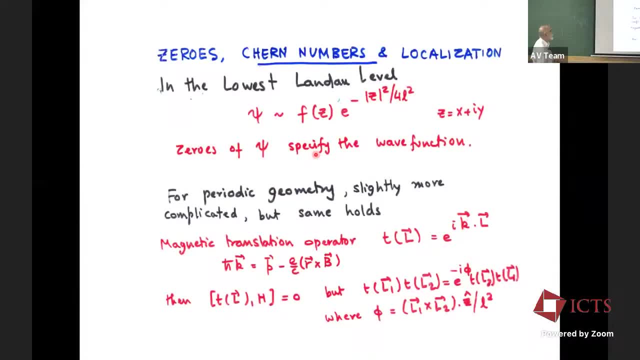 Interesting about this, the method that we're doing. okay. So in order to do that, I want to try and go through the nature of the wave function than the lowest land In the lowest land, our level. the iron functions are some analytic polynomial function of the complex coordinate Z, which is 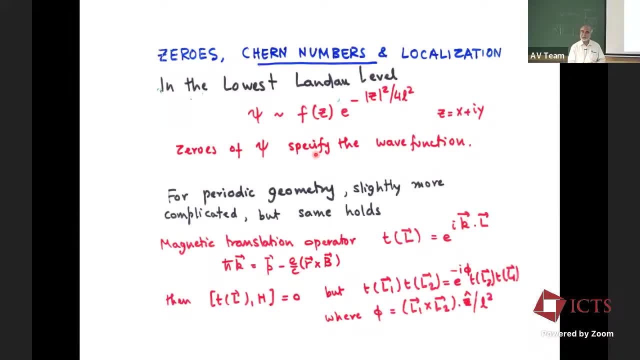 X plus I, y. X and y are the coordinates of the electron and if you create the complex coordinate Z, X plus I, y, then all the way functions single particle wave function. they just function of one variable, Our function of Z times the gaussian factor E to the minus magnitude of Z squared over for l squared with L, is the magnetic length. 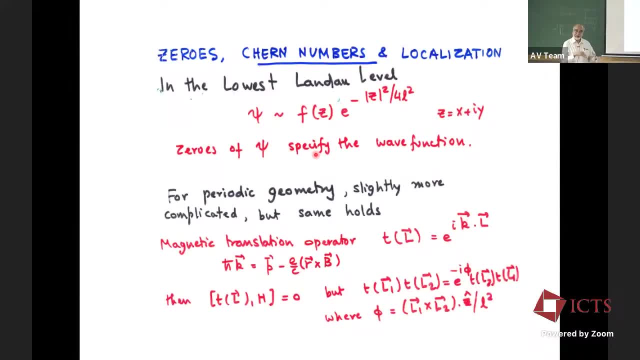 And L is square root of EV. Sorry, The length goes down as the magnetic field goes up, so it goes as one over square root of H. Now suppose you have a periodic geometry rather than infinite space. okay, so i'm not talking about a two dimensional sample, l by l. 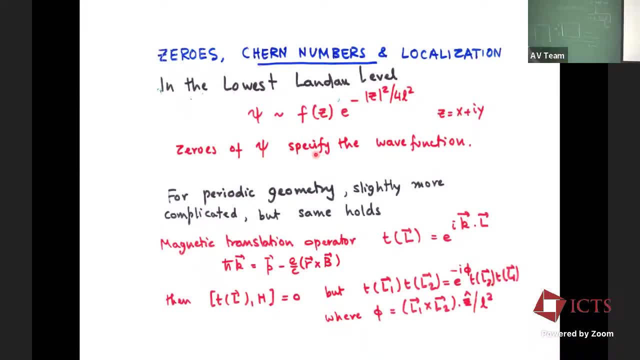 And of course I can talk about very large l, l and that That's, that's represented by that wave function. But if you have a finite sample, you can put in periodic boundary conditions. Okay, you can imagine you, but you can put it periodic boundary condition with a twist angle, because this is the 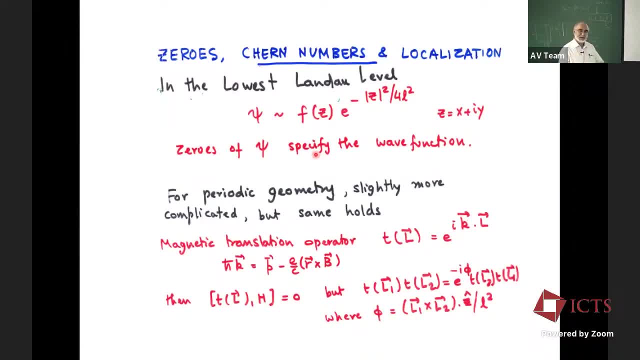 You know, if you were talking about Anderson model, you can put periodic boundary condition or anti periodic boundary, Okay, that is, you change the sign of the wave function when you stitch them together and actually that's one way of finding out conductance of a sample. 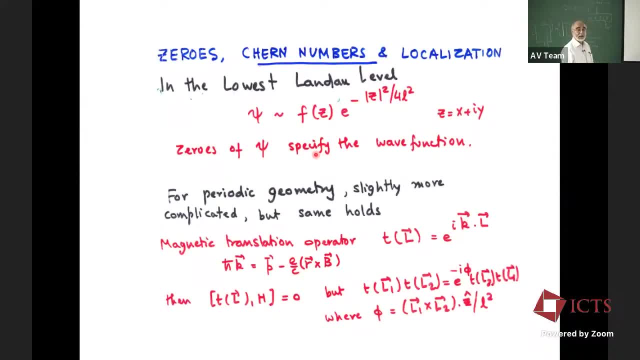 Since here it's a complex hermitian problem. you can have any phase angle E to the i theta, so there'll be an E to the i theta x for this one and another E to the i theta y for that and but because The magnetic translation operator as defined there 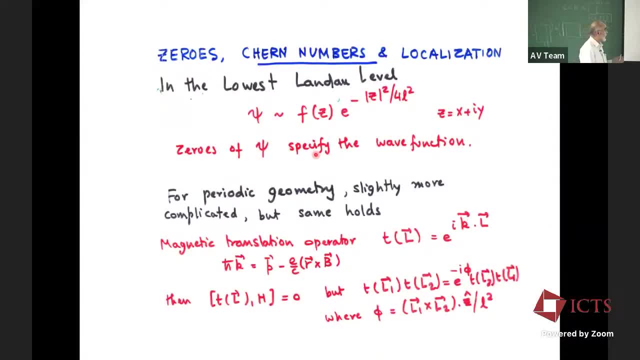 commutes with the Hamiltonian And but the magnetic translation operators don't commute among themselves. so in a sense it looks like blocks theorem in for crystal structures. but there is a, there's a little twist to it, which is this one right here, they are not. they don't commute. 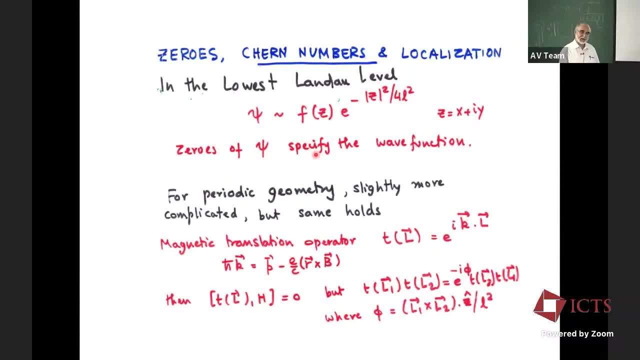 The translation operator for l one times and multiply by the translation operator. well to Not the same as putting the translation In the two. in the opposite way, you get a, get a phase factor, which is basically the flux through the, through that black bucket, l one. 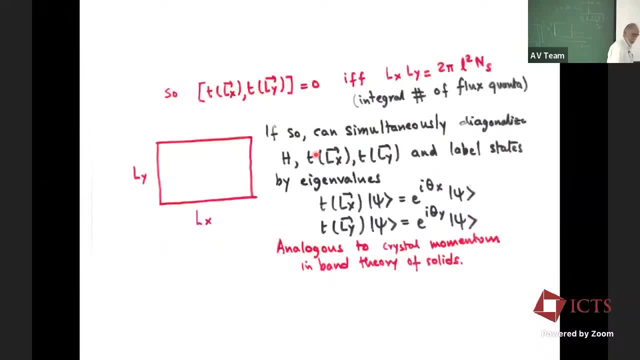 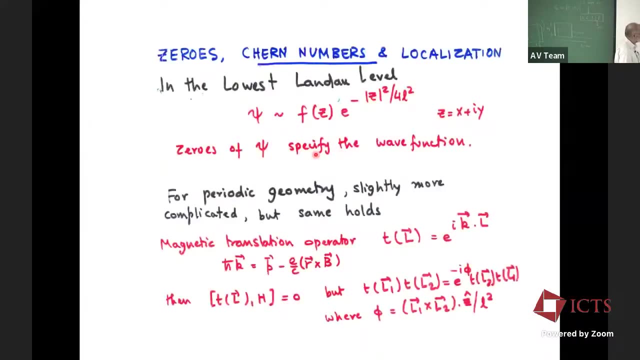 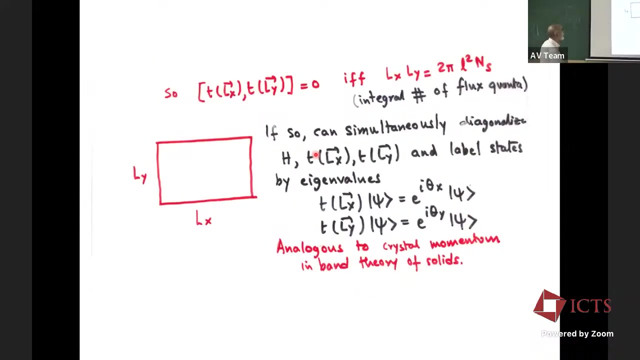 By l two. However, If that flock, if it is such that there's an integer number of two by, If I is to buy times an integer, then of course they do commute. But It is equivalent to saying that if there's an integer number of flux through the sample, then there's come. 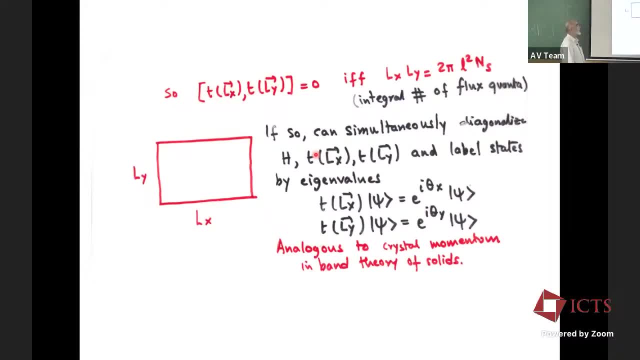 If that is the case, then you can simultaneously diagonalize h, t of l x and t of l y and you can label the states by the eigenvalues Of the translation operator, just like in periodic lattices. you know that they have eigenvalues with modulus one. they're just a phase factor, okay. 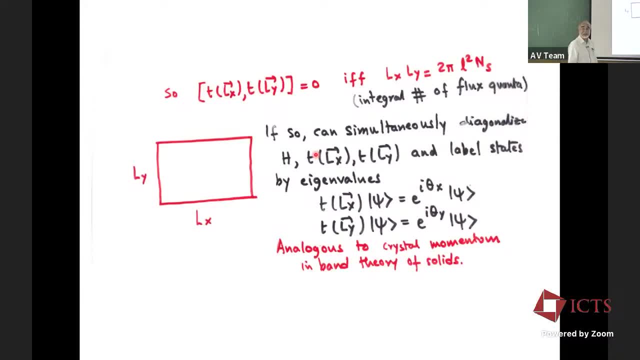 So it is very analogous to crystal momentum in. but you can only do it if there's an. your sample has a size with an integer number of flux, one First numerically you can do that. you can choose your sample to have that okay. 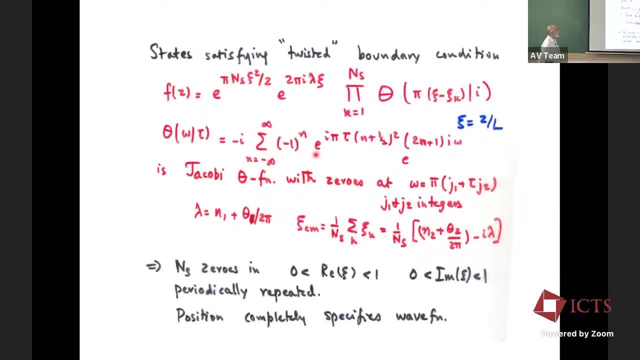 Then it turns out you can actually write down and actual the wave function instead of you know some polynomial. in Z times, The Gaussian factor, you get Jacobi theta functions and those who are mathematically inclined can go play with them as much as they like. but one property that we are going to use which you can prove using those Jacobi theta functions is that in the actual 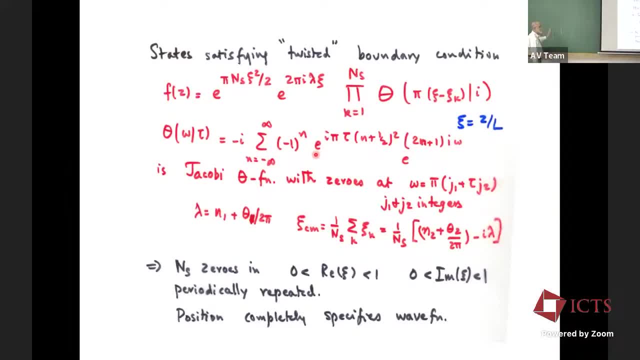 Sample. okay, there are precisely As many zeros of this complex wave function As there are flux, as the flux through that sound. So, and, moreover, it turns out that if you know the position of the zeros, You can write down the wave function. that's all. so there's a one to one correspondence between the zeros of the wave complex wave function. 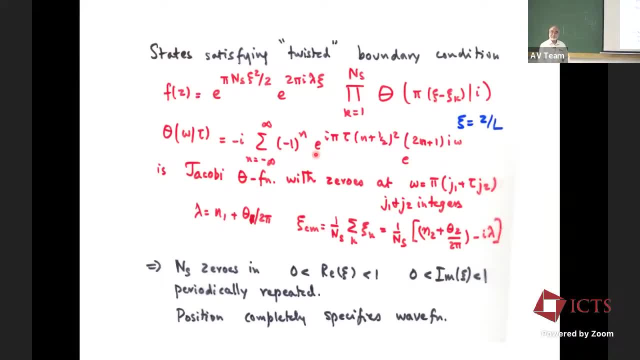 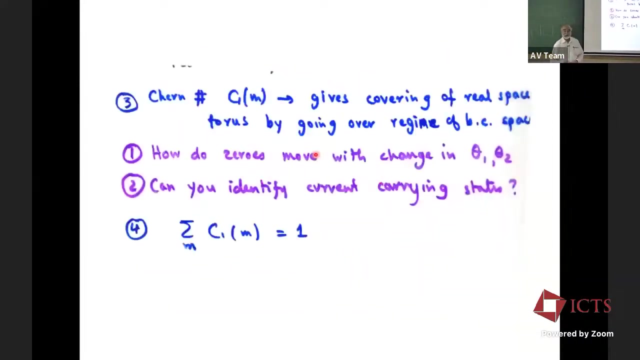 And the Functional form of the wave function, The wave function of the Right right. No, no, yeah, no, that's just a flux to the sample. So we we said let's try and analyze this. what's going on how you see, I had this. 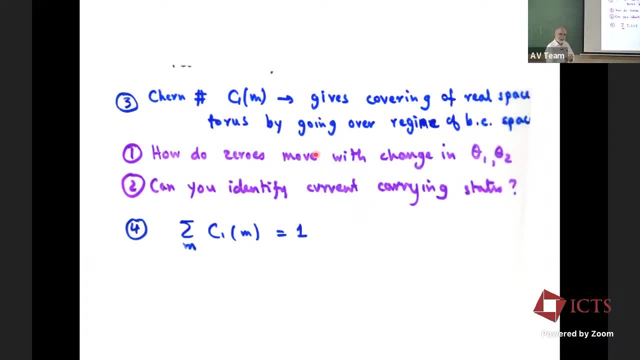 This idea coming from localization, that powers had this idea that you know how much the eigen state and the eigen function changes if you change the boundaries from being periodic to anti periodic determines whether it's what the conductance of the eigen status so tells you something about localization properties. so the question I asked Dan rovers, who was a 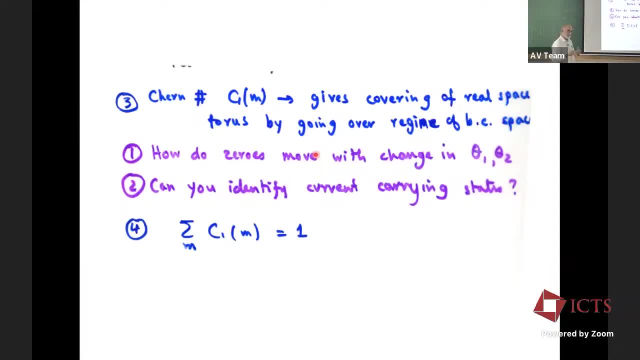 Summer student at Bell labs. was You change the boundary condition? see what the zeros are doing. can we identify a localized state by saying that the zeros are all localized, And identify an extended state in terms of zeros being extended, Extended, were extended over the sample, and how? how are the zeros going to change? you're going to change the boundary condition, so what you do is you. 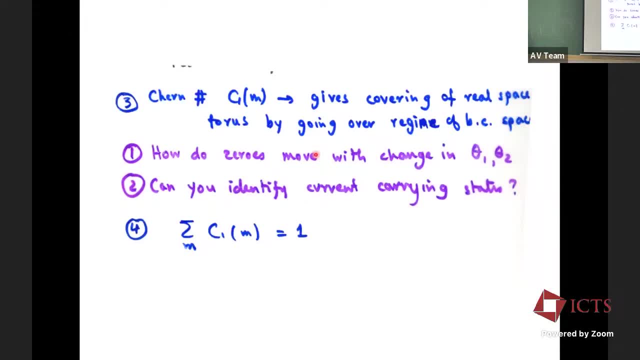 This is, This is Theta X going from zero to two pi and Theta Y, which is from zero to two pi. and you make a grid in here, very fine grid, And you solve the problem for each boundary condition, and for each boundary condition you have ns zeros. and so you, somewhere those ns zeros are there, one, two, three, four, let's say it's for for eigen states. 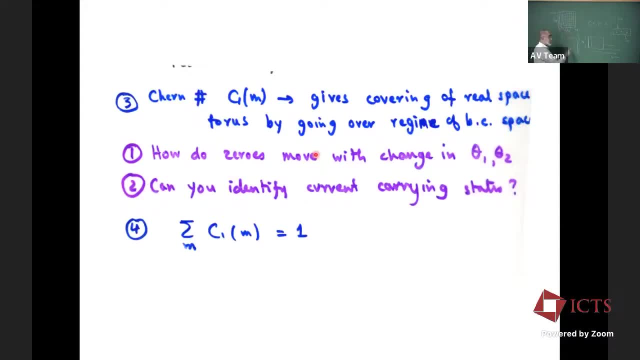 Then there are four zeros, then you go to the next boundary condition. these zeros will move And you keep doing that. cover this whole A boundary condition, space up and see what happens to the zeros. and I had this naive idea that if you had an extended, say, the zeros will go all over the place and if the 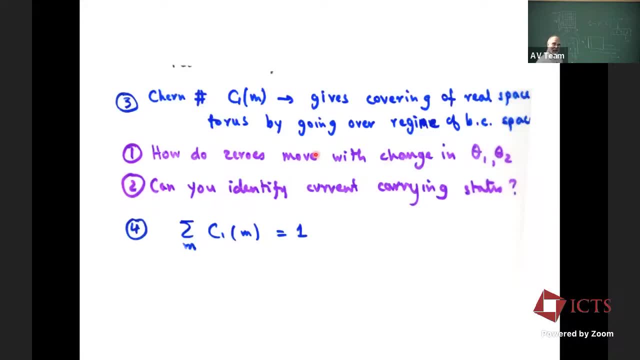 I can say it is not extended, it won't really care about the boundary condition And therefore the zeros will just stick around where they are. So we, in the end, we asked: how do the zeros move when you change the Theta X and Theta Y, which I've written as Theta one and Theta two in there, and can you identify states which which are actually extended and carry current and give you the whole effect? 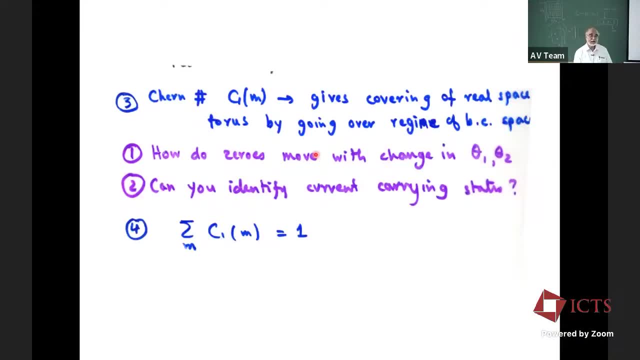 Now it turns out that actually, all These states are We. we learned, as we did the- we're doing the calculation- that there is a topological quantum number associated with every state. that's called the churn number, and this is an integer quantity. Okay, and it turns out that this churn number basically gives you: 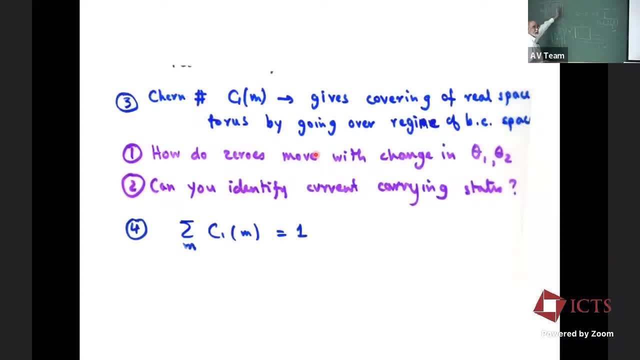 That if you cover This boundary condition space Once, how many times have do the zeros cover? the wheels traverse in the real space and the integer residue of that is the churn number it turns out. So we were right. I mean, my thinking was right- that if it is an extended state it the zeros will move around. 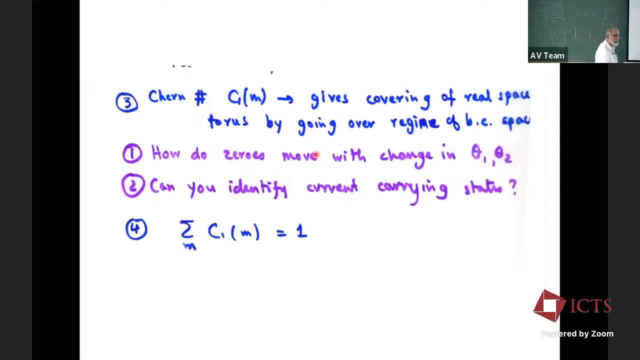 But there was a little bit more to it, which i'll show you in the next few slides. Okay, yeah, yeah, right, We know that now this is 1980, 1980. so i'm giving you, in all these lectures, i'm giving a sense of history. you know, we're, we're, we're in this thick of words and we're trying to figure out our way out. 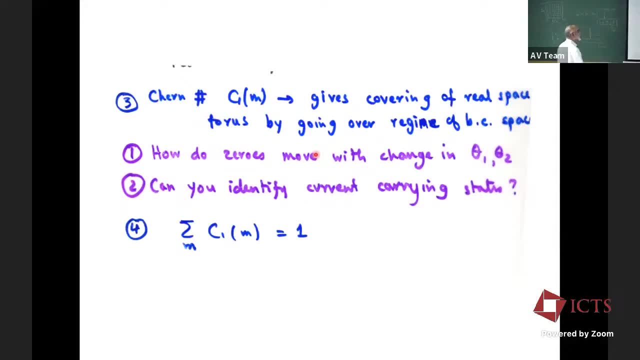 And so- and these are original slides, I have not doctored them, I couldn't write much more- You know very sanitized version of these slides which will go with today's language, but this will be the last slide, But today's language, but this was the language of 1980s. Okay, the other thing of course one knows is that some of the churn numbers of all the eigen states as well. so the first thing you are you might ask is: how do you know that? there isn't that the an eigen state has a fixed churn number? what guarantees that? okay, 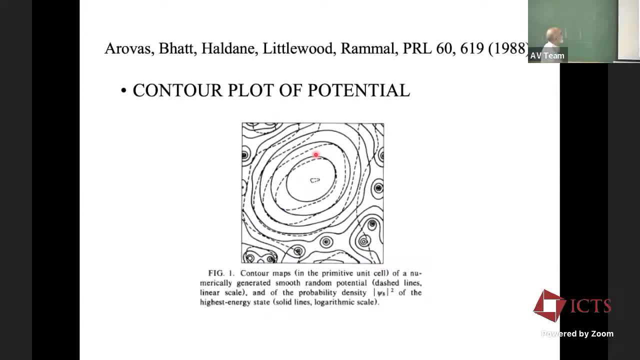 And I will come to that a little bit later. let me show you the put. we sort of took one, some random potential, and that's the equip potential. Okay, The numerically generated, smooth, random potential And the contour maps are given there. and you know, just to give you an idea that this is not some, these are no symmetries whatsoever, it's just: we listen. one example of the thing that we did: okay. 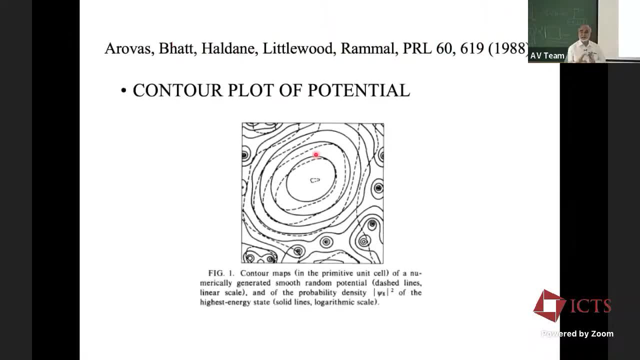 And it turns out that this size that we were able to do and and analyze very well only was eight flux quanta at that time. All right, so it's a very small sample. so there are eight zeros and eight eigen functions, And what i'm plotting now is the zeros. 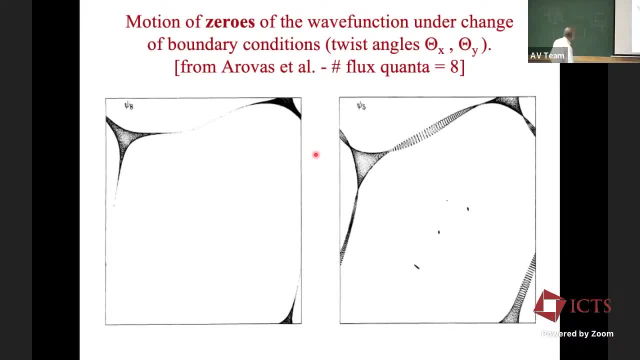 Where? where are the zeros for each eigen state? so what i've done is basically covered this boundary condition space with a very fine grid, and every or each of these Values of the boundary condition angles. I put down the eight zeros and then I asked the question. 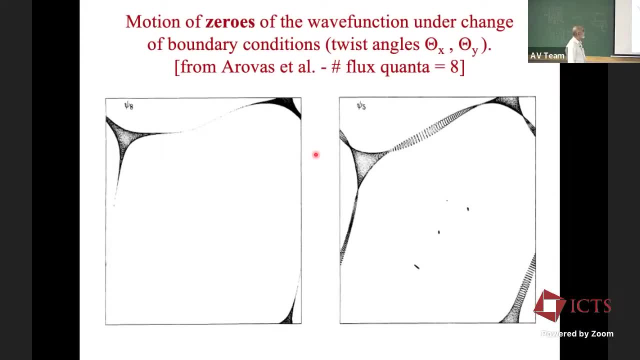 What happens as I change the boundary condition. okay, So unfortunately this one is not showing it very well, but this one here- this is the highest eigen state and there should be some more zeros in here- but Is Not showing them, but one of the things that you see very clearly that even if the state isn't really localized, 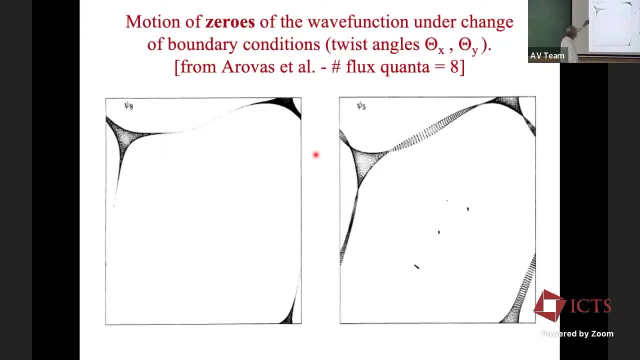 The, the zeros, are not completely localized. there's always one strand that comes this way and another one that goes that way. every one of the eigen states has that, So that's not a good enough. you know, just saying that the zeros don't move is not, is not, is not possible in any of the eigen states. 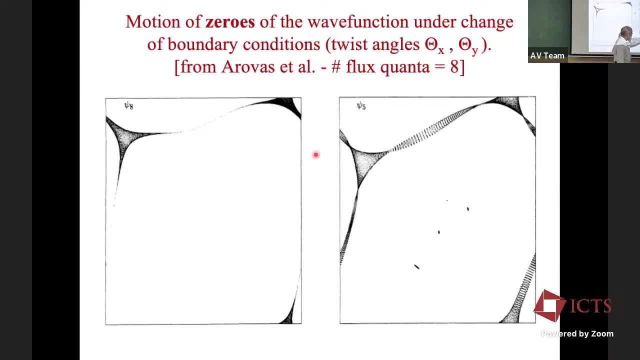 You can see what happens here. some of the zeros are sitting and localized And others are moving around. Okay, but these, both these eigen states, actually are localized. yeah, no, they have. they have zeros in real space For any given. theta one, theta two. 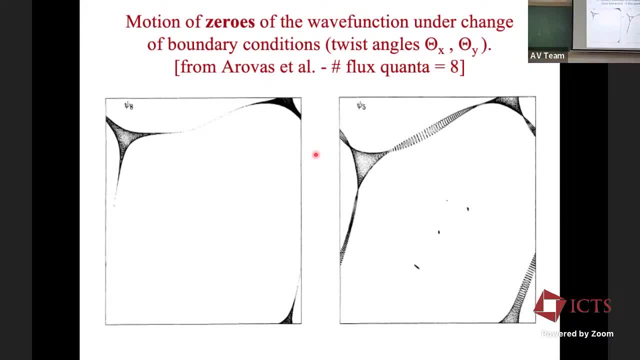 And then I changed theta one and theta two and I asked: how do these zeros move? and these are the figures that they make. okay, And these two states are the highest to stay in this aside. eight- no, this is sci fi, so it is closer to the Center of the band- and basically 1234, up to eight. let me show you some of the others. 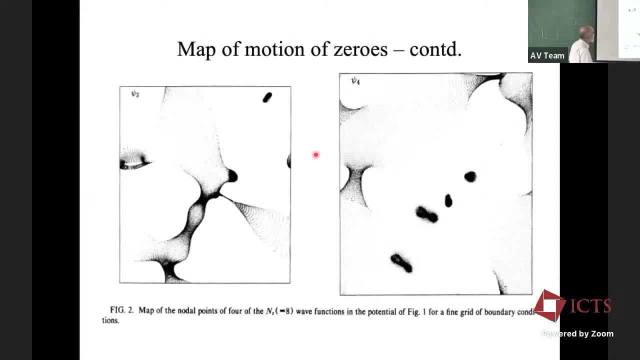 This is five, four and this is side three. now, unfortunately, these These are haven't come out very well in the projection, but you'll have to take my word for it that in this way function. we cannot get any zero here or there or there. 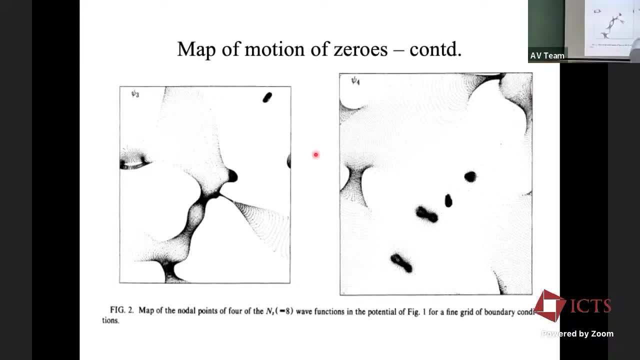 On the other hand, There are these. you can sort of see a little sea of little zeros there. there's a see all over. so basically, this way function side. for I can say: I want A zero here in space and I can manufacture a boundary condition- theta x, theta y- to get you a zero there, but this one and others, I cannot do that. if you say that I want a zero here, this, I again, function will never have a zero. 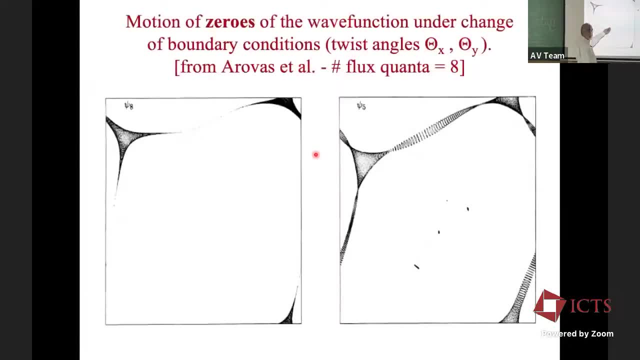 Similarly, when I go backwards here, this I can function will have no zeros here, this will have no zeros here, etc. So we realized that the only way to sort of decide whether I can function was extended or localized was actually to say that the zeros must be present at any point in space. that is what is the, that is what an extended state is. 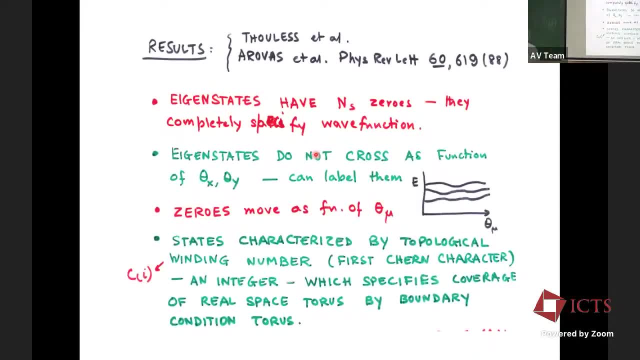 Let me tell you that's the actual, Actual reference, or over set up 88.. First, I can states have exactly that many zeros that are flux quanta through your sample And they completely specify the wave functions. the second thing that you can prove is that eigen states do not cross in energy as a function of theta, and the way to see that very clearly is: 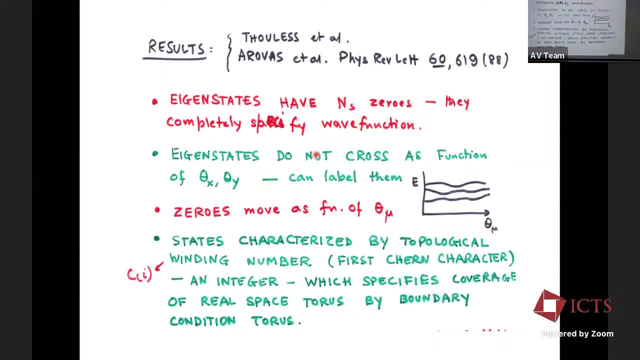 If two eigen values are very close to each other, you For some Tita X and Tita Y, you can forget about the rest of the eigen values. then you can sort of say one of them is here, the other one is here, and here's delta real plus I. delta I because it's a complex submission matrix. 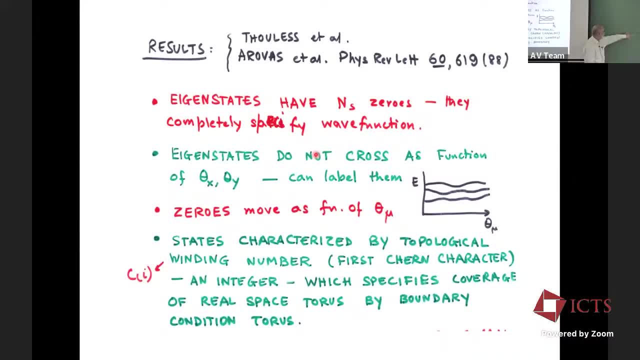 And the only way you're going to get to I in values to cross is: this has to be equal. these two must be zero, Delta R must be zero and delta I must be zero. there should be three conditions met, whereas we have only two parameters: Tita X and Tita Y. 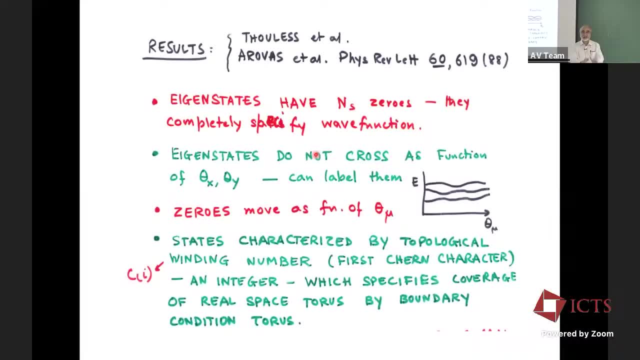 So generically eigen function, eigen values, will never cross when you change the boundary condition angle. If you change the potential also, then you can make it cross. but we are talking about eigen states in the given potential and so all of these eigen says they sort of look like like spaghetti as a function of Tita X and Tita Y, just like band structure does. 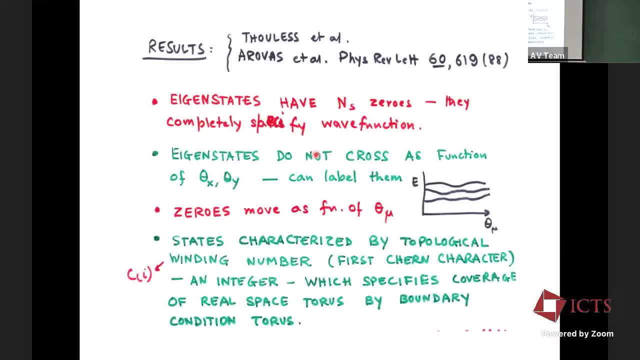 Okay, no Right. and that states then I characterized by a topological winding number. this is something that we've learned from after reading papers by David taulus, which is that's an integer which basically specifies the coverage of the real space doors by the boundary condition. 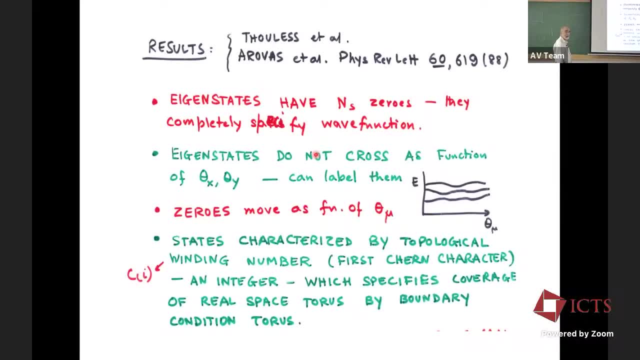 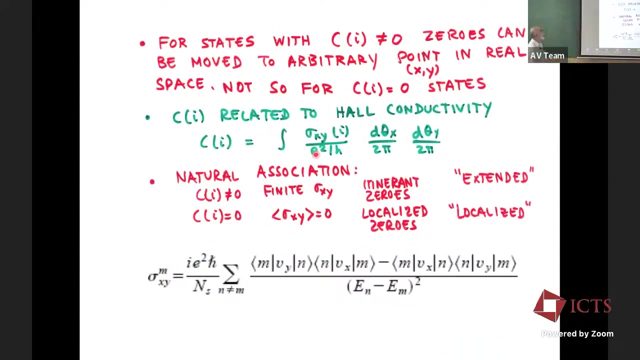 What Right? No, no, they won't, Because there are only two. Yes, If you change the potential, yes, they will, but if you fix the potential, they don't. they can't cross. generically, The other thing that we found, that the 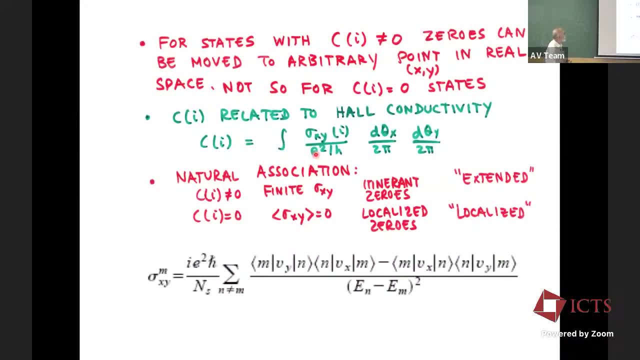 The For the states that have This Churn number Coverage Not equal to zero. And now we know that the number is nothing but the angle integrated average, all conductance of the sample. And we found that out The hard way. basically we we calculated the whole conductance and then we integrated over the over the boundary condition angles and we found we're getting numbers like point 9999.. 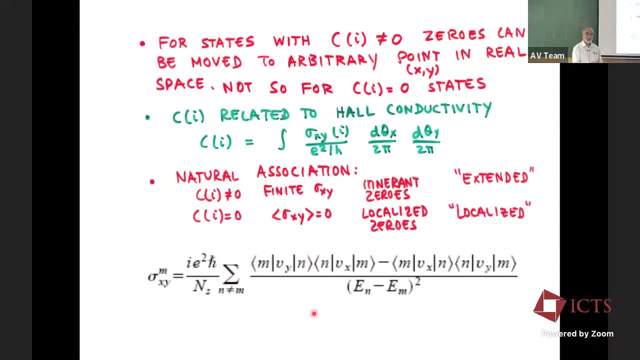 And we found we're getting numbers like point 9999.. And we found we're getting numbers like point 9999.. Seven and when, though, or three, or something like that, And so we realize that, basically that, that the integral, the average, all conductance. 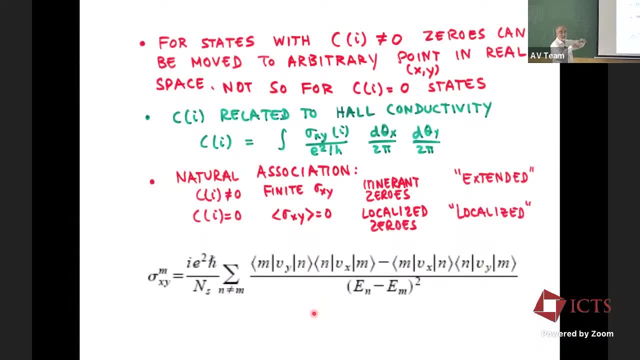 Of any given against it. The fact that they don't cross allows us to identify the DuTTs want to, and whatever the number of flux quanta there are, and so in. Sometimes there was a natural Association, But when the chart number is found, 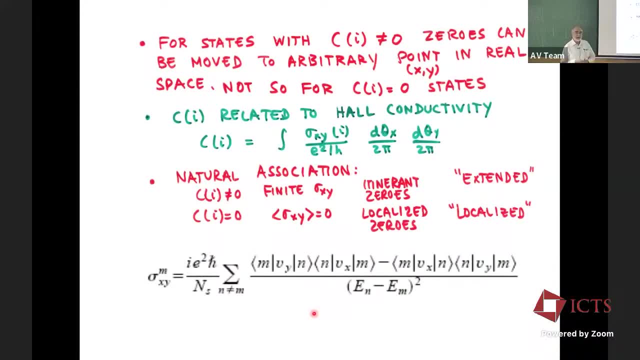 0.. It has a finite quantity. 3% in kelvin Indri productions, char н number is not zero. It has a finite quantity, con sticks to it, to the Hall conductance. It's certainly the average boundary condition. average. 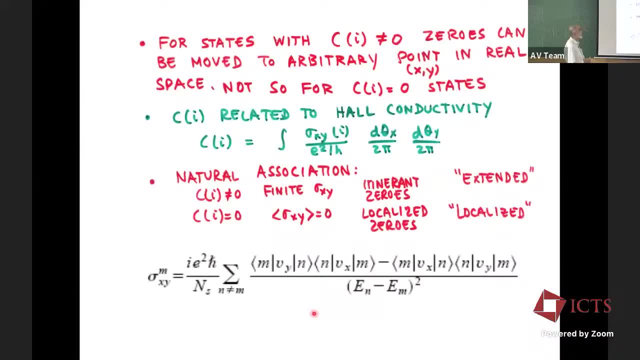 Hall conductance is a non-zero integer And you have itinerant zeros and we identified those states as extended and those that had your number zero were localized. I mean, yeah, you're right, I understand that this is a continuum problem case. 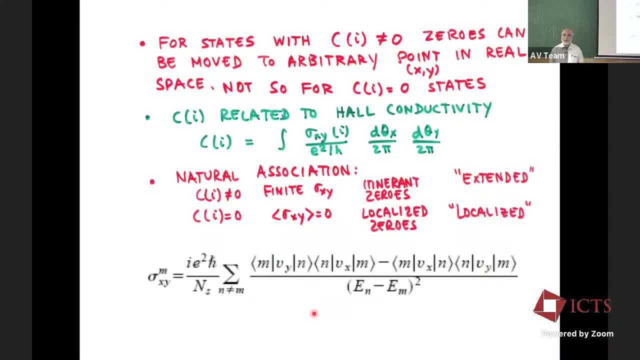 Right, exactly right. So you could probably do that in that case. Yeah, absolutely, With a disorder potential, right? Yeah, it wouldn't be momentum. You have to do the supercell. Yeah, yeah, Okay, anyway, so that's again. 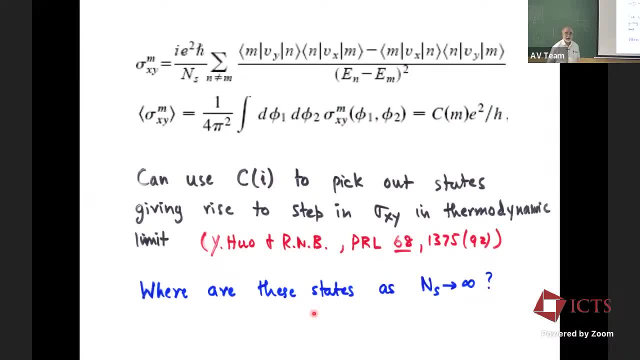 just writing out that the Hall conductance is a velocity-velocity correlation function and its average value in units of E squared over H is an integer. okay, So basically that's where it stands. That's where it's sat from 88 to 92. 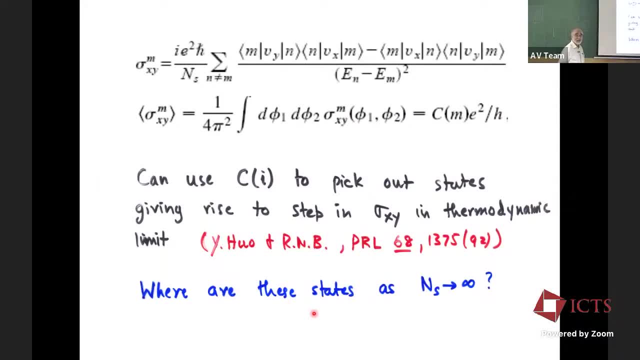 when I moved to Princeton, My first graduate student, Yan Hu, I told him: let's try and figure out where these churned non-zero states are in the band. Okay, And in particular, if we increase the size of the system? 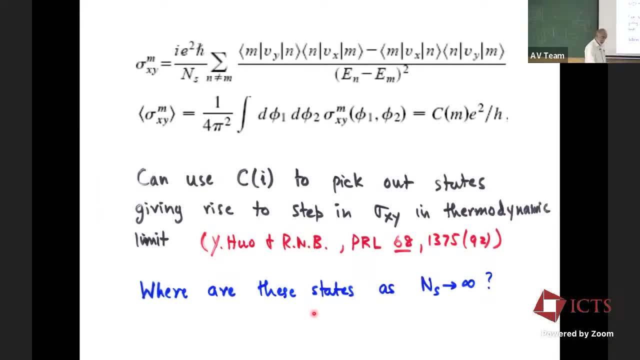 what happens to them, Where are they in energy space? And of course, you don't want to look at just one sample. You want to look at an ensemble average, because that's the only thing that makes sense When you're talking about a disorder problem. 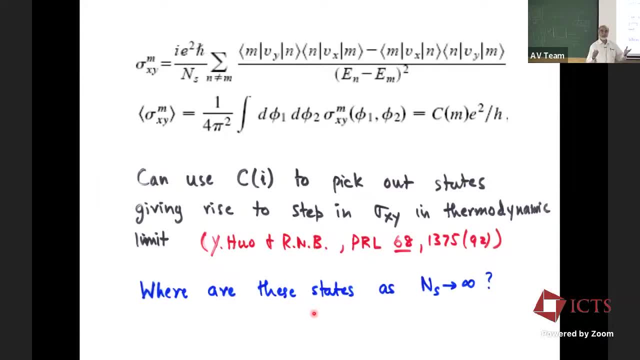 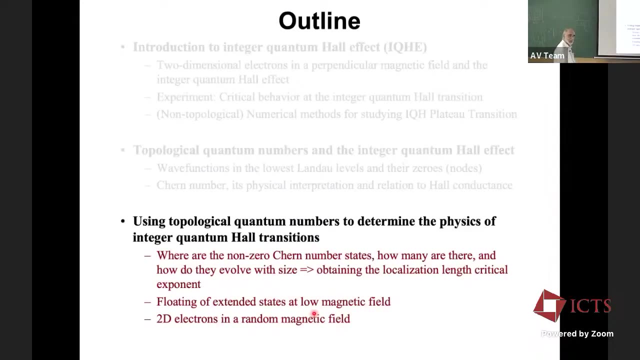 is that you want to see what is the density of states of churned zero states and what is the density of states of churned non-zero states, And I'm going to show you that data next. Okay, That's basically the work that my first graduate student, Yan Hu, 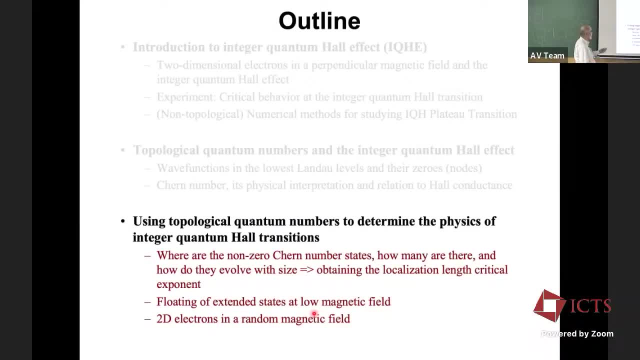 did at Princeton. We asked: where are these non-zero churned number states? How many of these states, How many of these states are non-zero? If you have a certain size of the system with n eigenstates, how many of them are going to be non-zero churn? 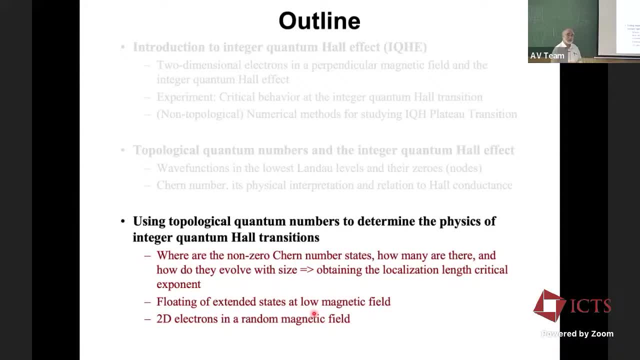 and how many are going to be zero Now, in those days, the assumption was that there was only one state with a non-trivial churn number. So the assumption was that if you had n eigenstates in each sample, there will be one state. 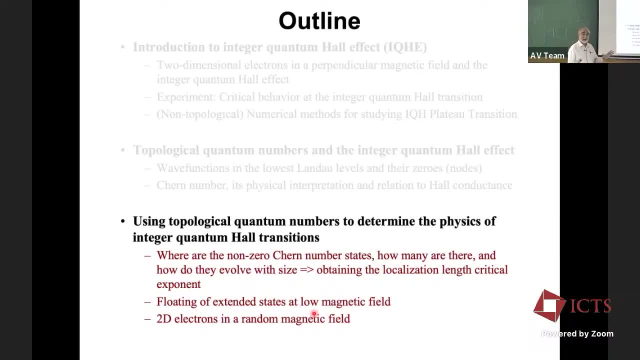 which has churn number equal to one and all the other eigenstates have churn number zero. Certainly was true for that sample where there were only one state with n eigenstates. Only one had churn number one and the others were all zero. But that's a very small sample. 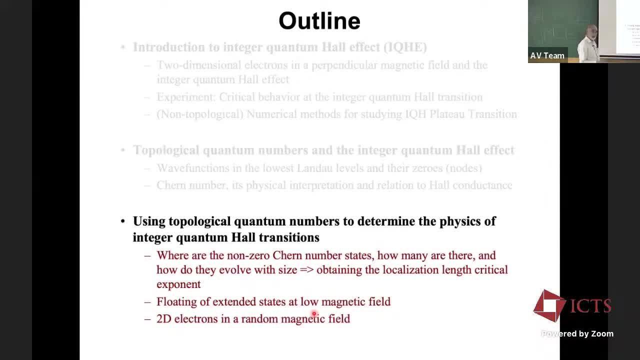 Okay, And then I will use the same method of calculating churn numbers and seeing where eigenstates are to understand something called floating of extended states at low magnetic field and also talk about 2D electrons in a random magnetic field. So those are the other two problems I want to do. 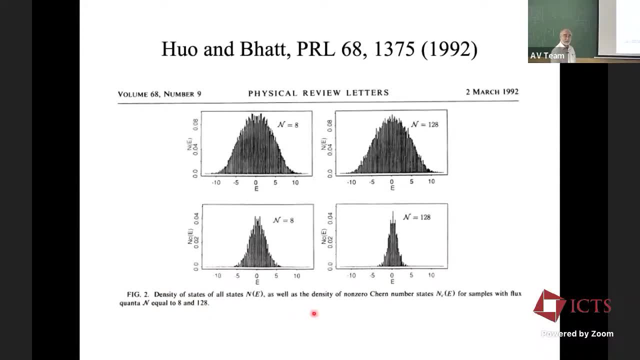 So here's the original, original work that was done. What is plotted here is the density of states, of all states, with a sample with eight flux quanta and another sample with the ensemble of samples with eight flux quanta each, And on the right is the density at the top. 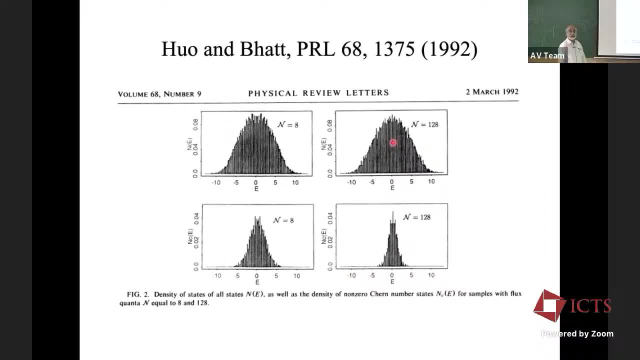 is the density of states for 128 flux quanta. So I think most of you can see that there's not much change in the density of state. There's no finite size correction density of states. that's really discernible, even down to eight flux quanta. 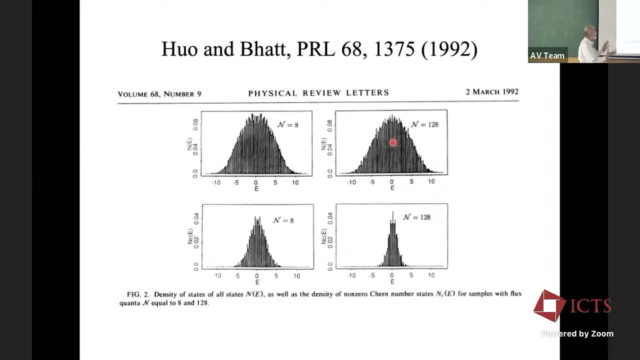 Maybe somewhere in the tails there are some issues, but it'd be. the central part looks very much the same. The next thing we did was find out what's the density of churn, number zero and not equal to zero, And we didn't sort of restrict ourselves to one. 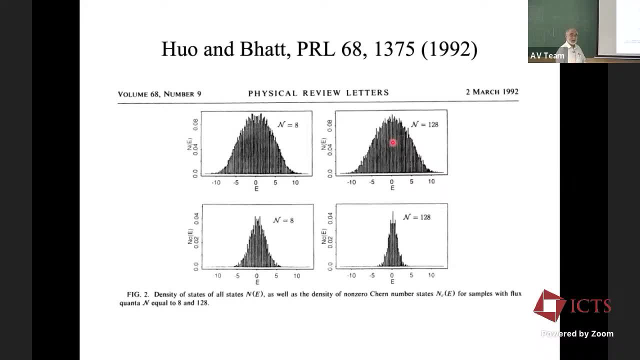 or minus one or two, or plus minus two, et cetera, because all that is required in the sum of the churn numbers has to be equal to one. So if there's only a single state with churn number, then it has to be plus one in it. 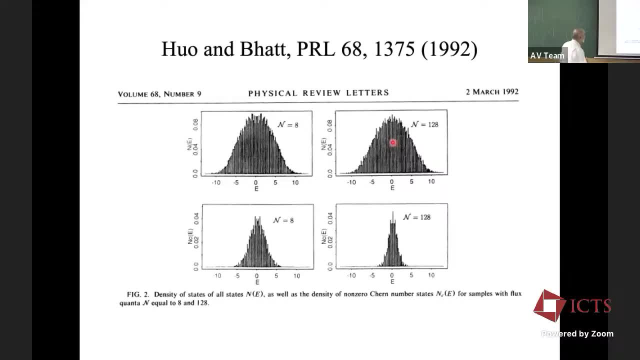 There would be only one for each sample. But what you find here is actually that the churn non-zero states are clustered around the center of the band, and they get clustered more and more narrowly as the size of the system goes up. So what I'm trying to say is that this width 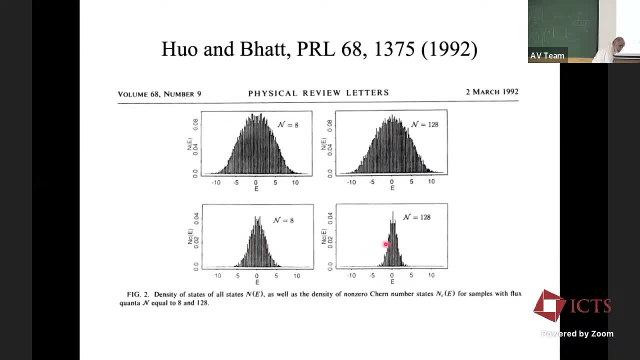 is significantly more than that width, And both widths are much smaller than the width of the total density of states- half width of the total density of states. So you can say: well, let's try and plot the width as a function of size of the system. 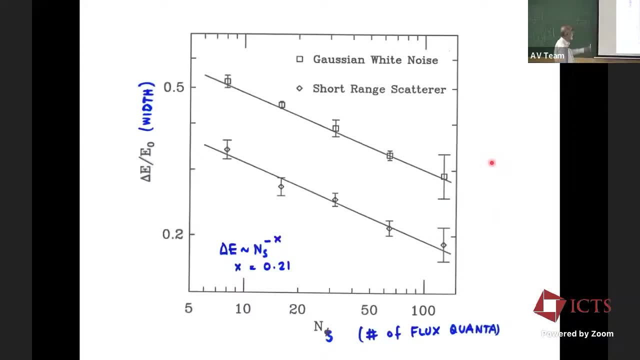 And that's what we did here: The width plotted against the number of flux quanta on a log blog plot, And it seems we tried two different kinds of random potential. One is Gaussian white noise, The other one is short range scatterers that have been sprinkled. 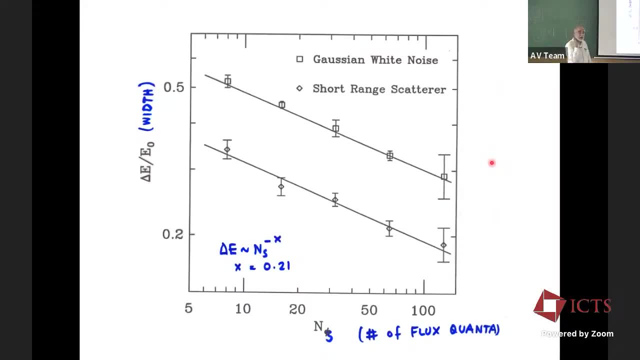 And while the actual numbers, of course, differ, because the two potentials are very different, And what we find is that the slur, the slopes of the two lines is pretty much the same and the slope is 0.21.. Now, if you remember the slope of the curves, 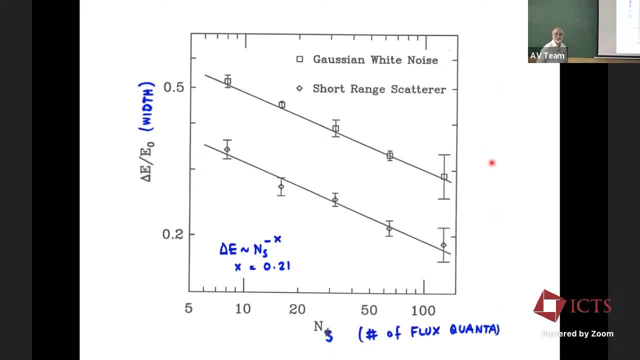 in the experiments was 0.42.. So that's very suggestive that there's something going on here, which is there's some relationship maybe between this X that I have and the Kappa that the experiments got okay. So what's the argument? 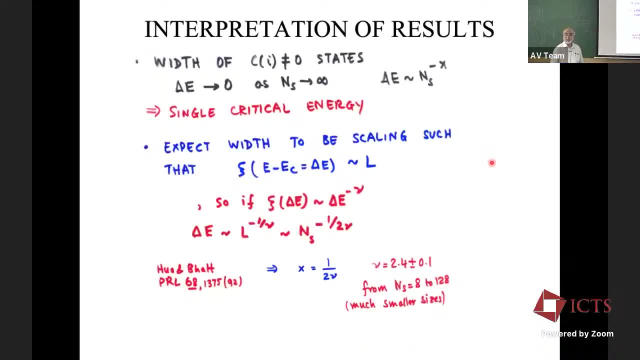 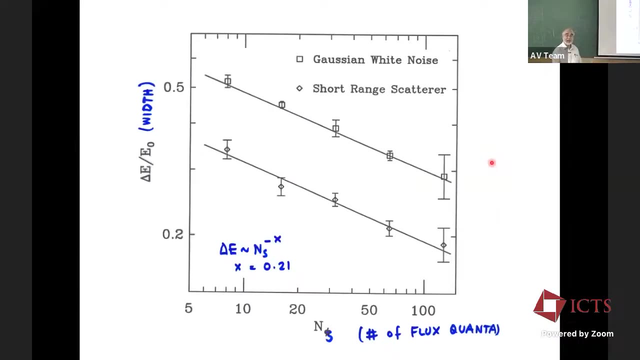 Okay, basically, what we're saying is that this X is measuring the localization length exponent, And the argument is the following. First of all, the data are consistent. It's not saturating. In those days, there were people who claimed that there was an extended band. 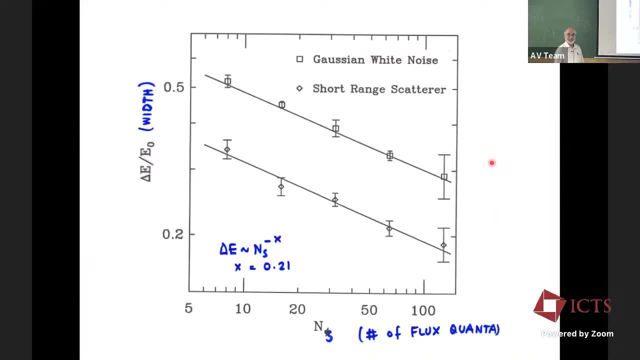 because some people did some Hartree-Fock theory and stuff like that And they were claiming that there was an extended state band and all that stuff. So this shows very clearly that the data are consistent, with this width going to zero in the thermodynamic limit. 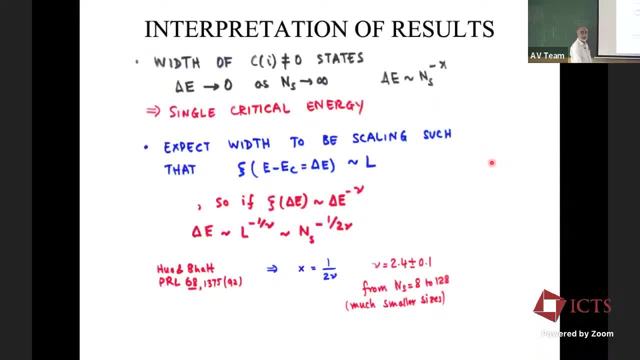 So there's only one critical energy which is at the center of the band, because we have chosen the problem to be electron-whole symmetric. White noise is equally positive and negative And when we put short-range scatterers we put equal positive and negative amplitude scatterers. 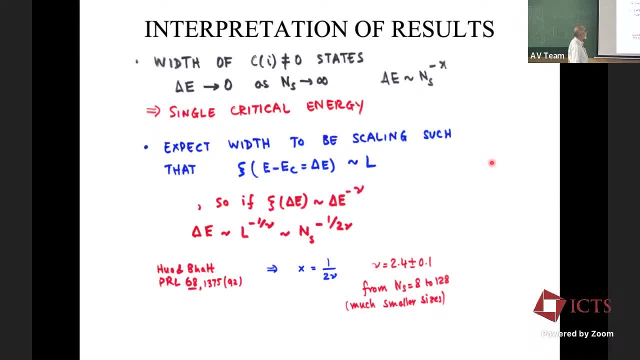 Statistically equal number. okay, Now what do we expect the width of this non-zero churns band to be? And the argument is that we expect that if we have a finite size system. we expect that if the localization length is of the order of the length of the system or bigger. 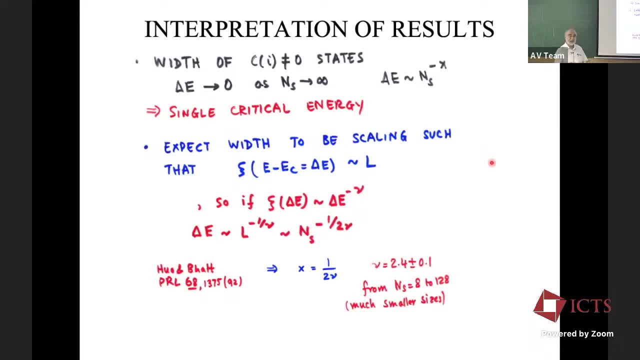 then the system cannot distinguish whether it is localized or extended. So the localization length or the length of the system is going to be larger than the length of the system. So the localization length is going to be larger than the length of the system. 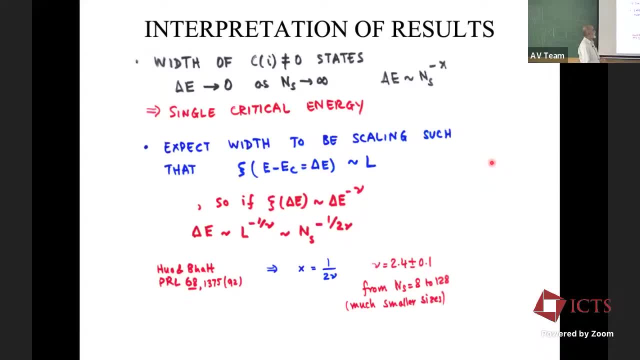 length at some energy Delta E. whenever it gets to be equal to L, that will be the width of my churn band, the churn nonzero states. so if I assume that psi varies as energy to the minus nu, that is just exactly this formula right there. then that tells me the Delta E must go as L to the minus 1 over nu, because I'm 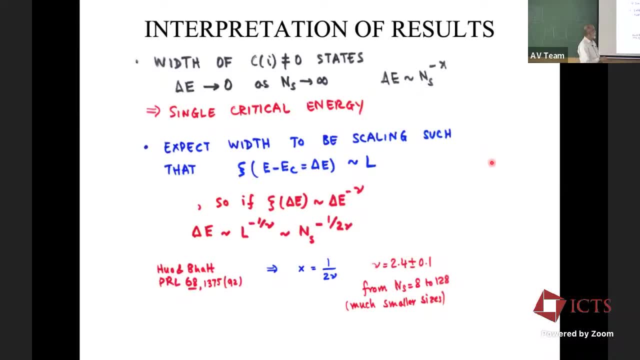 putting that equal to L, and so it must go as number of flux quanta to the minus 1 over 2 nu. so if X is 0.21, then I can get nu from there. it's equal to 1 over 2 X, or 1 over 4.42, which is 2.4, with an error bar of 0.1. 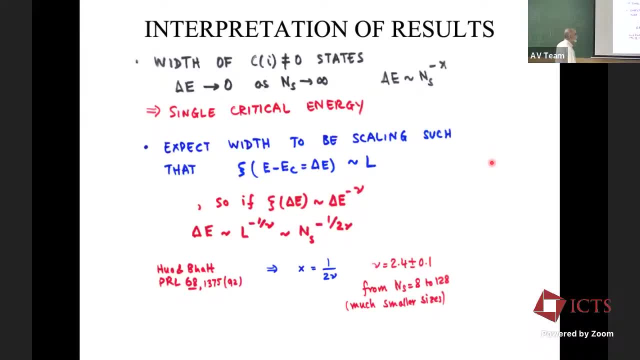 that's what we figured. so it's very small sizes compared to the data that was that has been done in the past, The data that has been generated for these widths because we have number of flux quanta 8 to 128. so if you want to sort of think about it, it's basically, you know, 3 by 3 to 11 by. 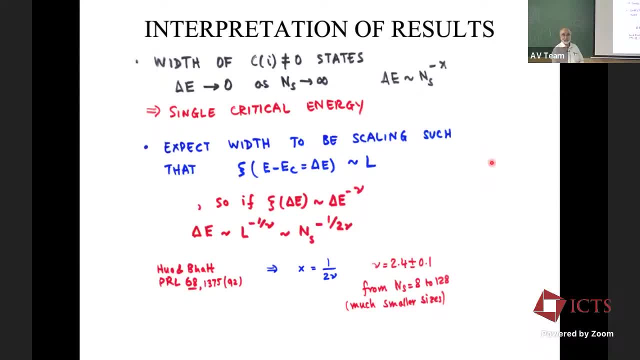 11 or something like that. that's the size. of this is very small sizes, and the data get 2.4 and actually, as you can see, the number has gone up. when they did a better job of analyzing their data. We are already getting a number that is higher than that- somewhat higher, though it's within. 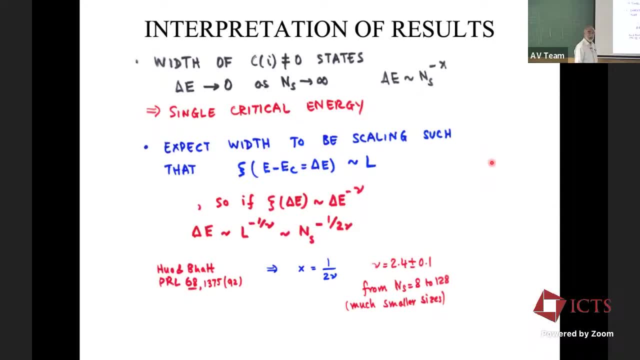 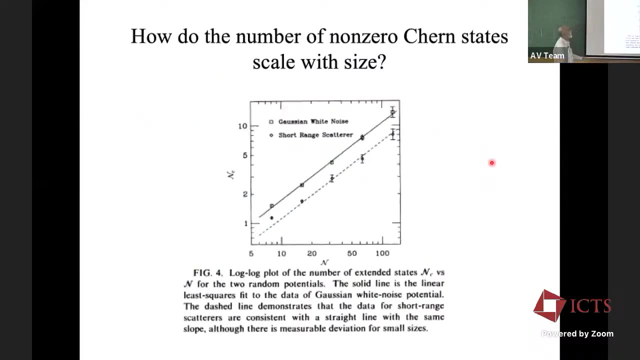 the error bars. so I'm not going to make any claim for it. but if I'd use those kind of size widths in my strips I would have not even got a scaling function problem. it would have had wrong behavior at small energies. And how about the number of non-zero charge states? we can also count how many. 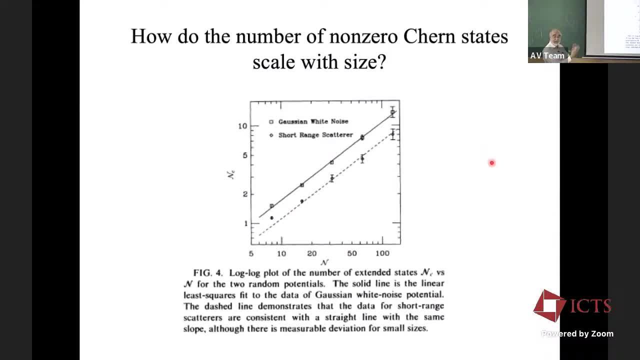 of them there are, and because the width is shrinking and the height is roughly remaining the same, we expect that actually that number will be sub thermodynamic. So if you look at this, this plot, it is roughly n to the 0.79. it's 1 minus that 0.21. that 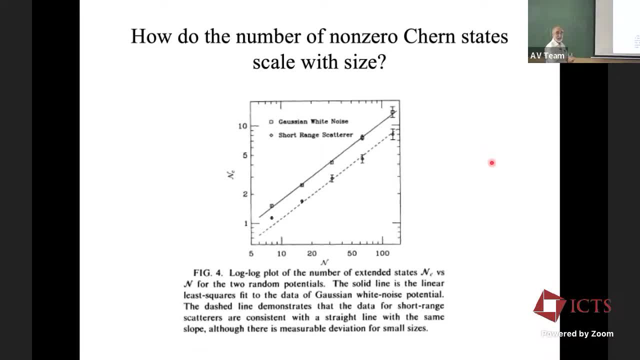 we had for the other one. okay, so it's saying that there is not one topological state for large sizes, it's a sub thermodynamic. in fact, the number of topological states is as the sample size goes to infinity. goes to infinity also, but not as fast as the sample. 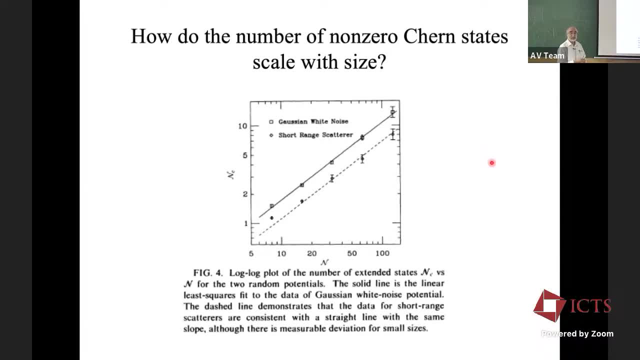 number size goes, which sub thermodynamic? and in fact the sub thermodynamic tells you that there is a localization that is diverging. okay, no, there's no, no proof of that. but people thought that that's what? because, because it is happening At one energy, they thought it was as specific and eigenstate. but that's not true, it's, it's. 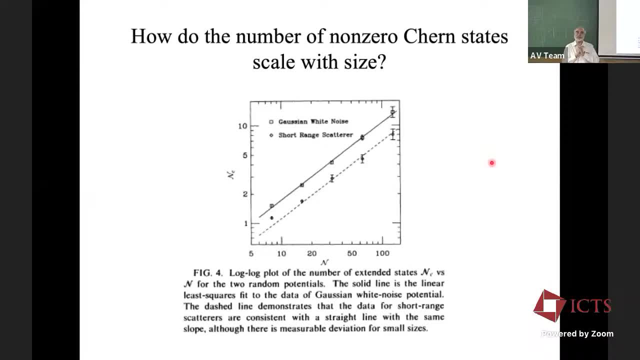 it states within a small energy window around the center and that energy window is going to zero in the thermodynamic limit. but it is finite and and how it's determined is basically by saying that for a finite size system the localization length at that energy scale is: 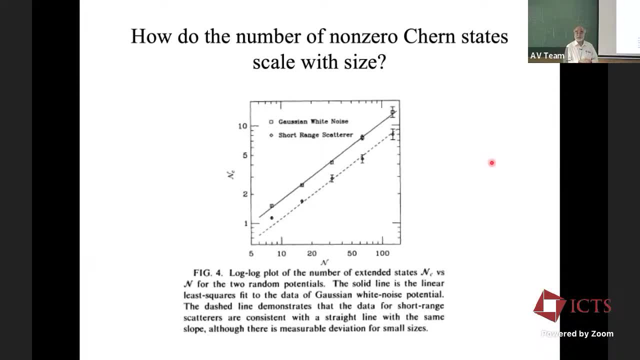 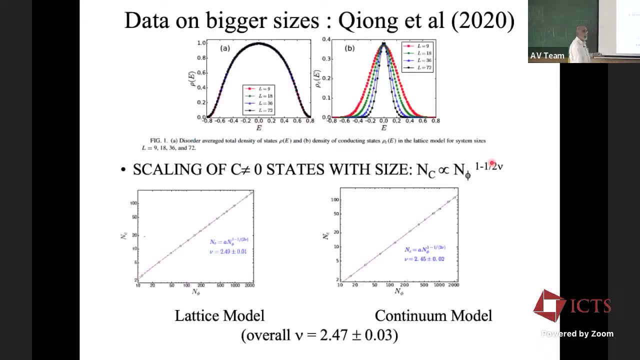 exactly equal to the length of the sample. Okay, Much better work was done by another student, or one of my students, chung, only a few couple of years ago. he did it both for the continuum model as well as for the for a lattice model. okay, just to check whether it was. it was different for a lattice model with flux threaded through. 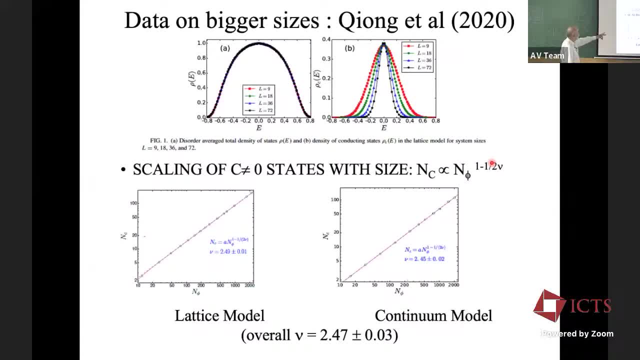 it And Again. So here we are plotting the number of churn not equal to zero states with this number of flux quanta, double logarithmic plot, going from flux quanta about, you know, 12 to over 2000, 2500, I think it is in both cases. so it's a factor of 20 in flux quanta or factor of 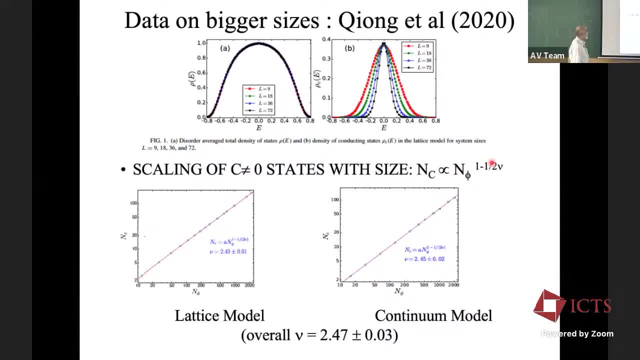 five in length, scales roughly and of course he is now doing some statistical analysis of the data and then getting error bars based on that. I have a suspicion about that, I don't. I don't like using law of large numbers so easily, but anyway, this is. these are the numbers. 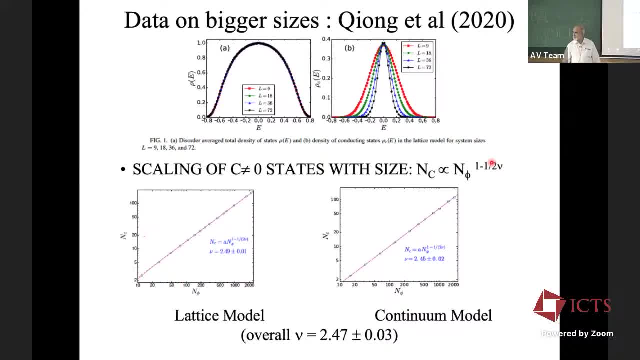 that he he gets. Don't touch NC versus n. This is 2.49 plus minus point or one for this set of samples, I don't, you know. don't take this point or one too seriously, nor should you take that other point or two too seriously. 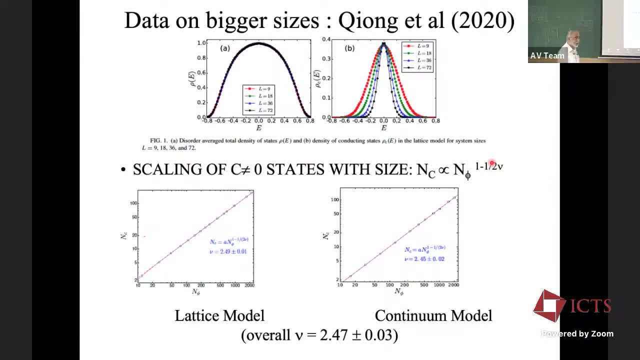 that the two should be the same. so clearly, if I took it really seriously, I would say the error bars don't overlap My. my own thing is: if someone gives you a very low error bar multiplied by three, if they give you a conservative error bar multiplied by two, then you're probably in roughly right okay. 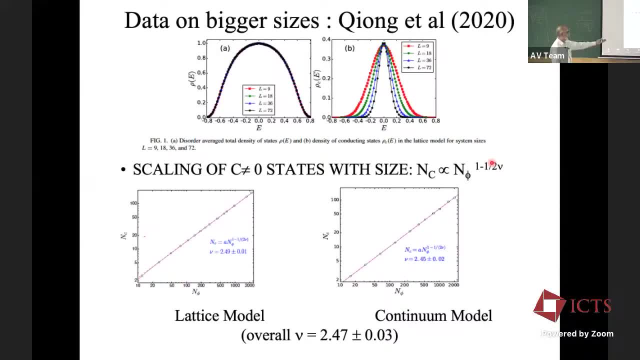 So I would say that this is suggesting that it is. I mean, between those two you can fit the both of them by saying it's 2.47 plus minus point or three. but I would say I don't think it's point or three. it's not 1% accuracy, is probably two to 3% accuracy. 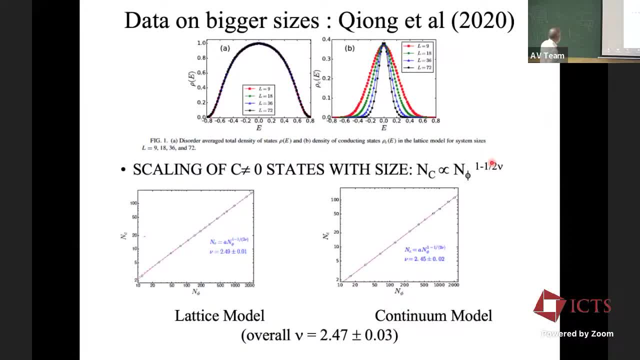 Now whether one should make a big deal about the fact that this is not equal to the one there, I don't know, but I do think that this- the fact that for very, very small sizes it was 2.4.. With an error bar of point one. 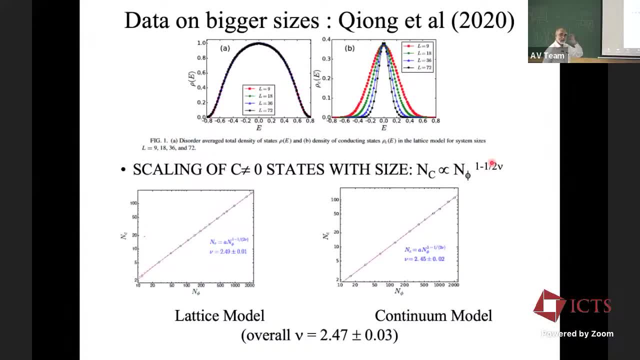 And With big sizes, and we still haven't changed that much is within the same error bar. Okay, it is telling. I mean I have more faith in this than the other one. and the other reason I say that is because, sorry, if you look at this curve, okay. 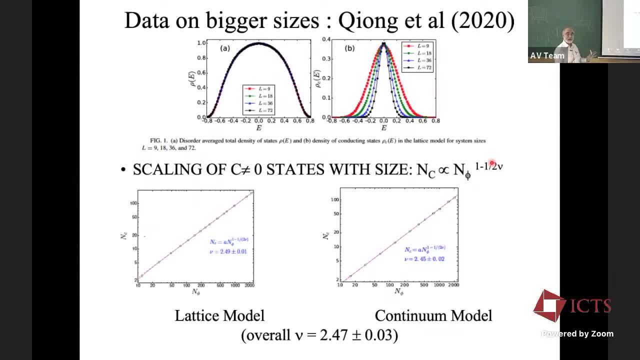 On on this log log plot. it really looks straight. I mean you, I mean I. I tend to look at it from sideways and see whether there's any curvature in the in the plot, to see if there are corrections or not. And we also did put in corrections. 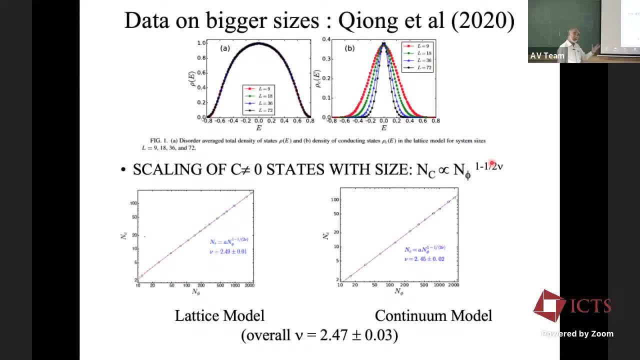 Okay, and when you put in corrections, you find that whatever corrections you put in a quantitatively very small. so you're putting two extra parameters, a coefficient and an extra exponent, Okay, and you do the best job of fitting everything. of course, new changes a little bit, but not not all the way to 2.6. it changes by like one or two in the last. 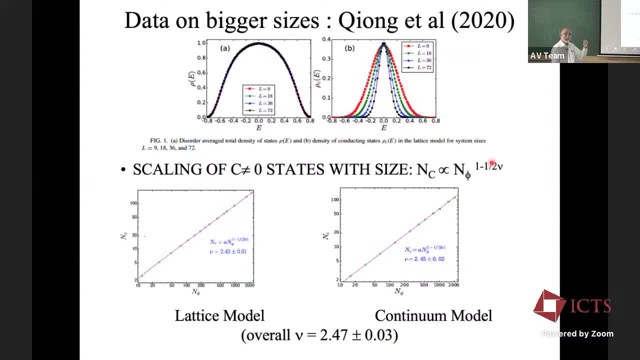 digit. And The reason it does Is because the coefficient of the second term is very small and the exponent, the, the sub leading exponent, is large, so it's minus two or minus 1.5 or something like that, when, whereas if you look at the, the analysis of the strip method, it's point four or point. 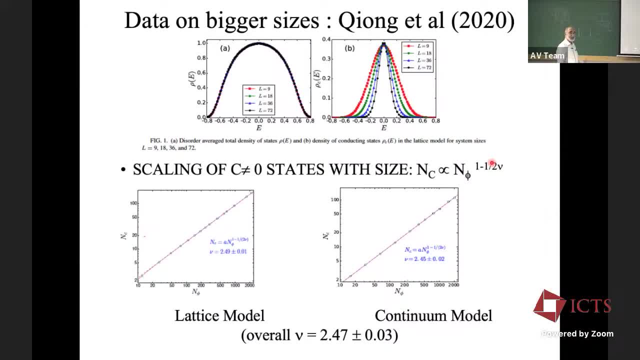 two. Okay, so that it's saying that there are lots of corrections in these strip method and here it doesn't look like this. that many corrections, Okay. So this is a mystery which needs to be solved. I'm not going to claim that this is the right answer. 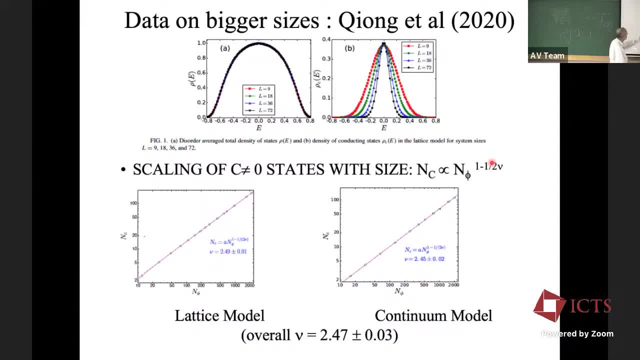 But I think that this needs to be looked at. these are that on the right, at the top of the density of states for different sizes, And I think he has done I'm not, don't quite remember this, but these are thousands and tens of thousands of samples. 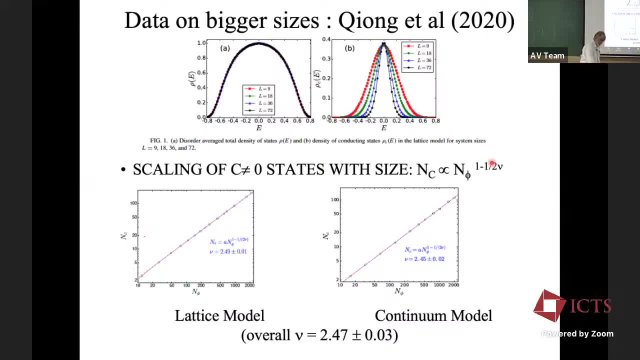 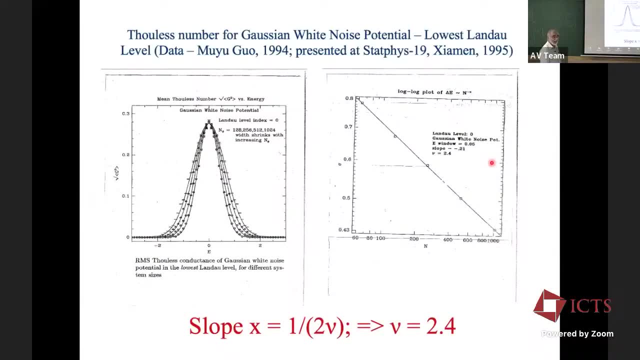 Average. Now, what I mean by that is that this is very simple, but from the point of view that you get a very different set of random states And then you go through and it's going to be very simple to understand What you're thinking. you're going to get a sort of set of random states. 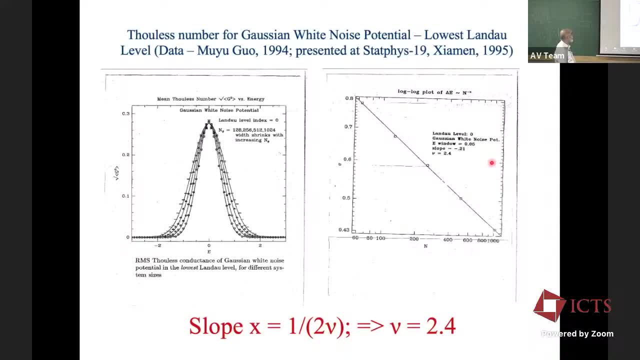 So it's going to be a little bit like a very simple carefully, I'm going to be looking at a very simple set of random states. It's going to be a little bit like a small but it's going to be anti-periodic boundary condition and see how much the eigenvalues move. 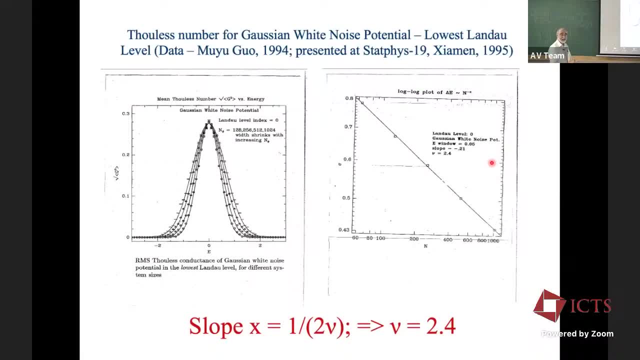 relative to the average spacing of eigenvalues, and that defines the Thouless conductance, if you remember the formula from lecture two. and so he plotted the Thouless conductance. It's called the RMS. for some reason. he decided he didn't like taking an absolute value. 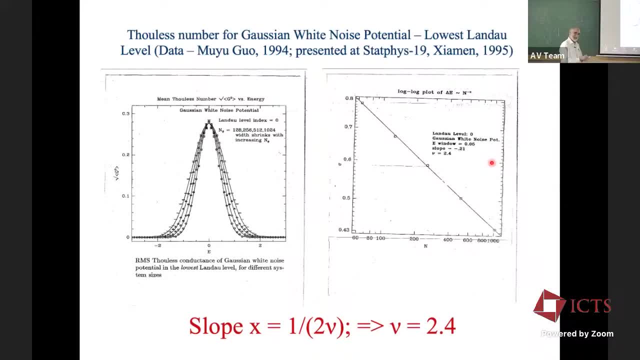 So he squared it up and and took the average and square rooted it and things like that. But again the same thing that it is collapsing near the center of the band, saying that the, that the in the thermodynamic limit, the conductance is only finite at the center of the band where there's an extent where the 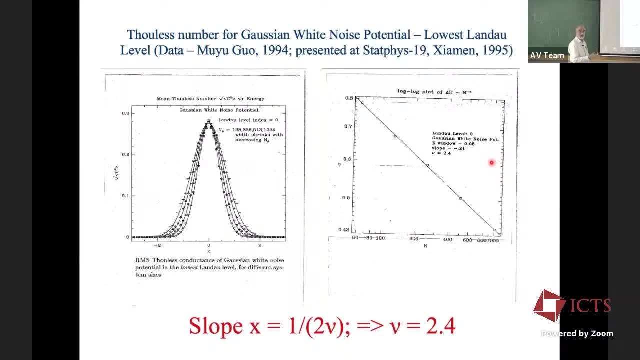 Localization and diverges everywhere else. the conductance is going to zero Because they are localized states and by plotting the width as a function of n he's able to get that, and the slope is again 0.21, suggesting somewhere around 2.4 again. 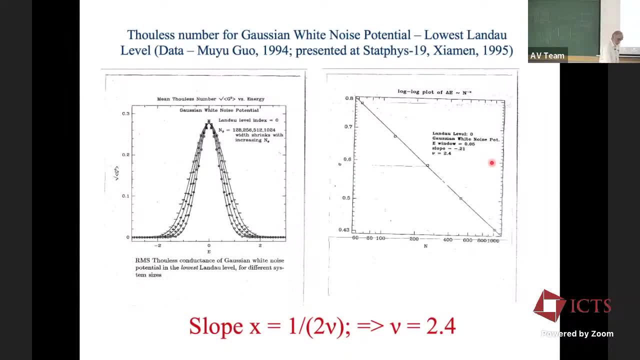 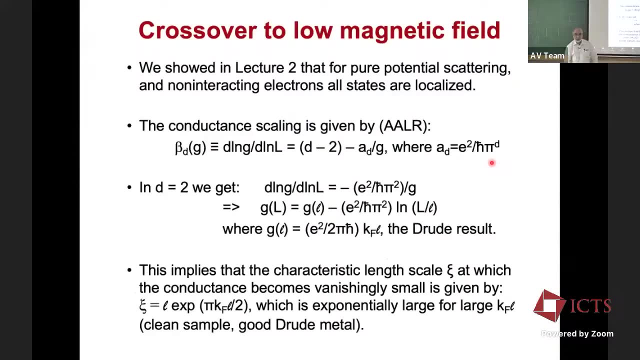 I don't know the error bar here, but it's sort of comparable. So What I'm trying to say is that there are different ways of doing numerics to get an answer, and I think it's very useful to have a situation where there are two very different methods. 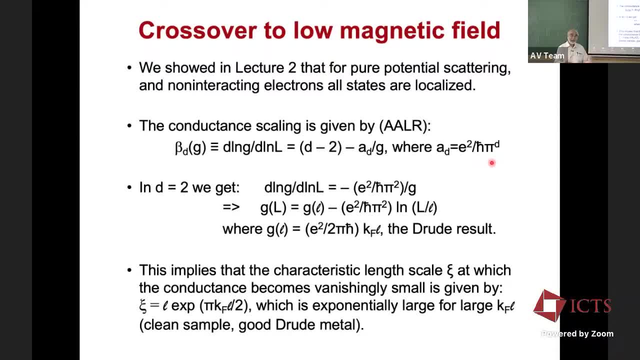 To get the same answer, then you can. if they give the same result, you can trust it. so to the extent that You know, for example, we can trust that answer is 2.47 or 49 and 2.58 or whatever it is. that is the latest number are you know? they are certainly within. 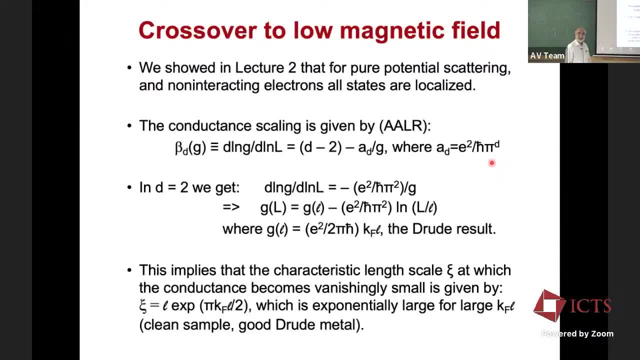 Within 5% of each other. so we can certainly trust that answer to 5%, but we I don't know whether you can trust it to 1%, not just yet. So another thing that you can do using these churn number methods, basically identifying what are the 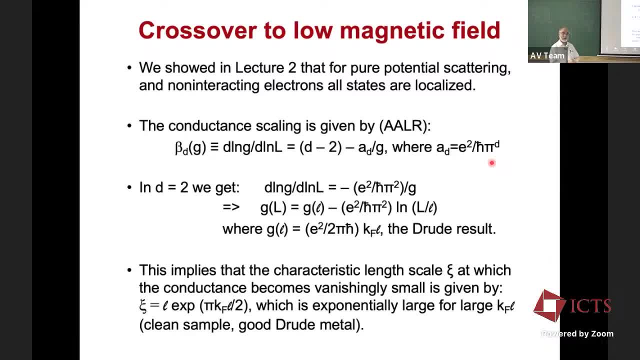 What are the extended or current carrying states? and in the quantum Hall regime is you can try and understand the crossover to low magnetic field. So let me try and motivate that in lecture two. when we didn't have any magnetic field, just two dimensional electron gas with potential scattering, one of the results of the scaling theory was that there is no metallic phase, it, it flows to insulator. okay, and for 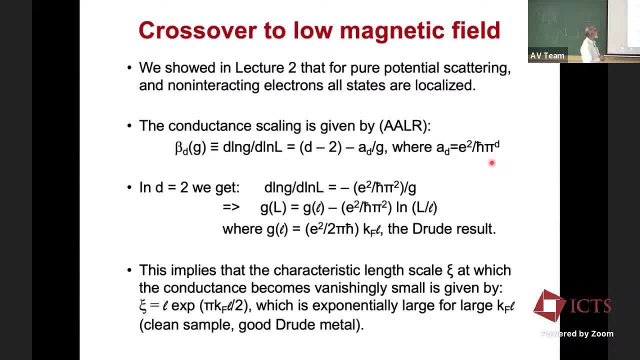 small. For large conductance you can develop perturbation theory which, which is basically here, it's given by the beta function. the Logarithmic derivative of the conductance with length scale is given by D minus two, minus some constant over universal, constant over G, and for D equals to you, just the first term vanishes. 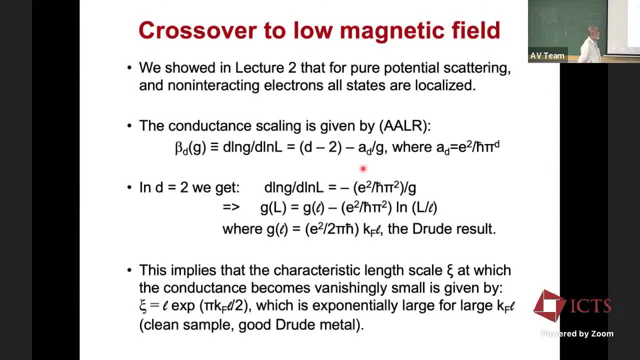 So you can just write down the conductance of the function length, and we did that in lecture two and showed that the conductance at a large length scale is the conductance at the microscopic length scale minus a universal number multiplied by the log of. 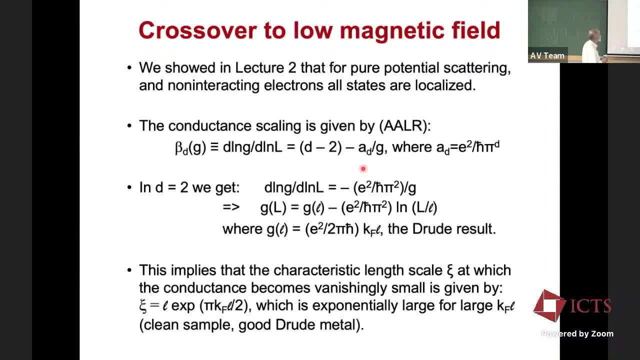 capital, L over L And of course g at the microscopic length which is the mean free path, is just the result which, in two dimensions, is e squared over two pi, h bar times kfl, And kfl is supposed to be very large. You're talking about a metal with very few defects, so the 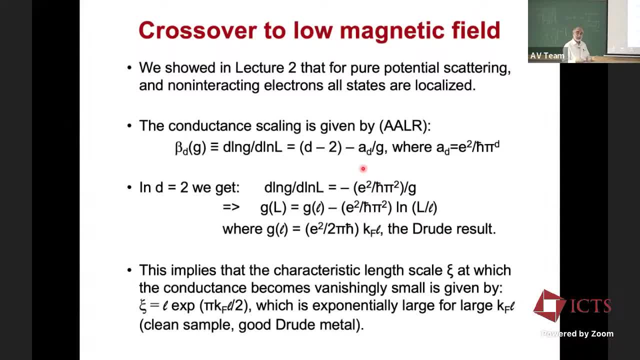 mean free path is supposed to be very long, whereas inverse kf, that is the de Broglie wavelength, is microscopic. So kfl is a very large number. So one expects that g of little l is quite big And it'll take quite a long length before the logarithm is going to catch over and make that. 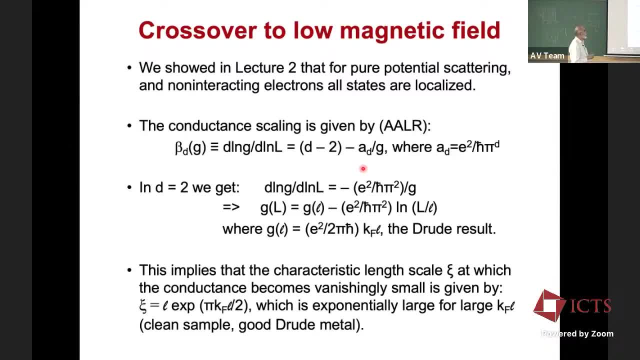 thing zero. So if you sort of say that, well, at some length scale xi, the conductance becomes vanishingly small. using this low, you know, perturbative result, you find immediately that xi is just put capital L equal to xi and put the left hand side equal to zero and you'll get xi equals. 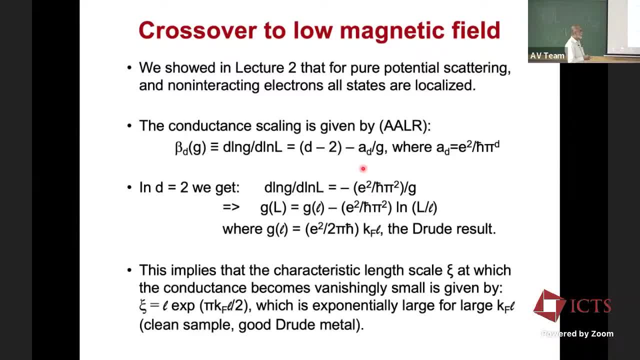 L exponential of pi kfl over two. And since kfl is supposed to be much bigger than one, pi over two, kfl is also very much bigger than one and its exponential is exponentially large. So basically it's saying that for weak disorder, 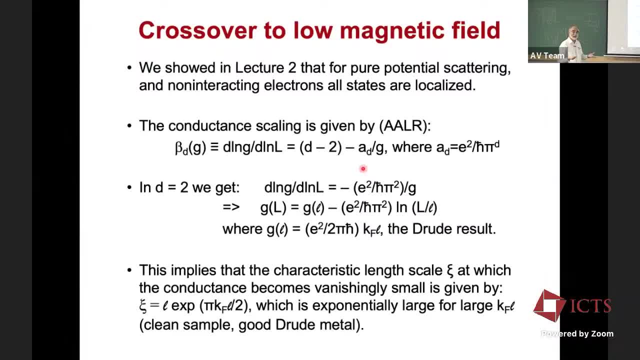 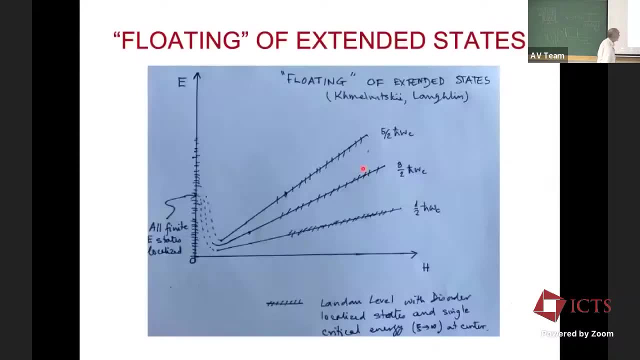 you have very long length scales, localization lengths, but every state is localized, even though they are localized over long length scales. So let's try and understand how these Landau levels, when you go to lower field, what happens to them. So that is a hand-drawn figure that I made two days ago. It's basically, if I look at the energy. 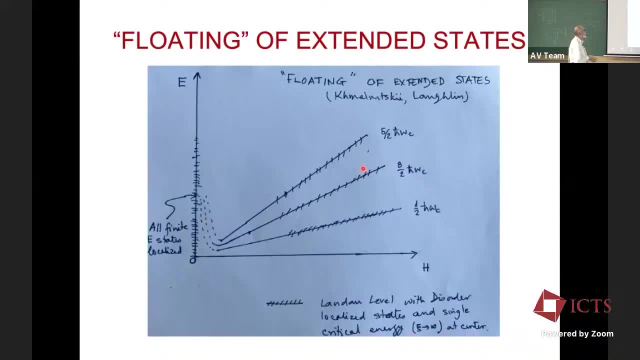 versus magnetic field, then each of the Landau levels is at n plus one half h, bar omega c. omega c is proportional to h, so they're just straight lines going through the origin. okay, So these are the energies of the lowest Landau level, as a function of field. 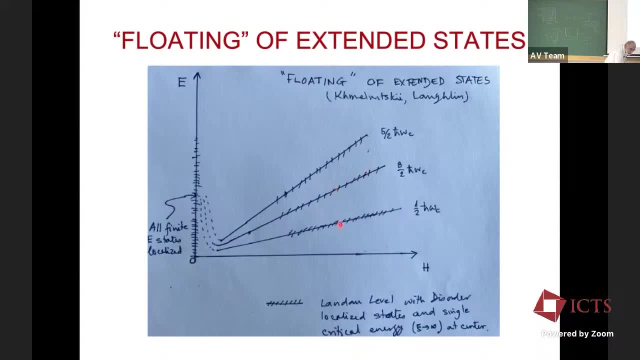 this is the energy of the second Landau level, or first Landau. this is the zero, this is the first, this is the second, et cetera, et cetera. This is known as the Landau fan diagram, basically. 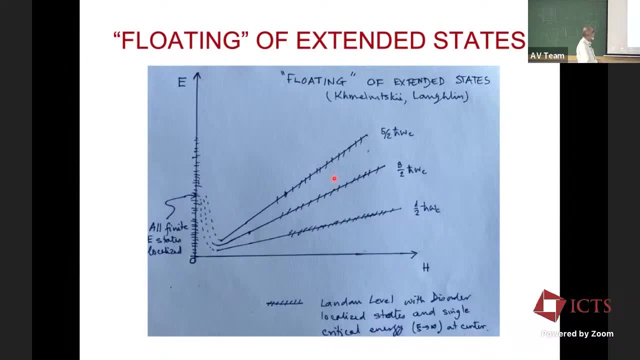 And I've sort of put hashes there to say that it's really broadened by disorder. okay, which a disorder doesn't depend on magnetic field, so the width is the same. So when the splitting between these Landau levels gets to be a part of the disorder width, 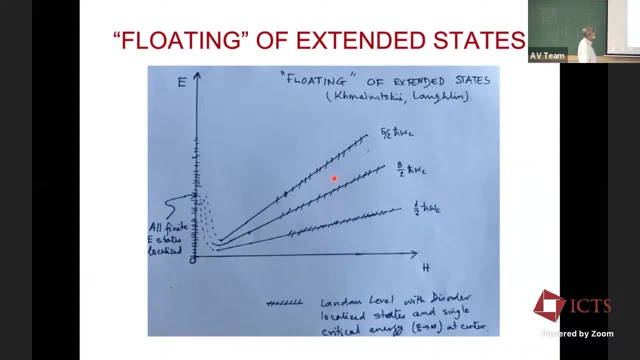 something else will happen Now. one other thing that was pointed out by Malnitsky and also by Laughlin was that we know that there is a extended critical energy inside each of these Landau levels where the localization length goes to infinity. We just saw numerical evidence of that. 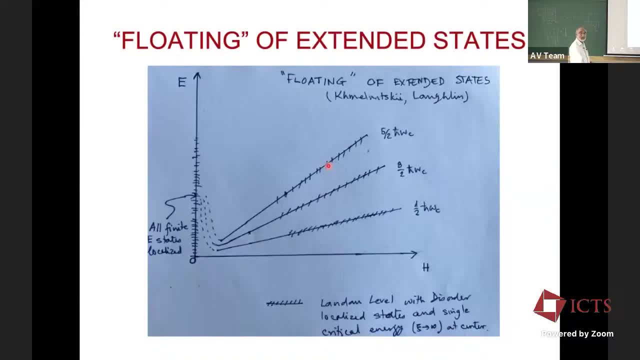 So what happened to those infinite localization length? We know that, out at zero field, all the states at finite energy are localized, even if they have exponentially large localization, and they're still localized, which means the only way that can happen is that this middle of the band, which is this, extended states. 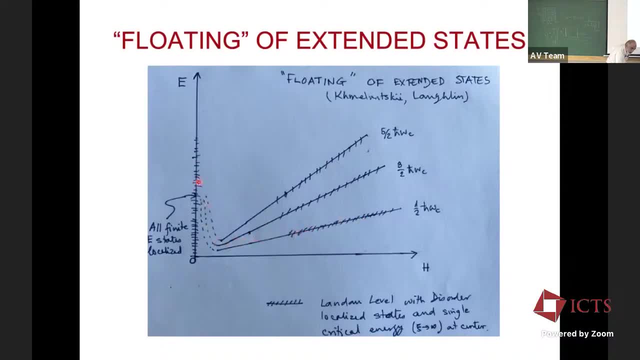 those are not equal to zero state. they must be going up to infinite energy as you go to zero field. That's the only resolution of that. They carry a topological quantum number. that cannot be. you know, they all have plus one. 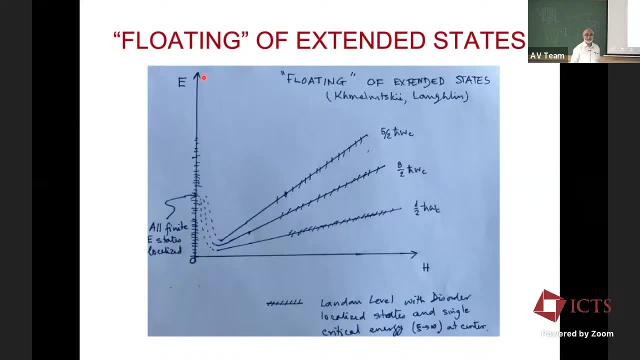 Plus one plus one never gets to zero In a, in a tight binding model. of course, what happens is that there are there are negative Chern number sub bands which will, which will cancel the things, but nevertheless, this was the idea that if you are very close to a free electron problem, you should see some floating of these critical energies. 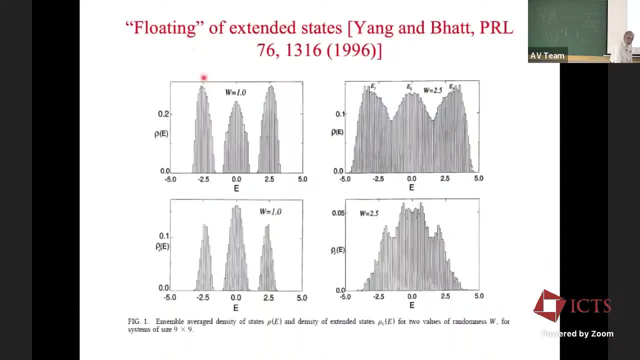 So we actually tried to do that and we did that. this is with Koenig-Kloss- He was my postdoc- and what we did was we actually did a tight, binding model and in this tight, binding model it has a central band and two side bands and you can think of the two side bands as Landau level, basically the first Landau level, and and what happens is that you should think that this is zero, the lowest Landau level, and that's infinite energy, and that's infinite energy. 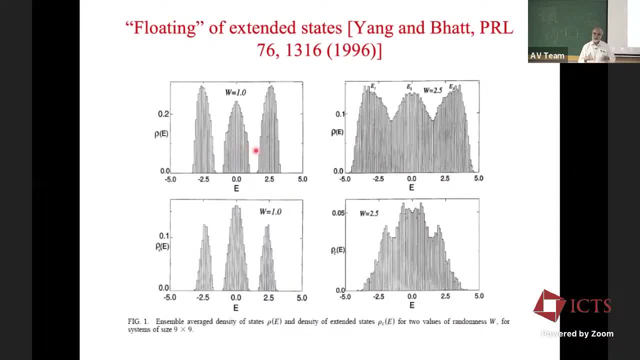 And that's on the other side of infinity, if you can make more sub bands if you want. but the data are most conclusive when you're just one Landau in this problem. Okay, And so this is the density of states, of all states, at a disorder strength of w equals one in some units, and this is at disorder strength of 2.5, and the lower panels tell you the density of Chern, not equal to zero states. 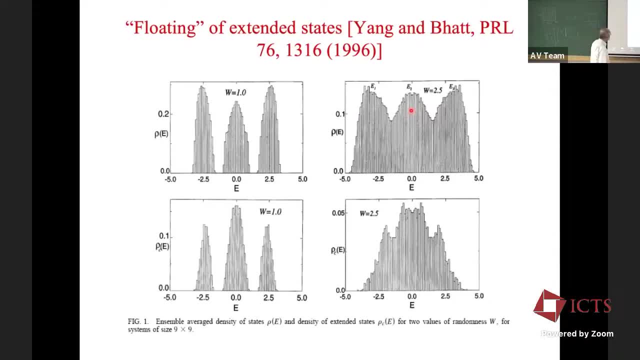 And what you find is, of course, for small disorder, the Chern, not equal to zero states are in the middle of the Landau band, So I'm trying to say that this one is at the center, in the middle of that. it's got a slightly smaller width than that, But when you go to this larger disorder, what you find is that this, this energy, is actually not the same as the energy of the full of the lowest band. 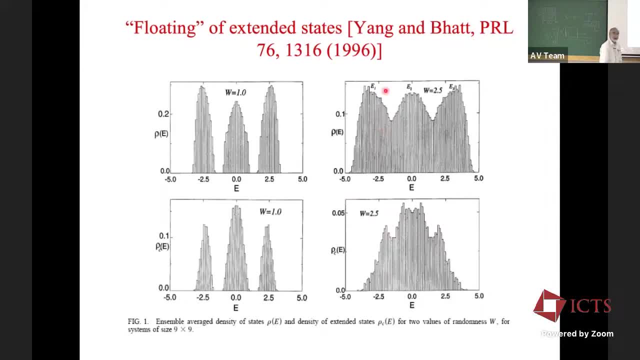 In fact it's quite a bit different, It's quite a bit higher. it's somewhere there. So the critical energy which is represented by Chern, not equal to zero states, are actually floating relative to the rest of the band. So the so there is evidence of this floating that was conjectured by Khmelnytsky and by Loflin. 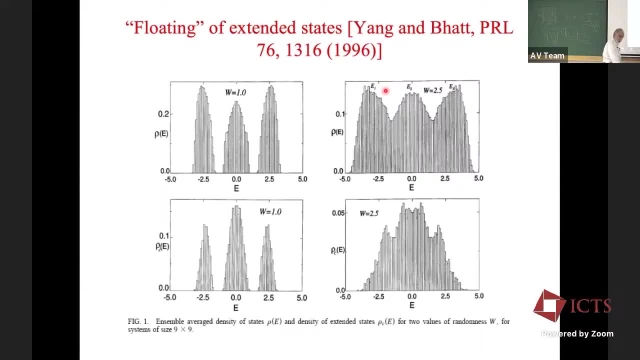 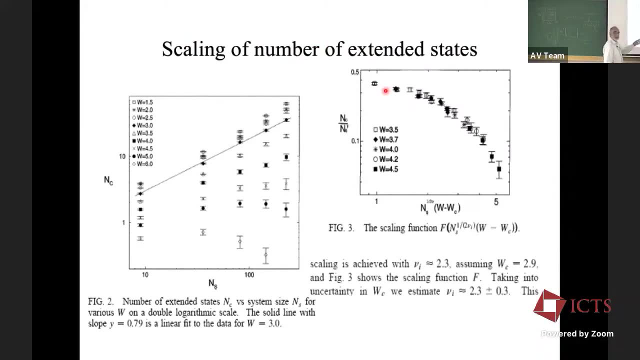 So that's another way, another thing that you can use this method for Okay, And you can actually scale the number of extended states. I don't want to go through that. Then you can do a full scaling of of this And again, all the data sort of depending on the localization length, gives you the right. 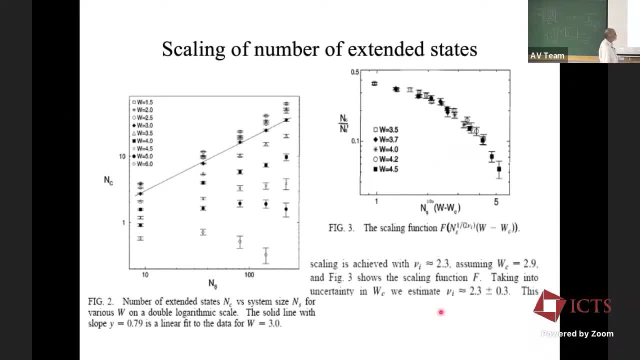 right, you know, gives you one single scaling plot And that depends on the exponent that you use, and best is achieved with exponent of 2.3.. Okay, here the error bars are much larger because you can see it's. 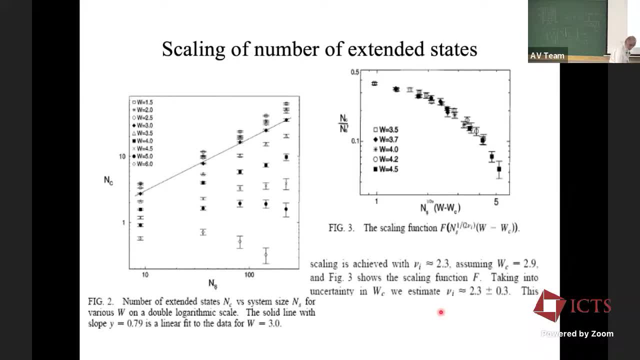 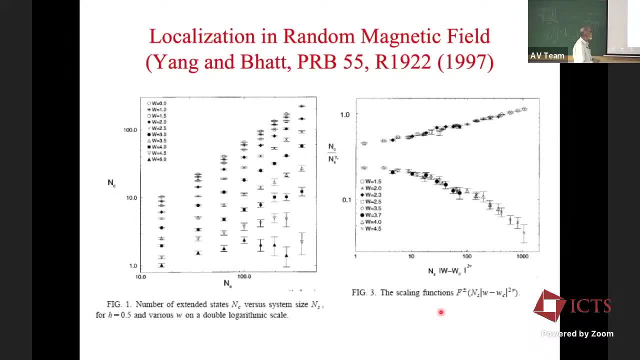 it's a little bit more messy, it's not as clean as a single Landau level, And you know, okay. Finally, I want to just mention one more problem that you can do- because you can do numerics- is you put a random field and then ask yourself how many states are. 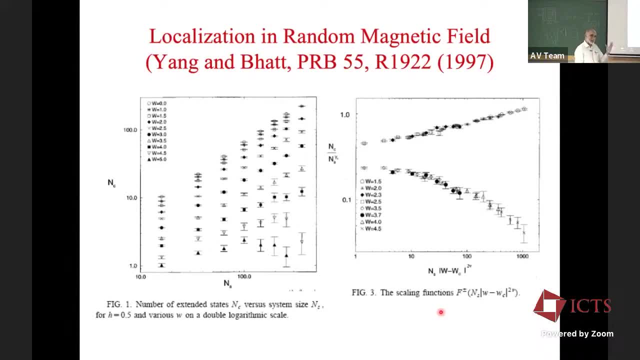 So this is a system in which you take a tight, binding model, you put fields up and down, equal with equal probability, and then you calculate the Chern number of each of the eigenstates And you see How many non zero Chern states there are as a function of total number of states for different energies and different disorder strengths. 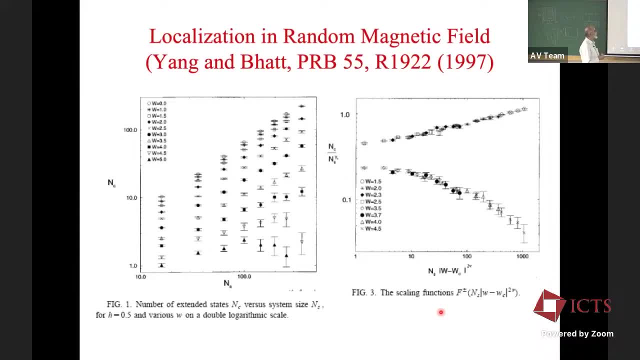 And what you find? the upshot of this is that the best data collapse seems to suggest that there are two branches to this curve, not one, unlike the case of uniform magnetic field, suggesting that there's at least the data are more consistent with there being an actual extended band. 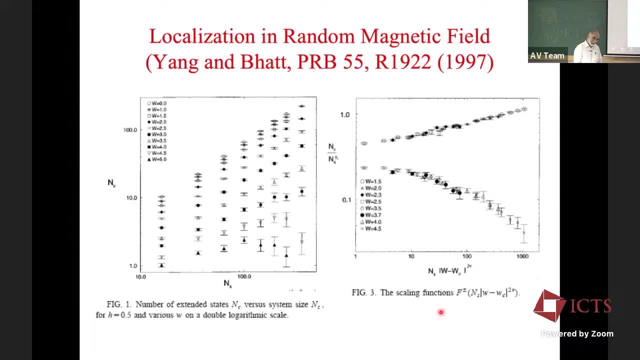 Okay. Now there is a very valid theoretical reason to believe that, to treat this numerical result with suspicion, and therefore I also want to, You know, show that you shouldn't just take numerical data at face value. It turns out that if you have random magnetic field, then you do the beta function. you get one over G squared instead of one over G, and that says that the localization length instead of being exponential. 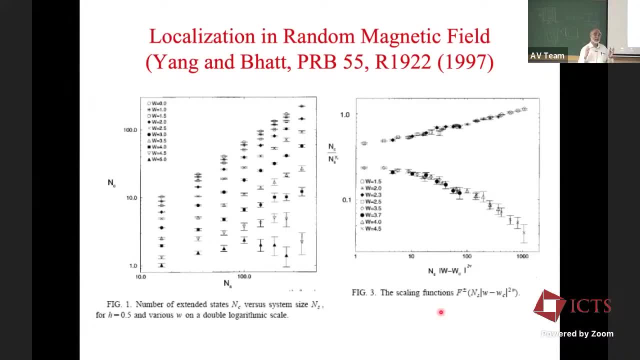 In KFL are actually exponential of KFL squared, so they're huge. so the kind of sizes we can do are tiny compared to the supposed, You know, localization lens that you would expect in this problem using the field theoretic or scaling kind of analysis. so it is quite, you know, it's not unlikely that something that diverges so rapidly at the at 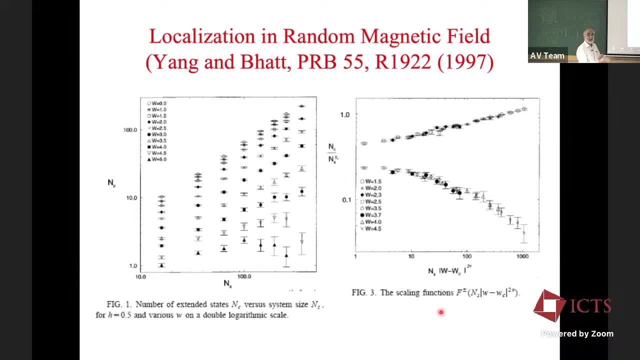 zero energy looks like as if it's diverging with the finite localization and I mean find that power or divergence at a finite energy, which is what this is suggesting. So you have to take that with a pinch of salt. Better numeric has to be done. I don't know whether that has been done since you know this- this was 25 years ago so- but I don't think anybody's really. 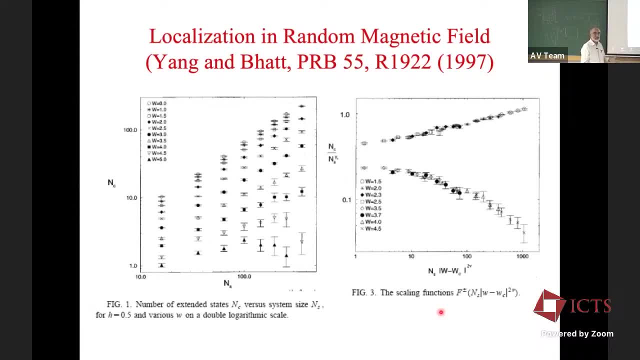 When, when you see that the scale is going so rapidly, as a numerical person you have to sort of say that this is not the problem that numerics is going to solve. this is going to have to be solved using analytic arguments, and the numeric can only help the analytic arguments if they cannot. 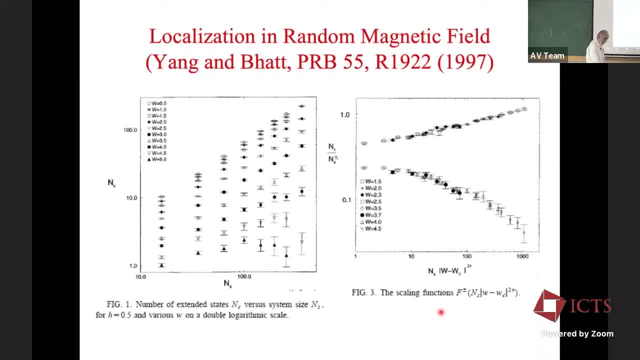 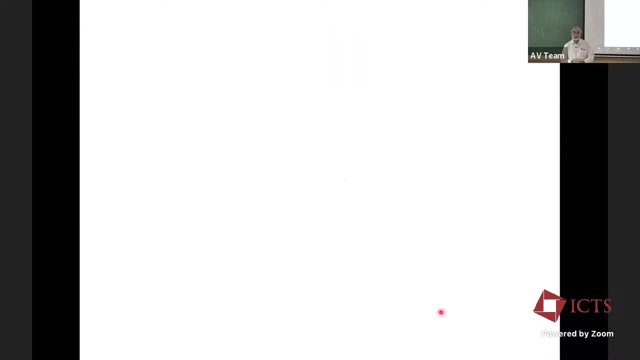 They cannot, You know, be the primary way to. on the other hand, if you want to look at the localization length in a, in a finite magnetic field, in a land of level problem, They are certainly very good At getting that. Okay, and with that I want to finish for today and I will continue tomorrow with talking about 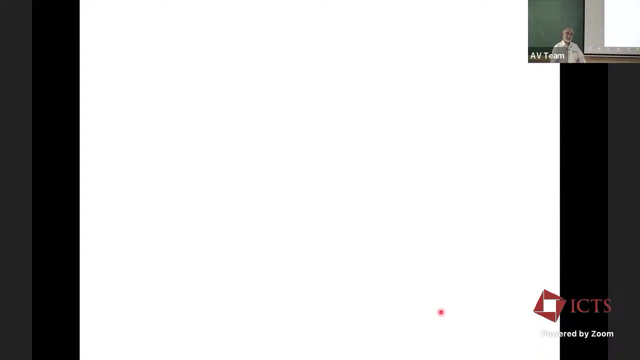 fractional quantum Hall effect to localization transition and then finally many body localization for an interacting system. so tomorrow- i'm sorry, thursday's lecture, final one- is going to be about interacting electrons and what you might access to contribute to that. So thank you, Thank you. 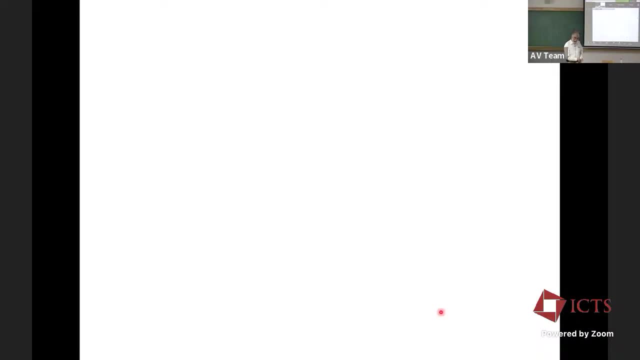 I. my own feeling is graphene has Both plus and minus, so so I don't know if I can answer that question. It is both plus and minus, so so I think that that would be. that would suggest that it's. It sort of depends a little bit on what the churn numbers of each of the land of bands. all right, because 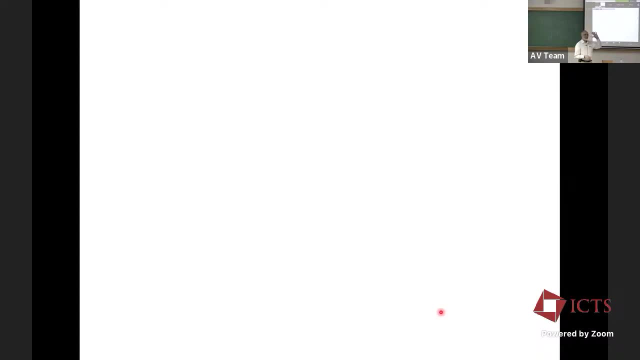 In for the simple parabolic case. they are all plus one, With direct this person, the central one is Different. If they're all positive churn number states, then of course there's no way to cancel them without getting them to plus or minus infinity in energy. 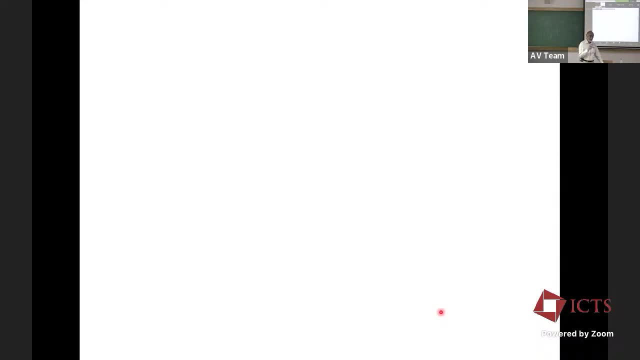 But if you realize that all of these things are actually in a lattice. so we're only talking about physics on the length scale of the magnetic length, which is on the order of 70 to 100 angstroms, whereas lattice constant is two angstroms, right. 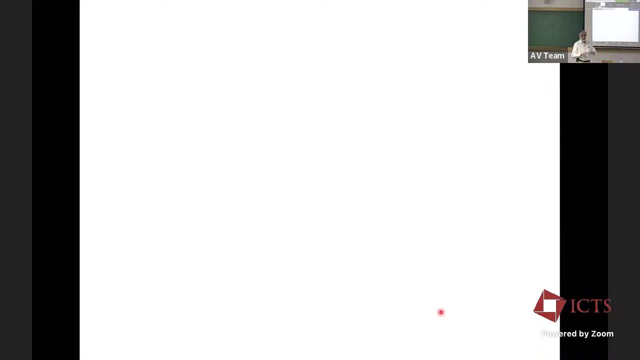 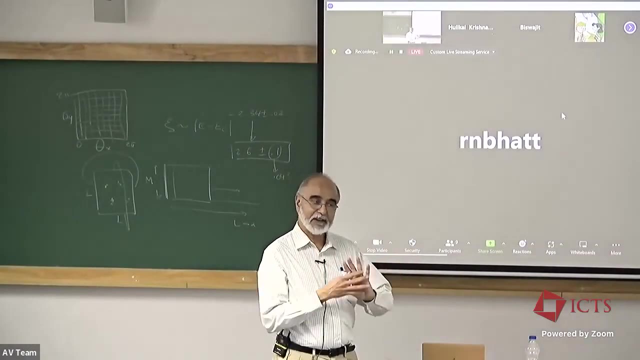 in the nearest neighbor distance. If you start with a tight binding problem, then what happens is- and let me not talk about graphene, let me just talk about ordinary gallium, arsenide or something like that, but I assume that the band curvature changes. 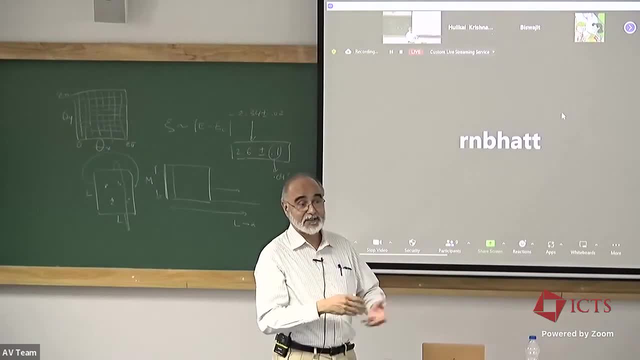 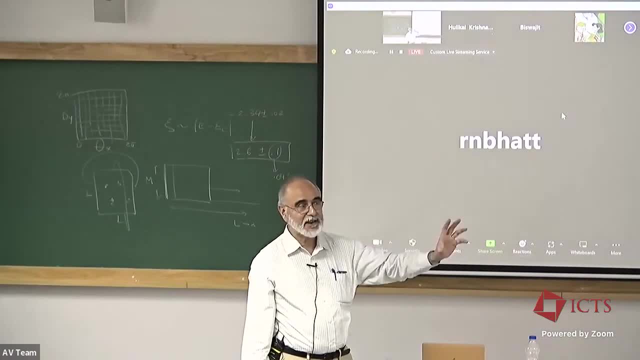 and then there's plus one from the other end, and then there's a central band that has exactly the negative churn number of the sum of all the others. And so what happens when you put disorder is the central band tends to broaden and come down. 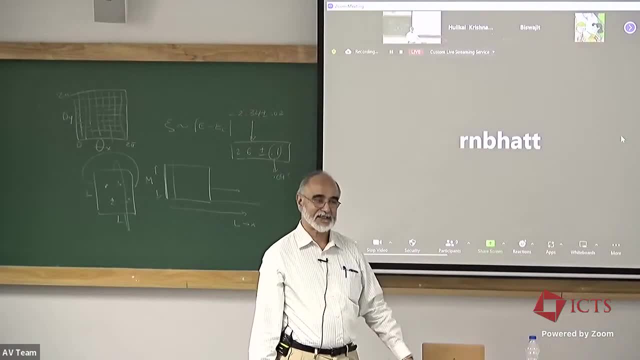 and eat up the churn numbers of all the bands. So I think it is probably true that the lowest, at least in the normal case, p squared over, p squared over two m- the lowest Landau levels do levitate, but maybe not the others. 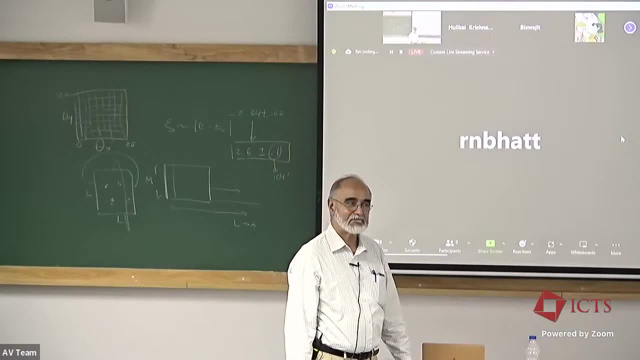 I mean, before they levitate, they get eaten up by the well, I don't know. If you strictly talk about the continuum, it's a singular limit. That's the problem, right? I don't know about the graphene. 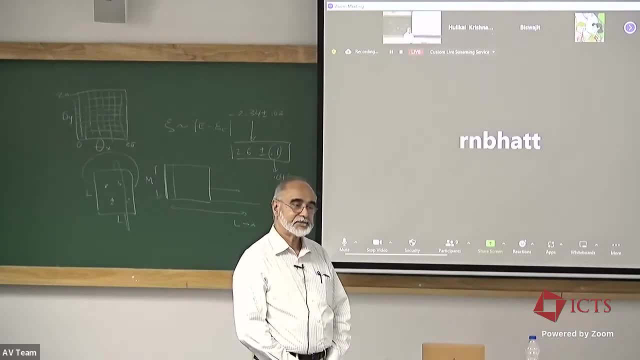 I haven't thought about it, but that's a really interesting problem. Yeah, So if I don't do it at, say, zero-mean bands, but at small-mean bands, Right, Right. So what is the possible scheme with respect to this K-f-n to K-f-n squared type of? 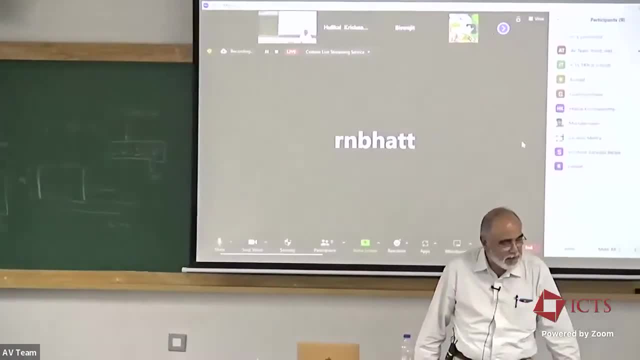 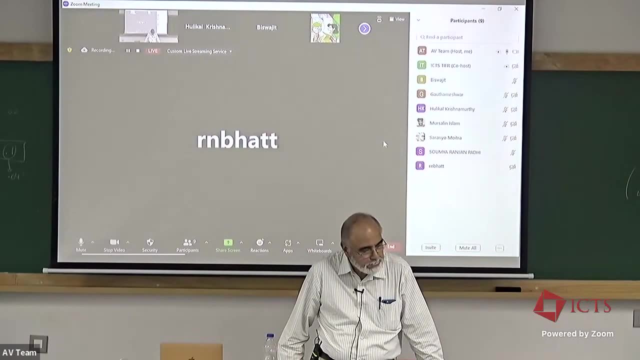 let me think about that. It will depend on if the my guess is that it'll actually go from K-f-l squared to K-f-l, because if the randomness is large, and that's the first physics that you're gonna see- and then when you go and you get to length scale, 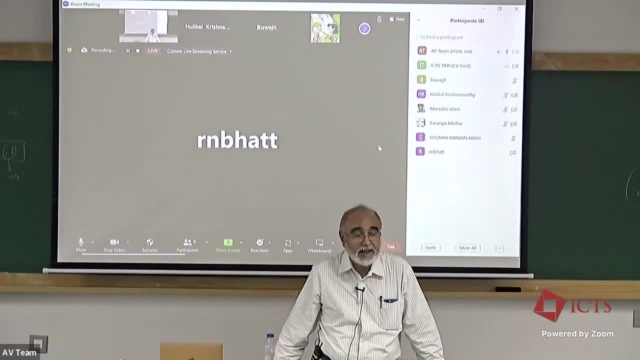 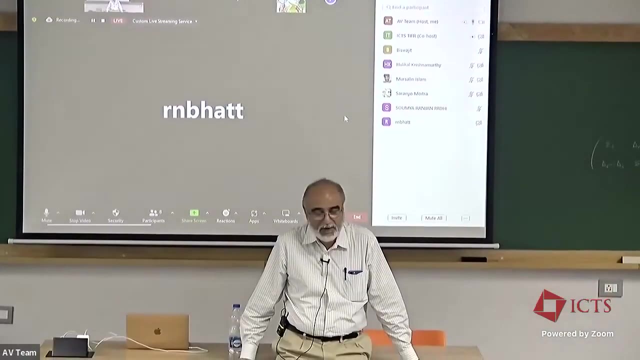 such that it starts persisting, receiving that little magnetic, mean magnetic field. then I think you will see the physics of quantum hall. So that's probably what it's going to do, but at the sizes that we are doing numerically. 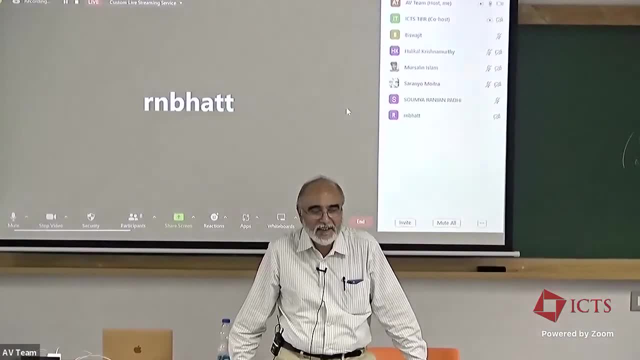 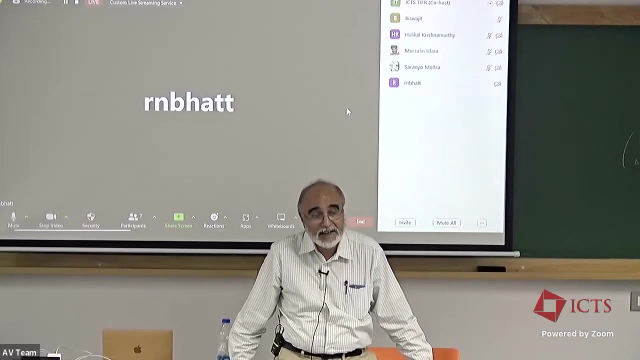 we are probably never going to see that little thing. You have to always figure out whether something is numerically feasible or not. but what you're saying is exactly right. You have to look at the crossover length scale by doing some approximations as to what kind of behavior you should get.